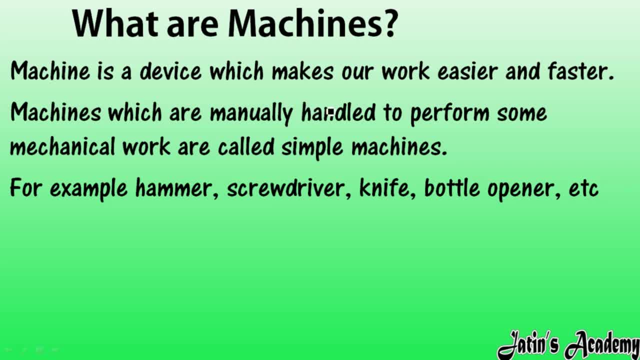 that is, what are machines? As the name suggests of our chapter, that is machine energy. So what do you mean by machine? Firstly, we should know the definition of machine. So whatsoever things we are using in our surrounding, for example, we are using hammer, we are using 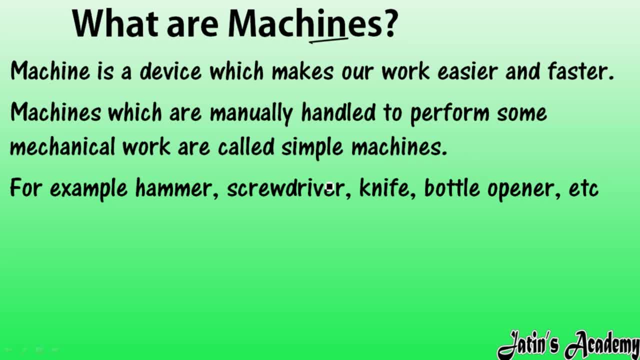 knife we are using bottle opener or whatsoever things we are using in our surrounding that makes our work easier and faster. For example, here, if I am having an apple, Here I am having apple. If I want to cut this apple, if I want to cut this apple by applying the force by my hand, Can I cut this apple? 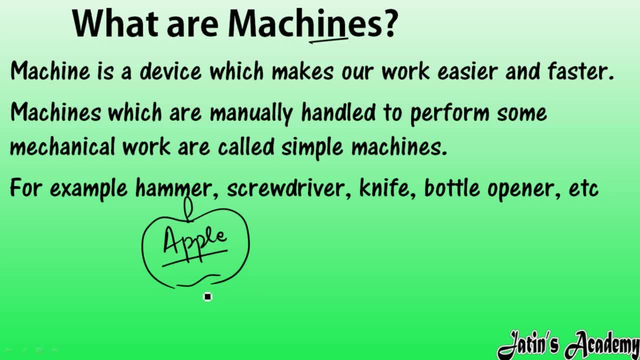 No, Obviously know how I can cut with my fingers or with my force from the hand. So if I am using here knife in order to cut an apple, so it is very easy to cut an apple within few seconds only by applying the force by knife. 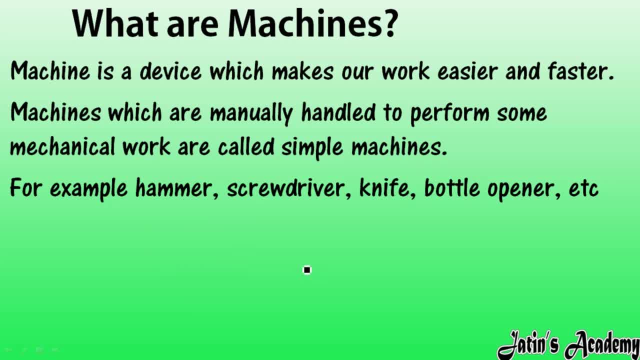 the instruments which are making our work easier and faster. that instrument or devices are known as machines- okay, and machines which are manually handled means whatsoever machine which we are using. we are applying some kind of force in order to move that machines or in order to take the work. 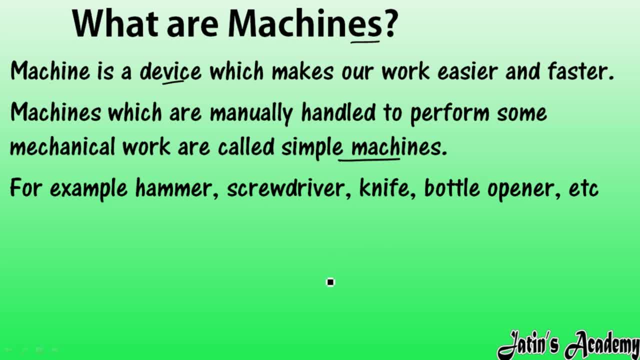 from that machines. that machines are known as simple machine or simply you can say the machines which are made up of only few moving parts, only one moving part. that is known as simple machine. for example of simple machine we are having like hammer in a case of hammer, not that much kind of 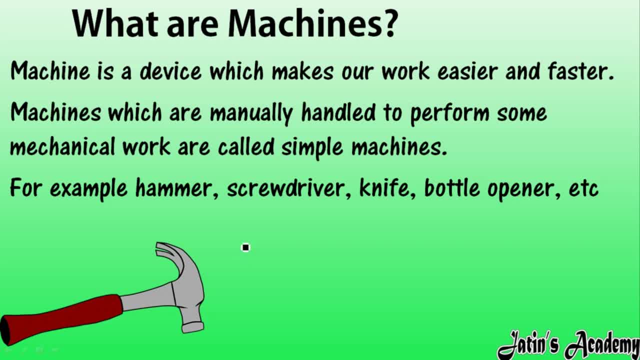 machines are connected and then a hammer is made. no, in a hammer simply one arrangement is there by which we can easily fix a nail into a wall or whatsoever. work we want we can do easily. okay, next we are having screwdriver, so screwdriver is also acting like a machine which makes our work. 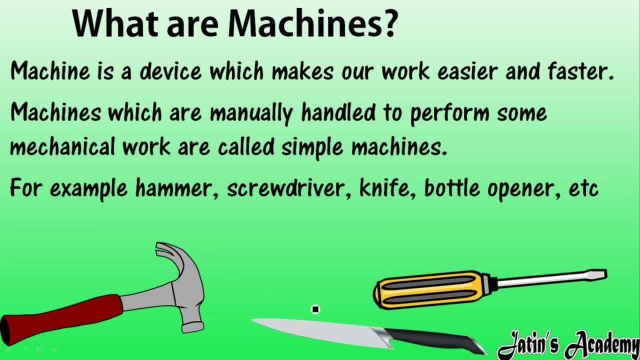 easier and faster. next, we are having knife, as i told already the example of knife. that knife is also acting like a machine, which makes our work easier and faster. next, we are having bottle opener. so in order to open the like bottle opener, in order to open the cap of the bottle- it is very difficult to use by. 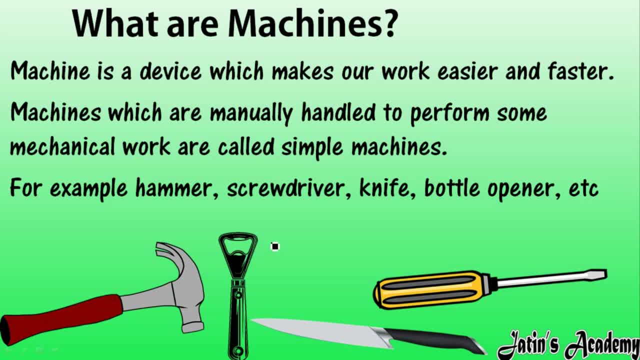 in order to open it by hands. so by simply using the bottle opener, within the fraction of second, we can easily open the bottle. okay, cap of the bottle. so the machines or the devices which are making our work easier and faster. next we are having knife, as i told already, the example of 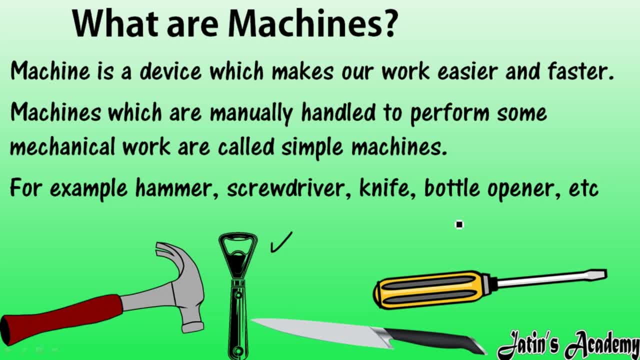 dagger made from iron, the knife make by hand is known as machin. next, the safety equipment- and we are saying that we are using these to make our work easier and faster- are known as machines, and the machines which are manually handled, which we are handling in order to work on it. 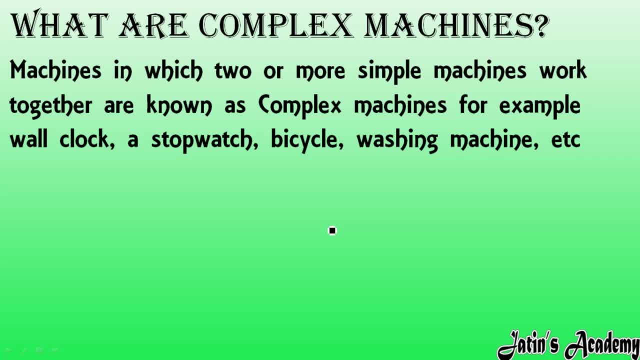 and the machine which contain only one or few moving parts. that is known as simple machines. okay, next we are having what are complex machine. in other hand, we are having complex machine also, but in our chapter or in our slay bus only. we are having just simple machines. but yes, we will looks in the 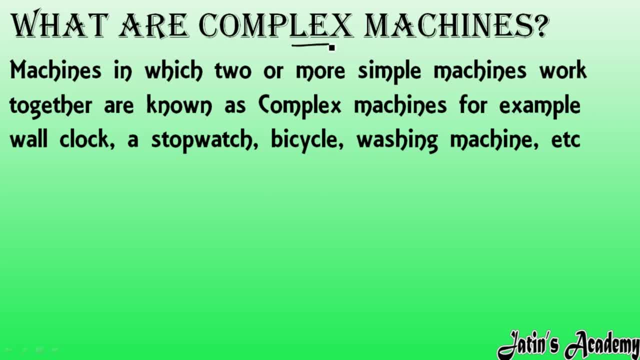 definition of complex machine. okay, so complex machine by name suggests complex machine. we have the final term, we will give step by step. a name suggests complex machines in which two or more simple machines work together. means, for example, we are having wall clock. means here, in wall clock two or more simple machines are combined. 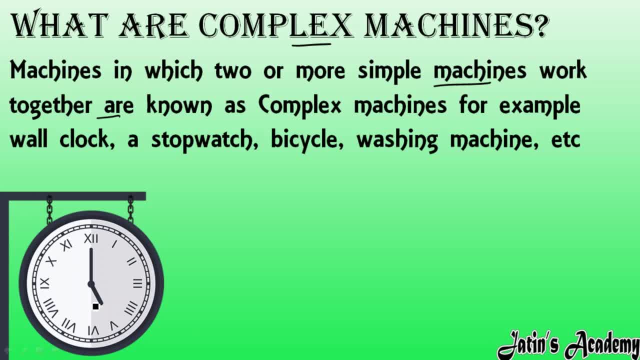 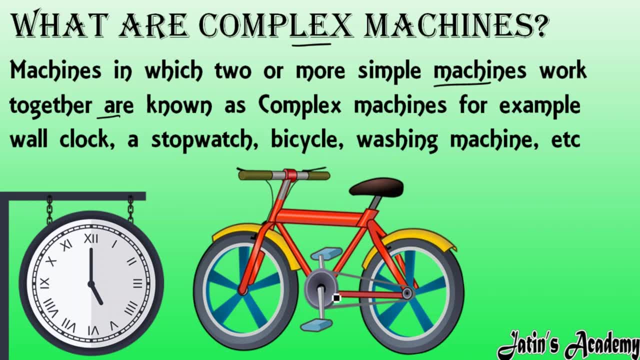 together in order to move this wall clock, so this wall clock is regarded as complex machine. in a similar manner, we are having bicycle here. in bicycle also, we are having more than one simple machine, so this bicycle is also regarded as complex machine. in a similar manner, we are having 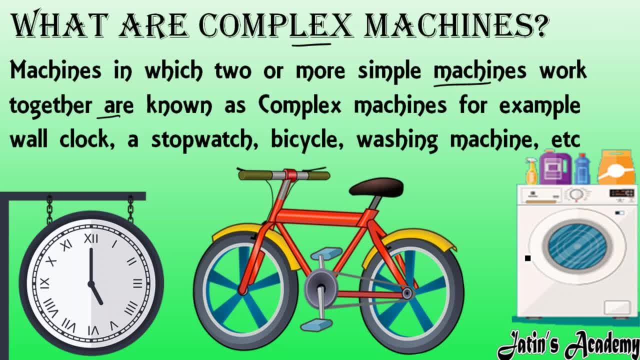 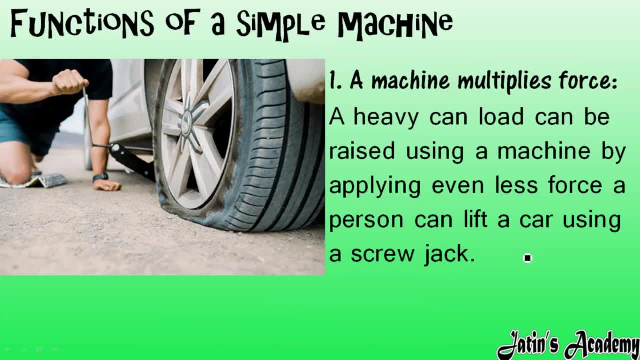 washing machine. many are there which are regarded as complex machine. okay, in a complex machine, two or more simple machines are combined together in an one object. fine, next we are having some functions of a simple machine in this chapter, as we are going to study only about the simple machine. 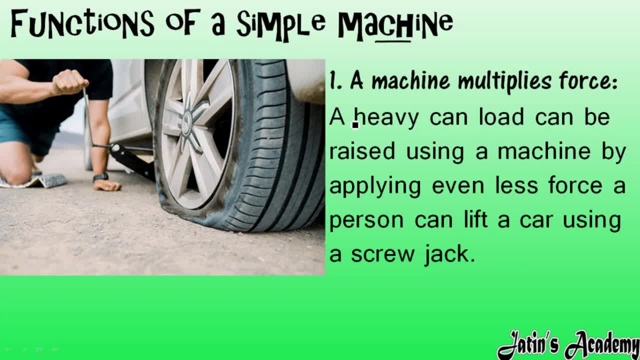 so firstly we will discuss about the functions of simple machine, that how simple machine are helping in our daily life. so first we are having a machine multiplies force. for example, when you are going somewhere on a road, you are having double machine, slow machine, which is a machine that is doing. 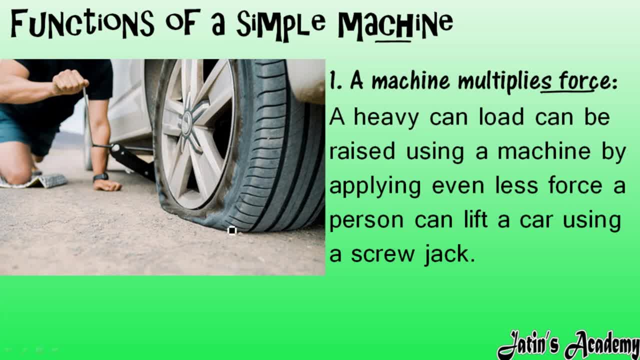 road trip and all in between the road trip, the tire of the car is punctured and you want to change the tire. so how you will change the tire? firstly, you will pick the car by your hand, by your muscular force. then you can change the tire. like this you are doing. no, obviously no, we are. 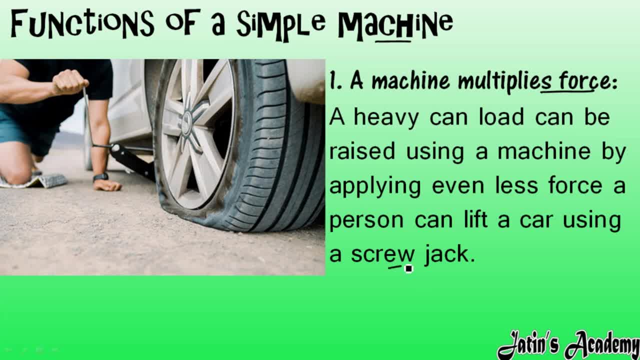 using here one kind of machine known as screw jack. here one kind of machine is there which this person is using. this is a screw jack, which is order to lift the car up, and by using the screw jack, firstly we will lift the car up, afterward we will change the tire. so what is happening here? 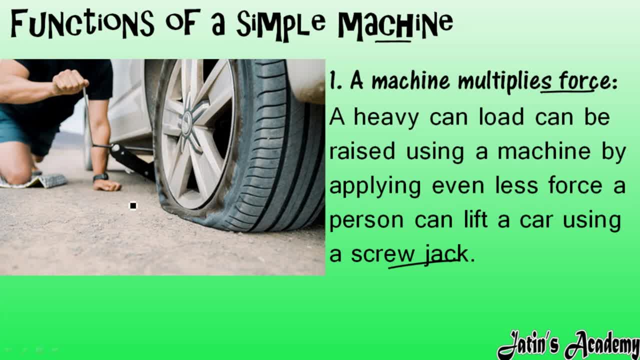 actually, here we are using a simple machine, this screw jack we are using. it is a simple machine. means here we are applying very less force in order to move this machine, but this machine is lifting very much. higher force means it multiplies our force. for example, if here i am applying 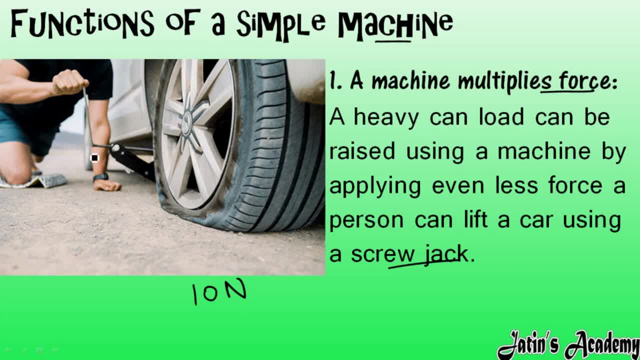 10 newton force in order to move this screw jack. this screw jack is lifting up, for example, 500 newton object or 500 newton force. it is applying on and car. okay means it is multiplying our force, and this is a function of simple machine. this is a beauty of simple machine, how it is going to help us okay. 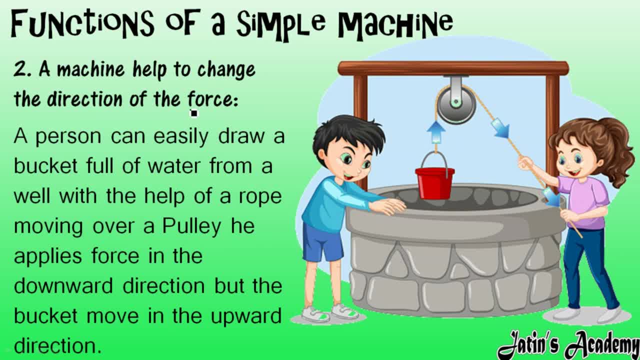 next, we are having a machine help to change the direction of force. for example, if you are standing in front of a well and you want to take the bucket up from the well, okay, what you are doing. we are not just making our hand down and we are picking up the bucket. no, here we are using one kind of 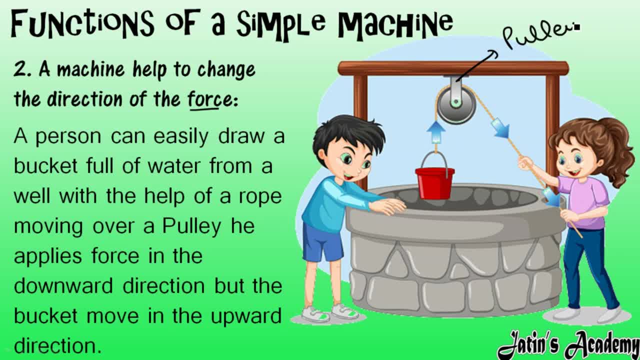 simple machine called pulley. one by one, we will discuss all this kind of simple machine, don't worry. but here, just see the example of pulley here, in this case, we are using a pulley in order to lift the bucket up from the. well, what we are doing here, see carefully. actually, if you want to apply your force on the 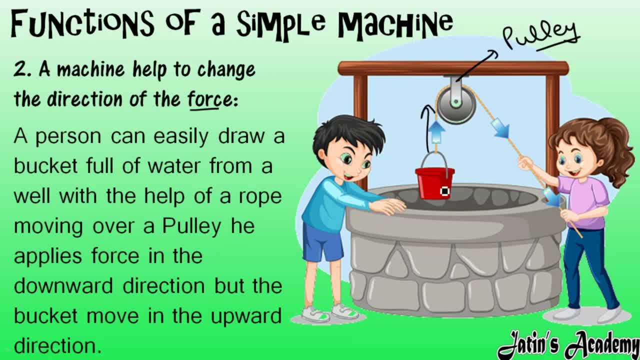 handle of bucket and you will take it up. it is very difficult to do like this, okay, so what we are using? we are using here pulley in a pulley. one rope is attached. actually, we are pulling. we are just pulling the rope toward herself in a downward direction by pulling it toward ourselves. bucket. 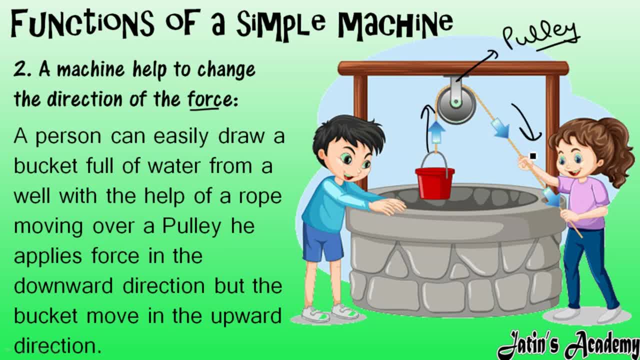 is coming in an upward direction means by applying force in a downward direction, bucket is coming in a upward direction. means with the help of machine, we are changing the direction of force. we are applying in a downward direction force, but here bucket is coming in an upward direction. so it is a very simple to change the direction of force. 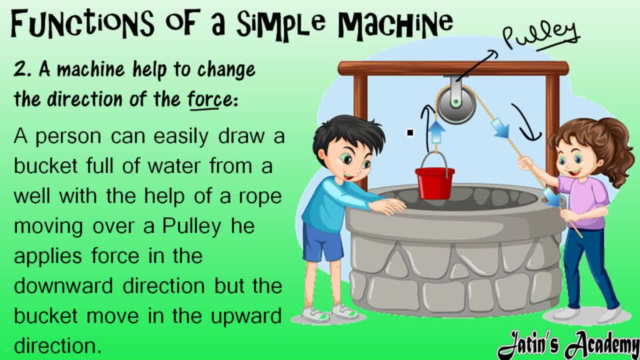 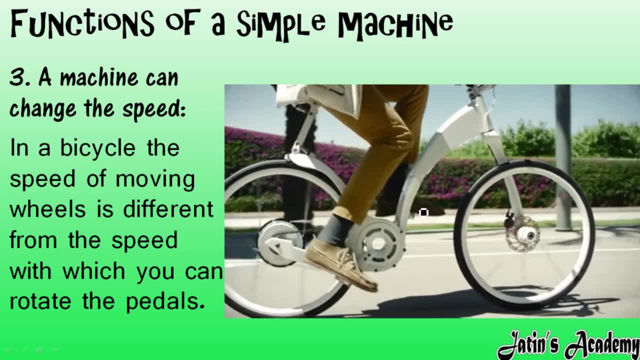 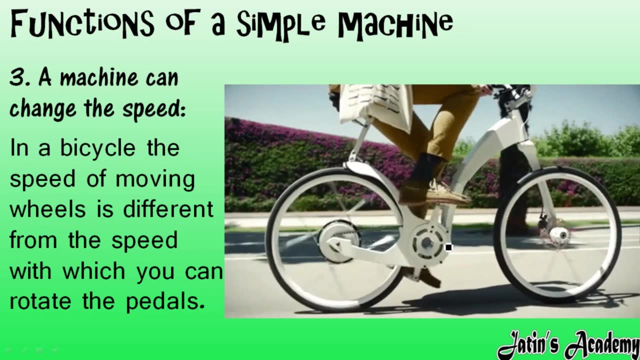 with the help of machine. next, we are having a machine change. the speed means in a bicycle, the speed of the moving wheel is different from the speed with which we can rotate the paddles means the paddles. we are applying very little force and with the help of little force these paddles are moving. but the speed of these? 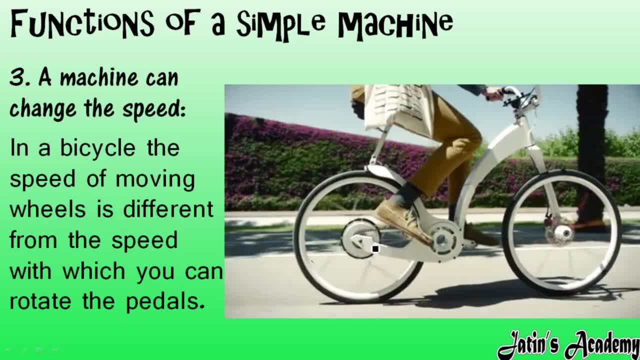 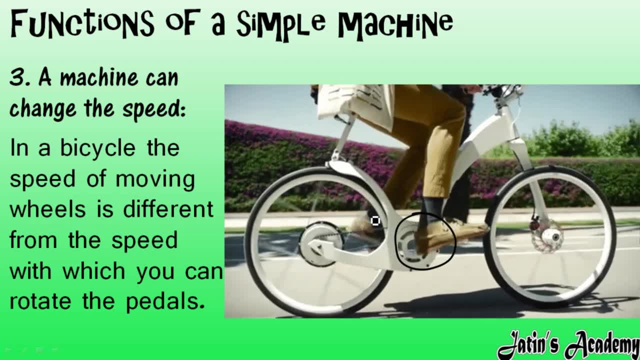 wheels. these big wheels are very much less as compared to the force which we are applying on the paddles. means these paddles now here are acting like a simple machine which is making our work easier and faster, and we can change the speed with the help of machine. 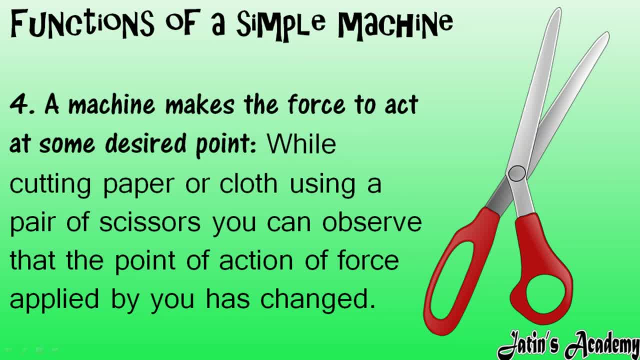 next function of simple machine we are having. a machine makes the force to act at some desired point means, for example, while cutting a paper or while cutting a cloth, we are using a pair of scissor. okay, so in order to cut a cloth, firstly we are applying force on the hands of the scissor. 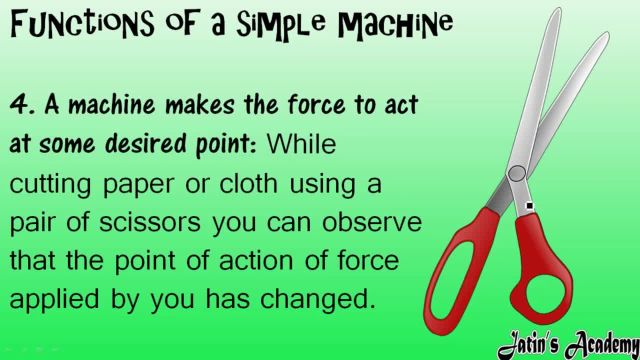 okay, we are applying force on the hands of scissor, but we are not applying force on the hands of the scissor. but what the scissor is doing? scissor is applying force on a paper by this long arms means by applying the force or by the machine. with the help of machine you can make the force to act at some. 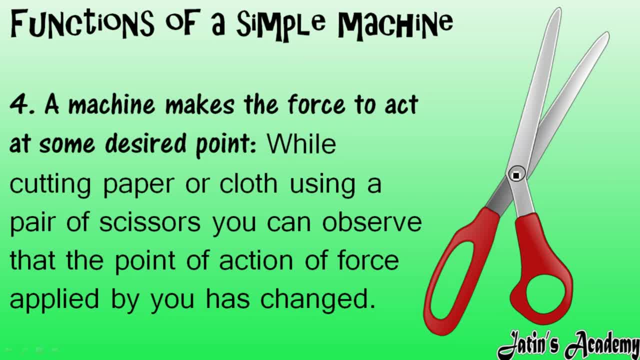 desired point. okay, we can simply make. the force means we are applying force here on these hands. but here cutting of paper is going to done with the help of these long arms means with the help of simple machine. we are just changing the desired point, okay, next we are. 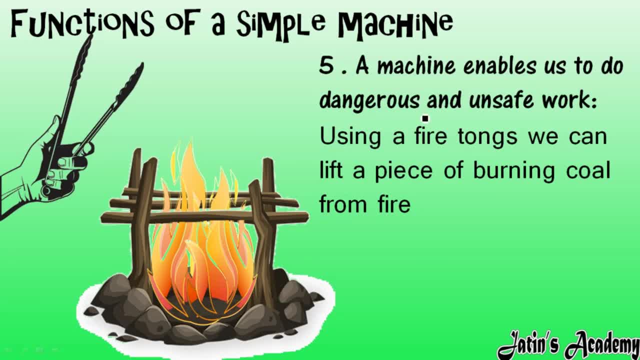 having fifth function of simple machine. a machine enable us to do dangerous work means in order. for example, we want to burn the substance in this fire, okay, by just using your fingers and putting into this fire, it is very like difficult or unsafe work. in order to do this, okay, but in order to do 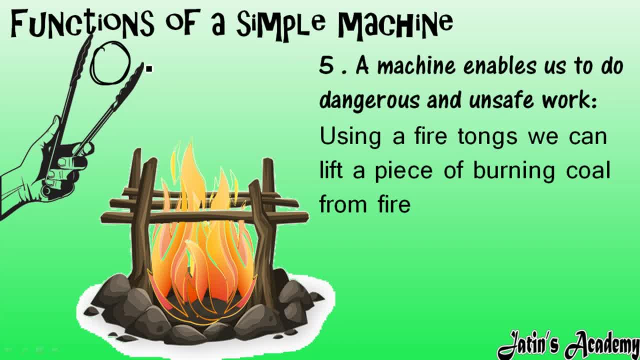 this unsafe or dangerous work. we are using this kind of simple machine known as fire tongs. this is a fire tongs which help us or which enable us to burn this material or burn this substance in a fire, so this simple machine is making our work easier. this is a simple machine, fine. next we are. 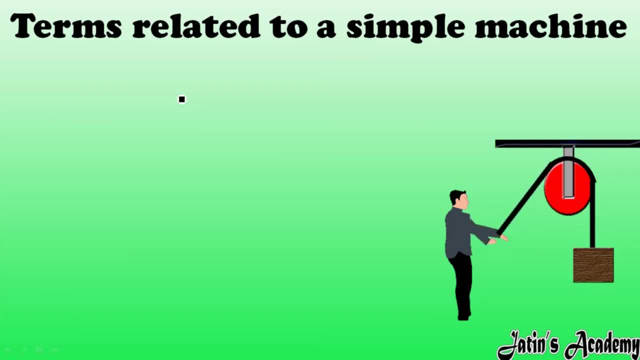 having terms related to a simple machine. so, in order to learn the simple machine, firstly, some basic terms are there that we should know first, and how to use that term. see carefully what are that terms? first, we are having effort. so what do you mean by effort in order to use any machine? 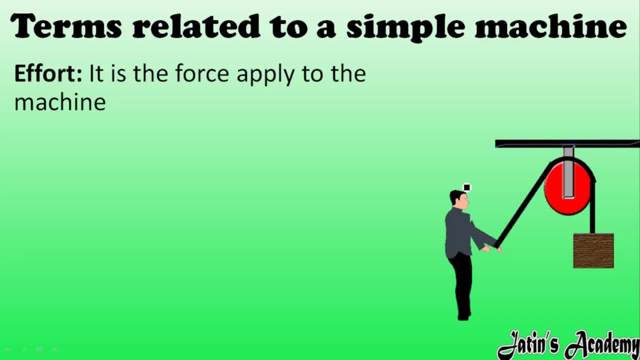 we are using a fire tongs which help us or which enable us to burn this material or burn this. firstly, we have to apply some force on that machine so that machine can do work okay, by simply just sitting on one like a place, the machine cannot do its work. fine, we have to go on. 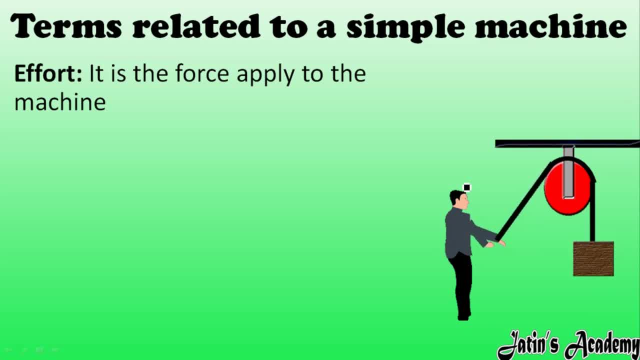 machine. we have to work, we have to apply some force on that machine. so this force applied by us on the machine is known as effort, fine, and next term we are having load. load means it is a force exerted by the machine on an object. means now, after applying overwork, after applying overforce, what this machine is applying force on 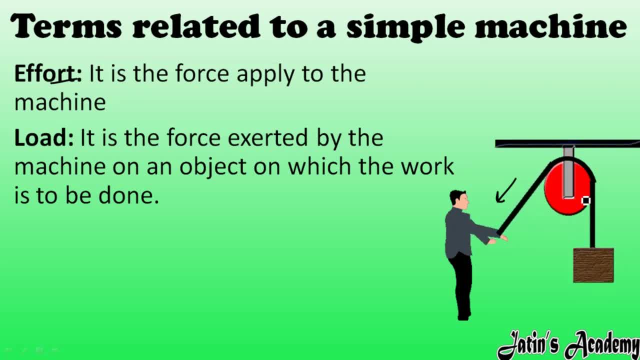 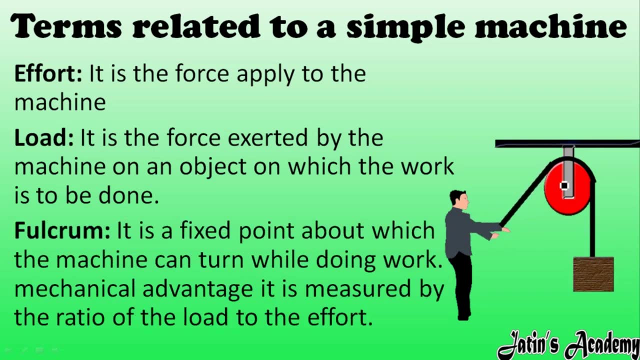 an object, all of this load in order to lift it up or whatever it want to do. the force exerted by the machine on an object is known as load. come related to simple machine is fulcrum. so what do you mean by fulcrum? it is the fixed point. it is the fixed point about which this simple machine is going to. 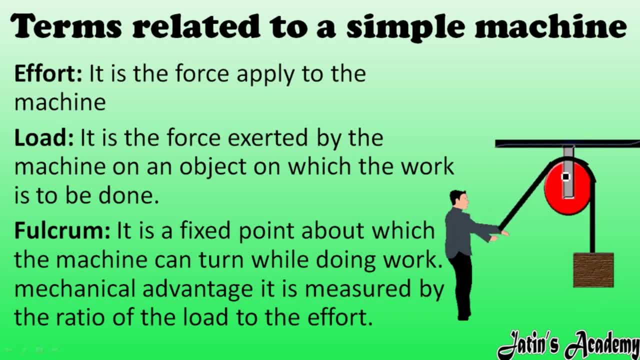 rotate while doing work. this fixed point is known as fulcrum. okay, next point: we are having mechanical advantage. what do you mean by mechanical advantage? actually, mechanical advantage is a ratio of load over effort means load over effort means what load? we have learned now. only load is a force. 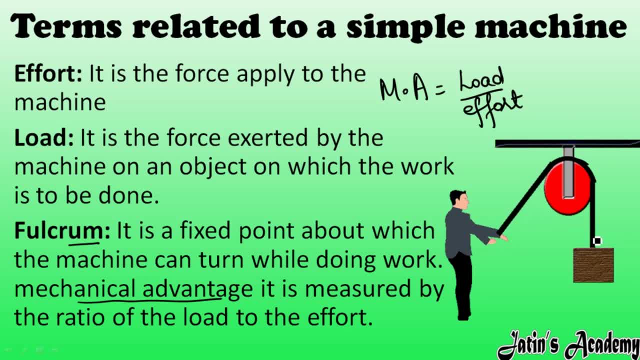 exerted by machine on an object. so what? what the force is acting by machine on an object over what the force we are applying on the machine in order to do that work. this is a ratio of these two terms. so these two terms is a ratio called mechanical advantage. so here we are having 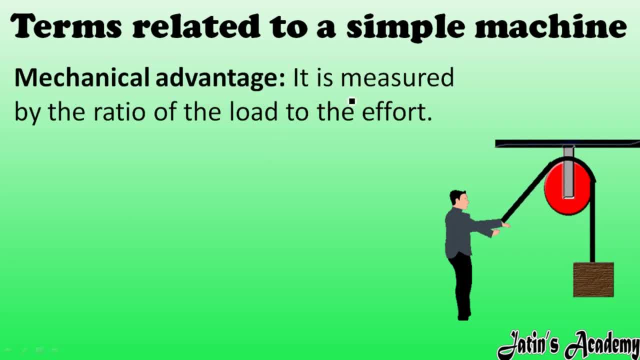 definition of mechanical advantage. so mechanical advantage is measured by the ratio of load over effort. mechanical advantage is equals to load over effort. next we are having SI units. as we know, load is what? load is a force applied by machine on an object. so load over effort is a force applied by machine on an object. 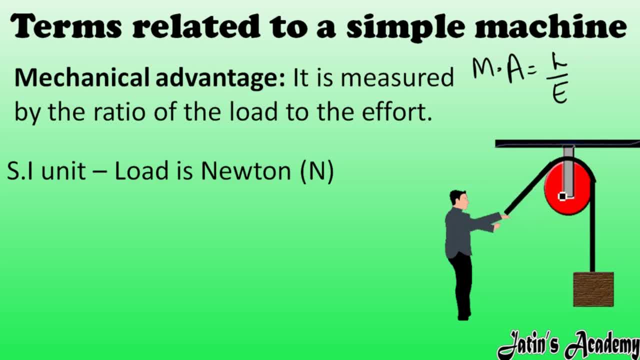 so, in short, load is a force. and what is the SI unit of force? SI unit of force is Newton. in a same way, SI unit of load is also Newton, because load is also a force kind of force. next, we are having SI unit of effort. as we know what is an effort, effort means whatsoever force we are applying on. 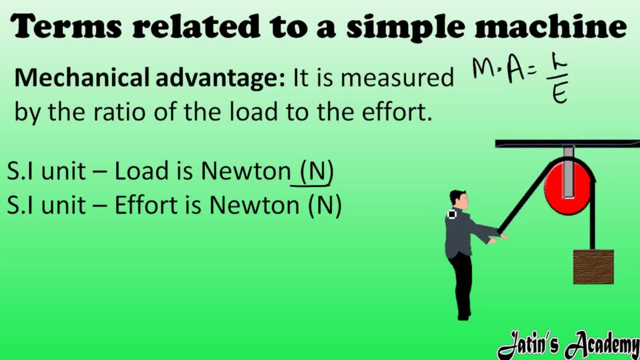 the machine in order to work it. that is known as effort. okay, so effort is also a force, applied force. SI unit is Newton, means effort. SI unit is also Newton if you talk about the mechanical advantage, SI unit of mechanical advantage. mechanical advantage is load over effort. what is the SI unit? 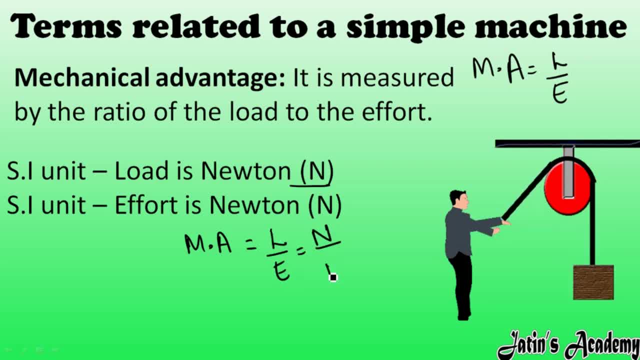 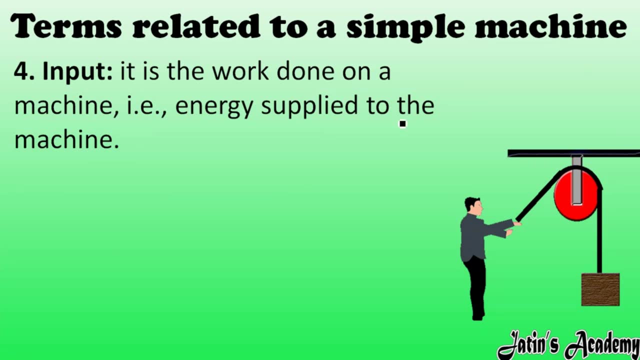 of load, Newton. what is the SI unit of effort, Newton? so Newton, Newton will cancel each other. means mechanical advantage is having no units, okay. next important term related to simple machine is input. so what do you mean by input? see carefully: input is a work done on machine in order to move this machine. what so ever work we are doing on machine that is known as 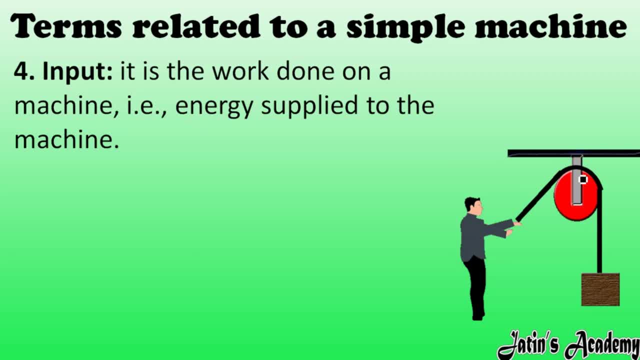 input, or you can also say like this: energy supplied to the machine, and. but not get confused in effort and input actually in effort, I told that whatsoever force we are applying on the machine, force means effort means force we are applying force. force means push or pull to an object. push, 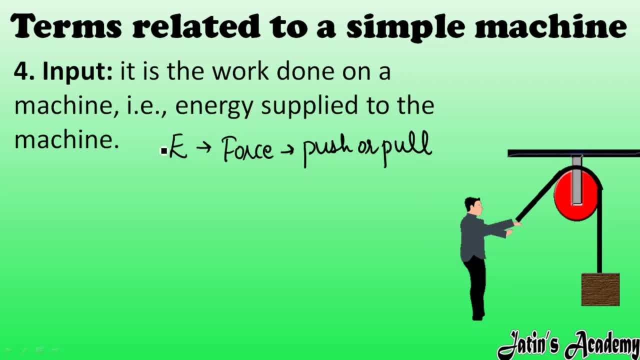 or pull to any object is known as force. but if you move this force on the machine it will not work. But here, in case of input, I am saying work done on machine. work done means what work done means. force multiply distance means how much force we are applying on machine and how much distance. 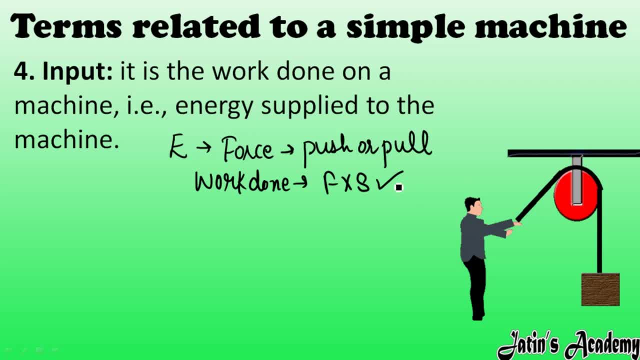 it is moving. Okay. so work done means force: multiply distance and force. simple force means push or pull to an object. Next important term related to simple machine. we are having output. So what do you mean by output? output is a useful work done by machine on an object. means how much? 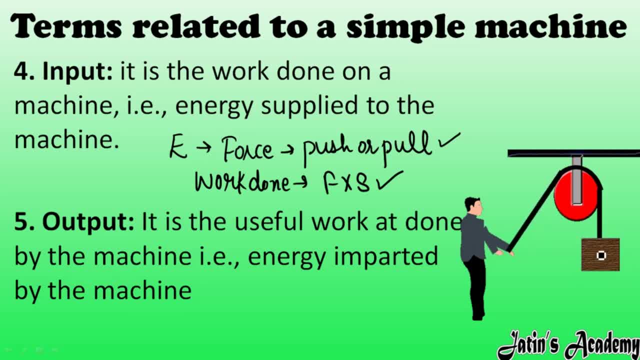 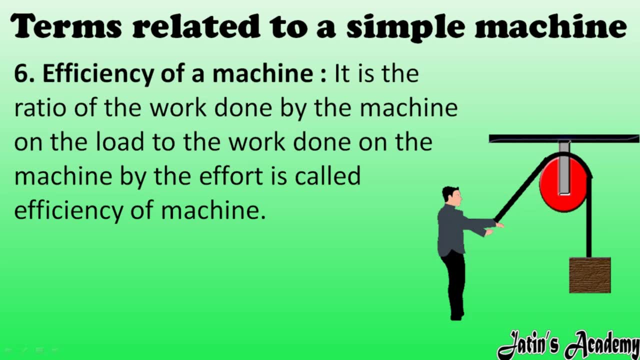 work. this machine is showing on an object in order to do the work that is known as output, and second definition. you can learn like this also: energy imparted by the machine on the object that is known as output. Next important term related to a simple machine we are having 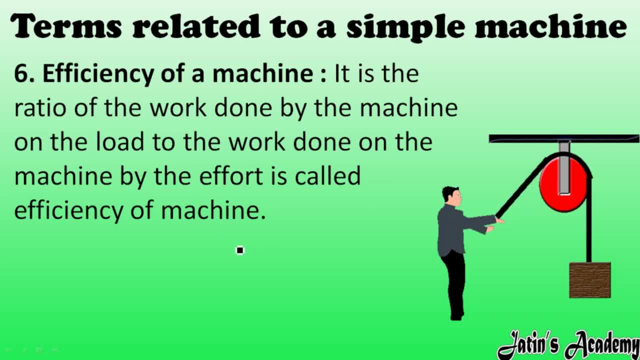 efficiency of a machine. So what do you mean by efficiency of a machine? efficiency of machine is defined as the ratio of work done by the machine on the load, Which is also known as output. So it is a ratio of output over work done by us on the machine, or you? 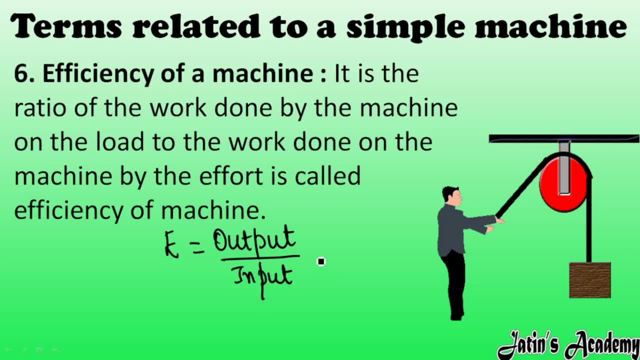 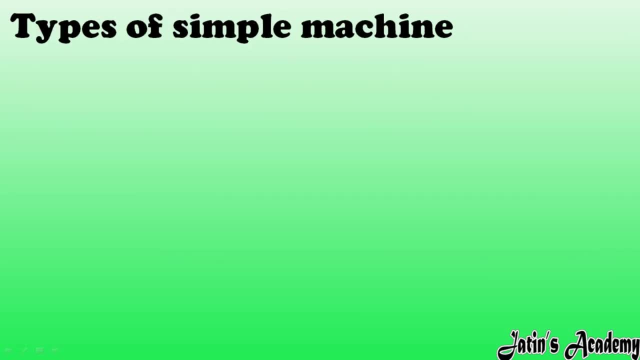 can say: input: Okay. so efficiency is having the formula output over input if you want to calculate the efficiency percentage. So efficiency percentage formula is output over input, multiply 100. this you can simply learn, also find this is known as efficiency of a machine. Next we are going to 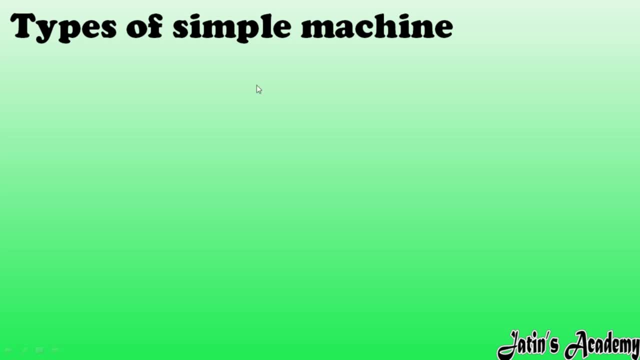 study about the types of simple machine. So here in this chapter we are going to study about the 6 types of simple machine. First we are having lever. second, we are having inclined plane. this is a form of inclined plane. Then we are going to study about wedge. 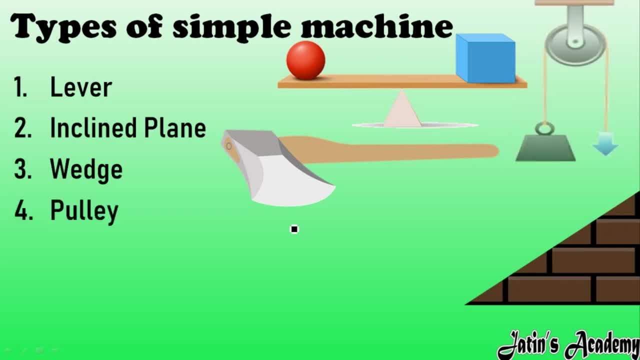 This is the wedge formation of a simple machine. Then we are going to study about pulley- this is kind of pulley. then we are having Screw- this is a screw. then at last we are going to study about wheel and axle. So in this chapter, in detail, we are going to study about all the 6 types of simple 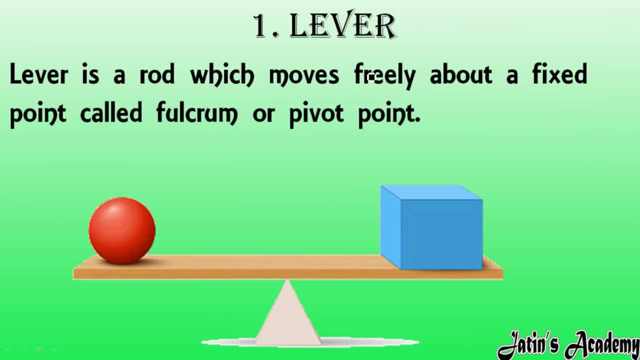 simple machine. so let us start with the first simple machine, that is, lever. so what do you mean by lever? actually, in this lever, lever is a rod. here this kind of rod is there which moves freely. this rod is going to move freely about a fixed point and this fixed point about which rod is. 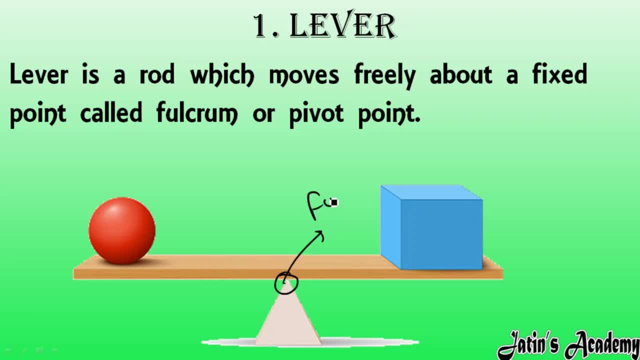 going to move freely is known as fulcrum. this is known as fulcrum, or you can say pivot point. pivot point means the fixed point about which this rod is going to move. fine, and at the one end, we are going to apply some effort here, at the one end, we are going to apply some effort, and here we 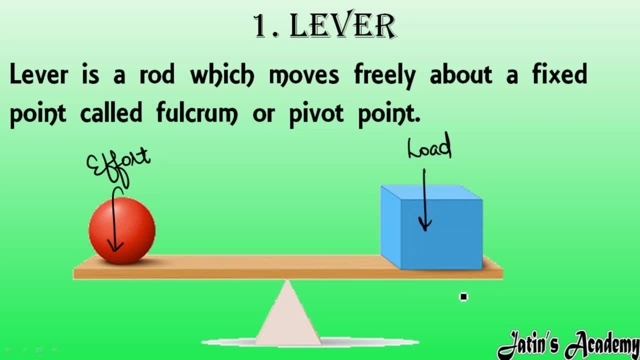 are going to use the load in order to raise any load. we are using here, some load, here we are applying some kind of effort and here in center we are having a fulcrum or pivot point. fine, then afterwards we are having the weight to be moved. 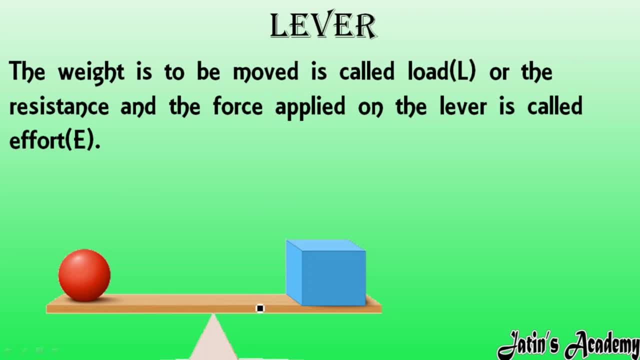 means, for example, with this lever whatsoever- wait, you want to move. that weight that you want to move is called load. this is a load, ok, Or the resistance load. other name is resistance, and the force applied on the lever means, as i already told, simple machines. i am not going to work by the yourself. 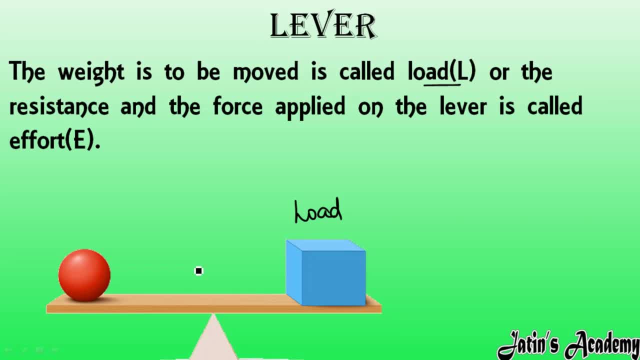 ok, we have to apply some kind of force on it and in order to move this lever also, we have to apply some kind of force on the lever and the force is strong and i have some kind of methods. force applied on liver is known as effort means. on one end, we are going to apply some kind of. 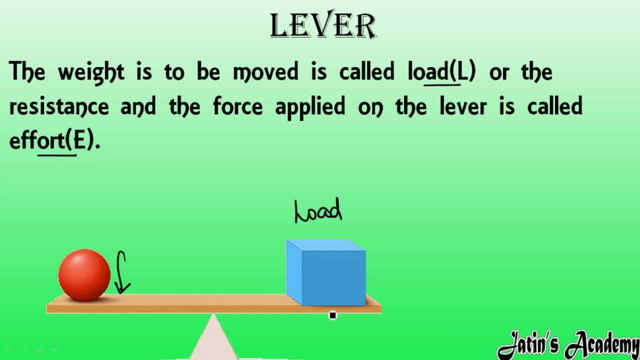 force and, on the other hand, on the other end, simple machine is going to do some work. that is known as, this is known as simple machines work, or this is a function of liver, okay, next we are having the distance between the fulcrum from the point at which effort is applied. this distance, 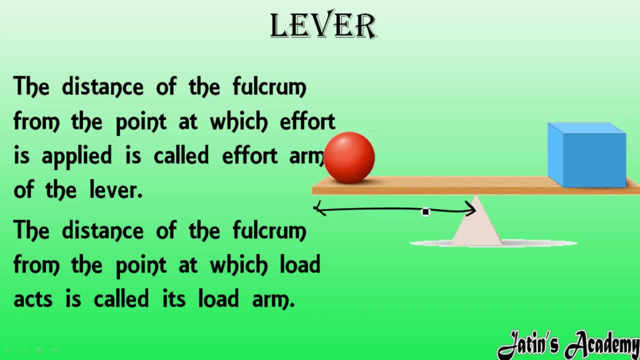 between the effort applied and the fulcrum- this distance is known as effort arm- and the distance between the fulcrum and the load. this distance is known as load arm. find the distance between the fulcrum and the effort arm- and the effort is known as effort arm- and the distance between the 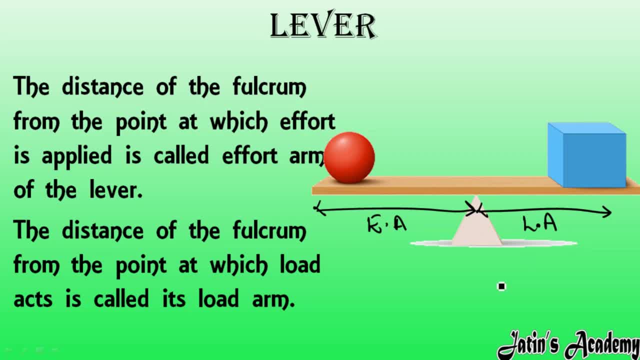 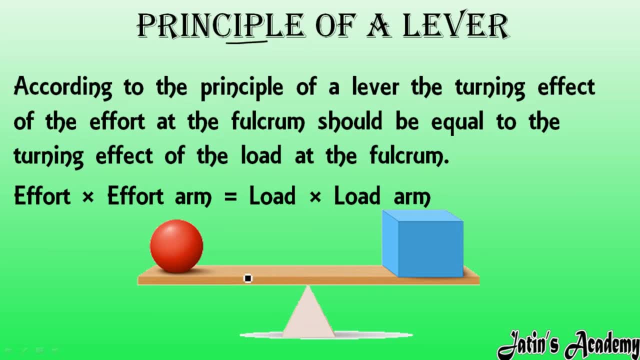 fulcrum and load. is load arm definitions clear? no, next, we are having principle of liver. on which principle, on which function liver is going to work? actually, principle of liver is a turning effect of force. so what do you mean by turning effect of force? actually, turning effect of force. you will study this concept in class 8. properly, you will study. 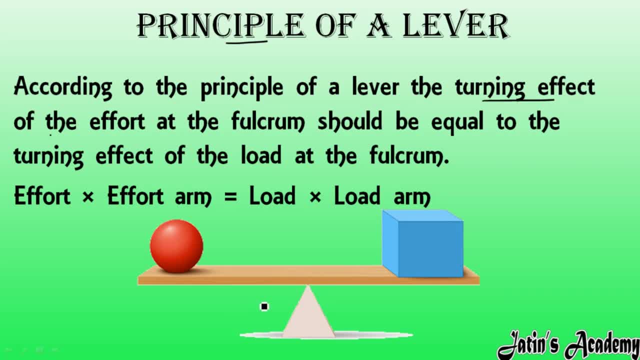 in that class, but, yes, in this class. i will tell you something about turning effect of force. turning effect of force means whenever we are applying force to any object, for example in this, i am going to apply the force here on this effort point. okay, so whatsoever force we are applying on? 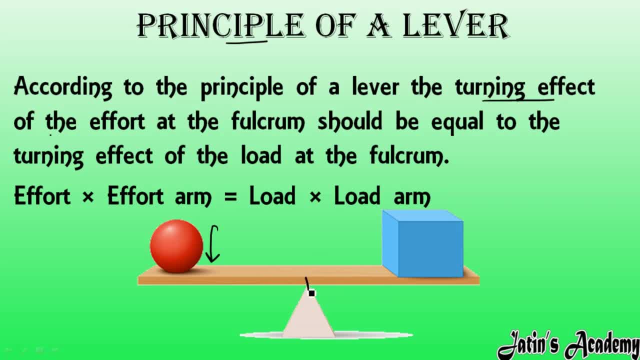 any object on that object which is pivoted or which is fixed at one point, that object start rotating about a fixed point. if i take the example of door, in a case of door, when we are going to apply the force on a handle of the door means when we are applying the force on the handle of door. 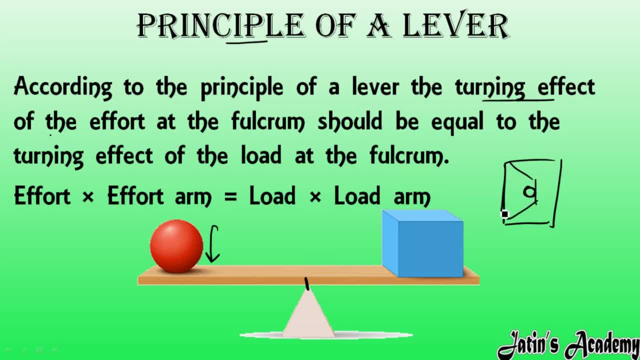 door start turning or start rotating about the fixed point, about this fixed point. so this turning, if this movement of force about the fixed point is known as turning effect of force, okay, and this states that turning effect of force at fulcrum should be turning effect of force at. 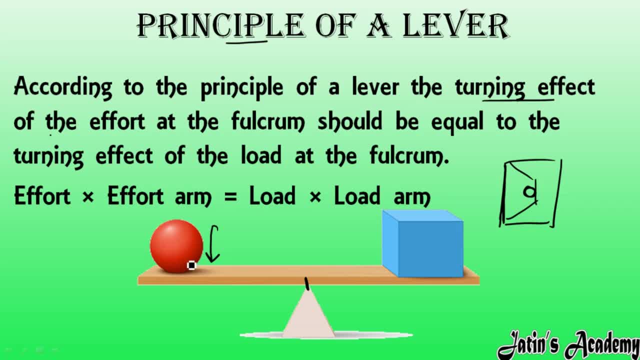 load means whatsoever. the turning effect of force is there at effort point. same kind of turning effect will be there at load point also at the load arm also. okay. so this principle we are having effort into effort arm means this effort multiply effort arm is equals to load into load arms. if 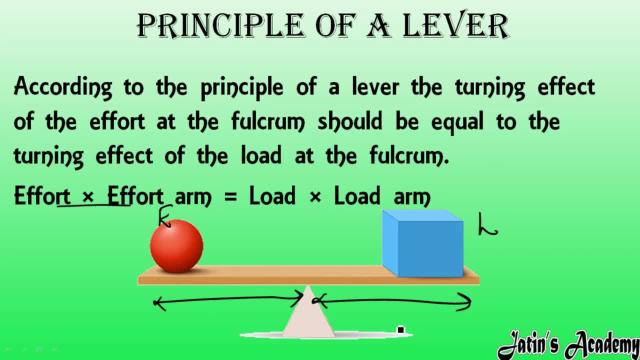 we are not understanding that much about the turning effect of force. no problem, just learn this formula. actually, this formula is important for the principle of a lever that is effort into effort. arm is equals to load into load arm. this kind of formula we are going to use in order to 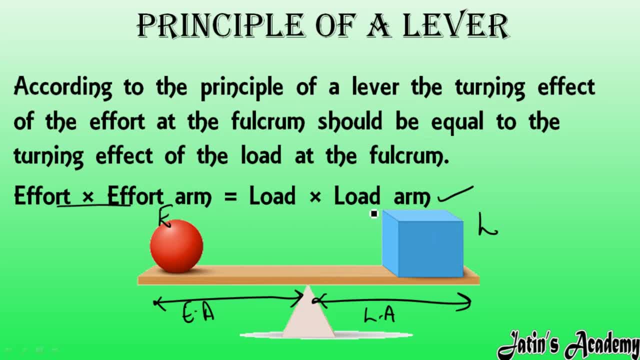 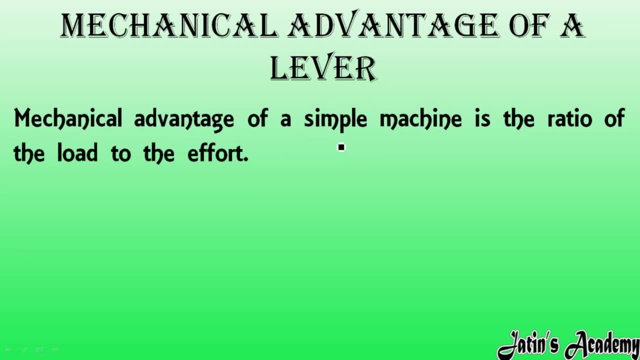 solve the numericals also. so you have to remember this formula, fine. next, we are having mechanical advantage of a lever. so, as we know, mechanical advantage is actually a ratio of load over effort. in order to calculate the mechanical advantage, actually, mechanical advantage means how much advantage we are getting from the simple machine. okay, how much simple machine is helping us? 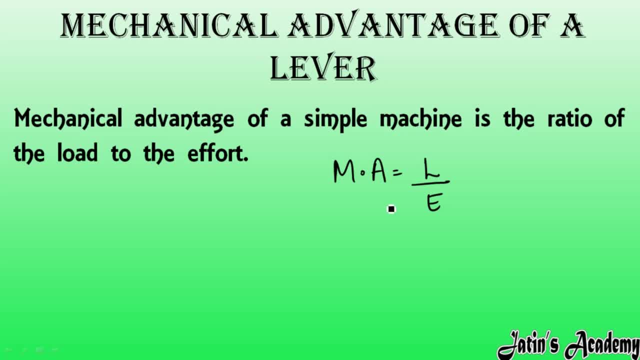 that is a mechanical advantage and in order to calculate the mechanical advantage, we are using the simple formula that is, load over effort means what force that simple machine is applying on the load or on the links of object and what force we are applying on the simple machine. it is a simple. 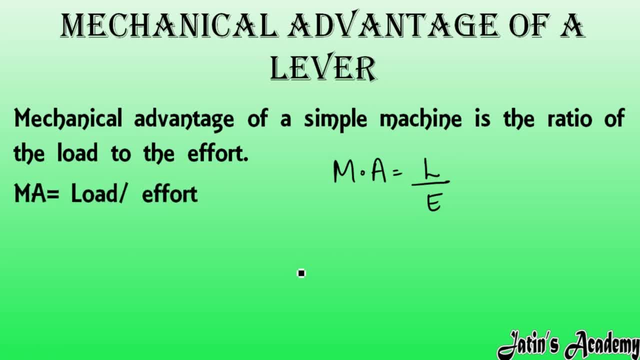 machine. it is known as mechanical advantage. so next we are having this formula: mechanical advantage is equals to load over effort, so mechanical advantage of a lever. so in order to calculate the mechanical advantage of lever, we are having formula like this: mechanical advantage is equals to effort arm, effort arm over load arm. so how this formula came, see carefully. 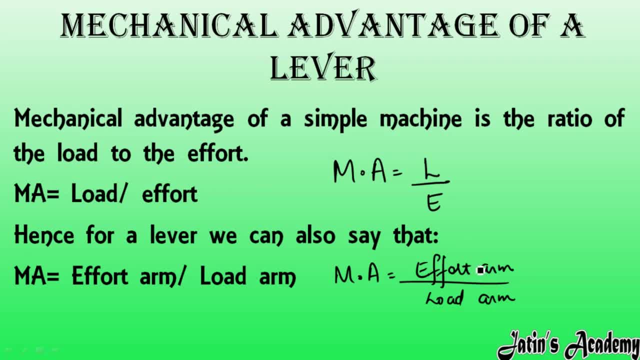 actually in the before slide only, we have discussed about principle of the lever. so what is the principle of a lever? that is, effort into effort arm is equals to load into load arm. we have studied this only now. I will write the properly here: effort into effort arm. effort into 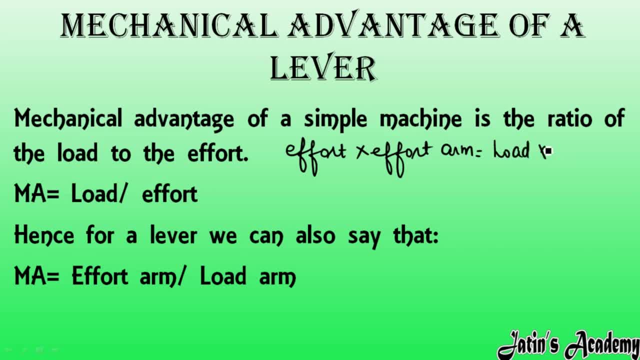 effort arm is equals to load into load arm. this only we have studied in the principle of lever, and here we want to calculate the mechanical advantage, which is nothing but a load upon effort means this effort is in multiply that. can I take this F word to that side? it will go in a divide sign. 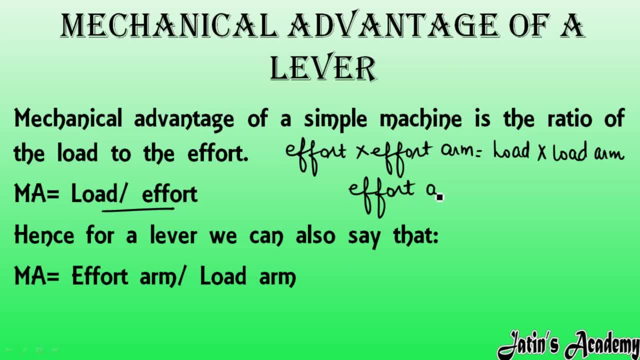 so here, effort arm is same in this formula. a for time is same, here is equal to same, load is same, Sephiroth or πάล is same, okay, only just effort is in multiply. that said, it will go in Divide. fine, so here you can see: this load arm is in Multiplied, that's it. it will go in Divide, so it will be effort. 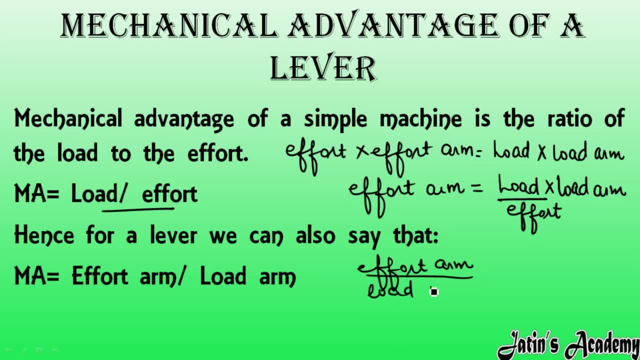 over load arm is equals to load over effort. fine, and, as we know, load over effort is what load over effort means: mechanical advantage. so mechanical advantage of lever is equals to effort arm over load arm. from this derivation this formula came. if you understood this derivation, that is very. 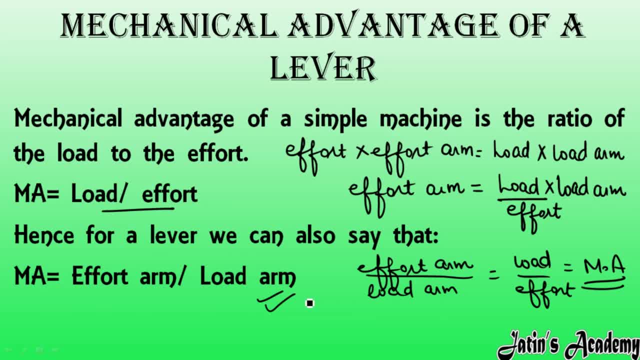 good, but if you not understood, no problem, just learn this formula: mechanical advantage is equals to effort arm over load arm, which we are going to use in the numericals also. fine mechanical advantage, simple, is load over effort. but in a case of lever we are having effort arm over load arm. 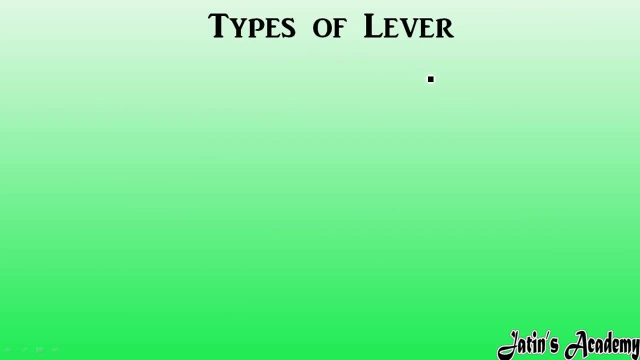 next we are having types of lever. so in this class we are going to study about the three kinds of lever. first is first class lever. in a first class lever, here same in all class lever, same arrangement will be, there only the difference between the arrangement of the load, effort and fulcrum. so 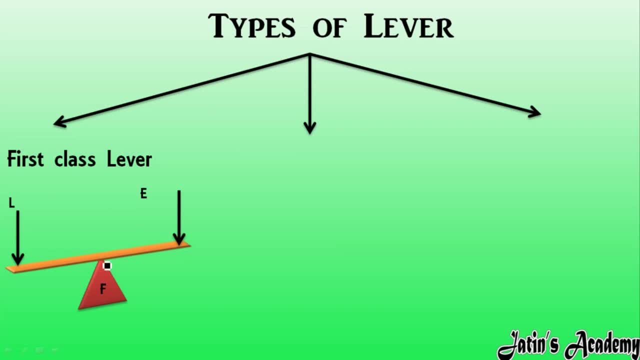 in a first class lever we are having a rigid rod which is going to sport at some fixed point- fine- and this fixed point is known as fulcrum. just learn from this. actually, we are having three kinds of lever. i will tell you one by one. first we are having first class lever, then we are having 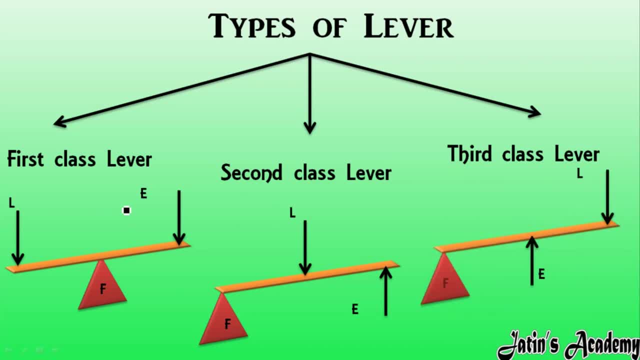 second class lever, then we are having third class lever. see carefully how to learn these diagrams. you have to learn like this: flea, f, l, e flea. flea means in first class lever, you have to take fulcrum in center. f means fulcrum in second class lever, you have to take load in center. 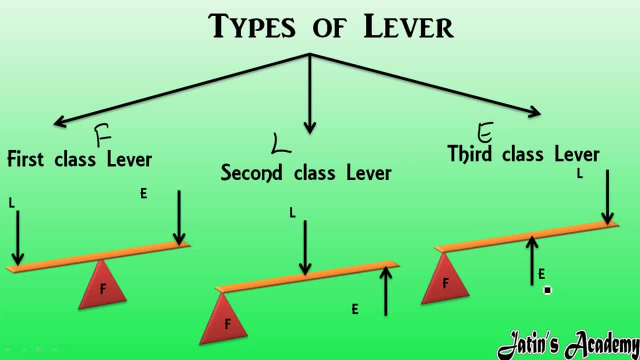 and in third class lever you have to take effort in center. this rigid rod will be same in all three, all three classes of liver, but only the arrangement of fulcrum, load and effort is there, fine. so flea formula: you have to learn flea first in fulcrum is there. in second class, load is there. and 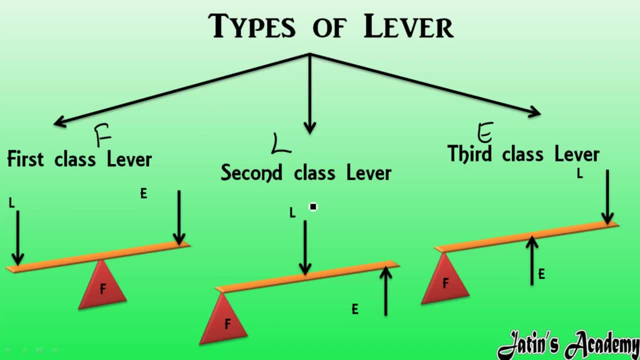 third class effort is there in the center. now what about the other two ends? so in the other two ends, first in first class liver, it is simple means that one end effort is there and one end load is there. or you can rearrange also here effort or here load. okay means fulcrum is in. 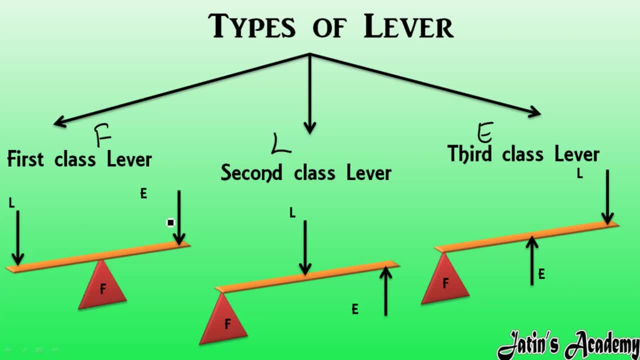 center and effort and load are on other ends. that is simple. fine, in a second class lever and third class lever you have to remember that this fulcrum you have to take on left hand side only, fulcrum you will take in left hand side only, and in second class load is in center, then obviously effort will. 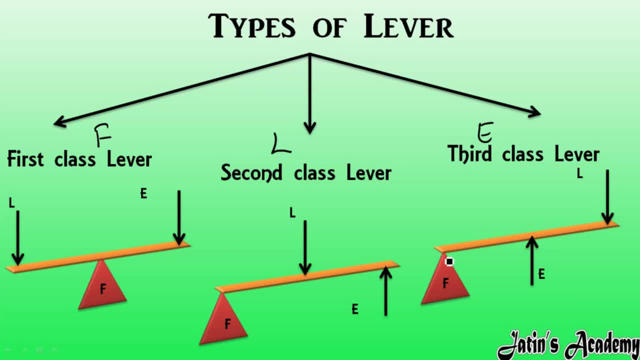 similarly in third class, lever effort is in center fulcrum. i told you have to take in at left side only so what is left. you are left with load. so obviously left is at the load is at the right side. so like this you can learn the arrangement of the first, second and third. 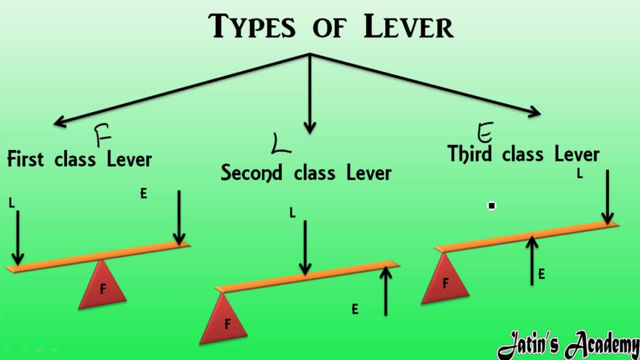 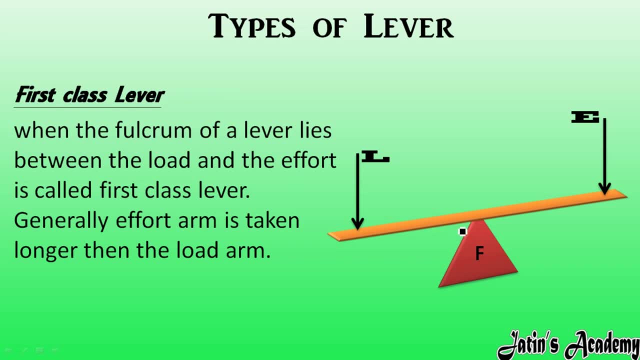 class lever and one by one, we are going to discuss why these arrangements are like this. fine. so first we are having first class liver. first class lever means when the fulcrum of a lever lies between load and effort. okay, when the fulcrum is in between load and effort, that kind of lever is known as. 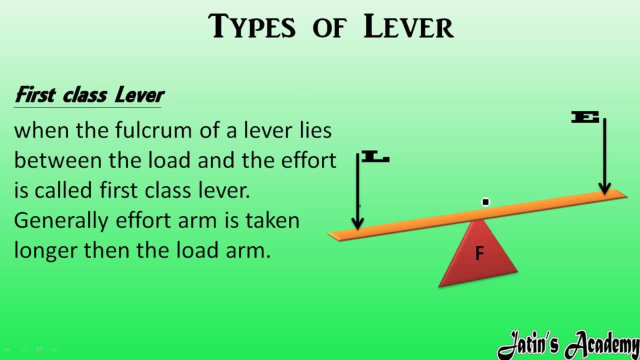 first class lever. so actually in this case- see carefully- this fulcrum is here and this is effort arm- means distance between effort and fulcrum is effort arm and distance between fulcrum and load is load arm. so in a first class lever, in all cases effort arm is more. this effort arm is more as 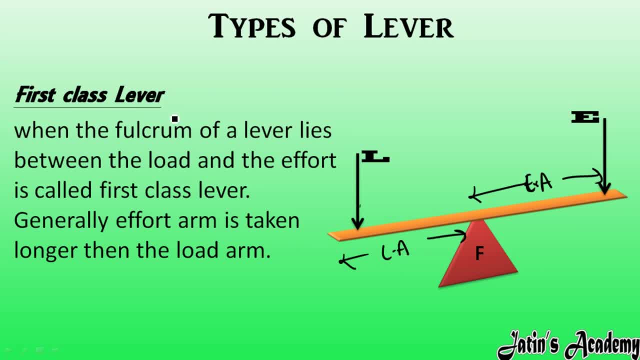 compared to load arm. but yes, in some cases in first class liver, effort arm is also equals to load arm means in some cases fulcrum is in exact center. effort is here, load is here. load is here, then effort arm is approximately equals to load arm. fine, but in some cases of 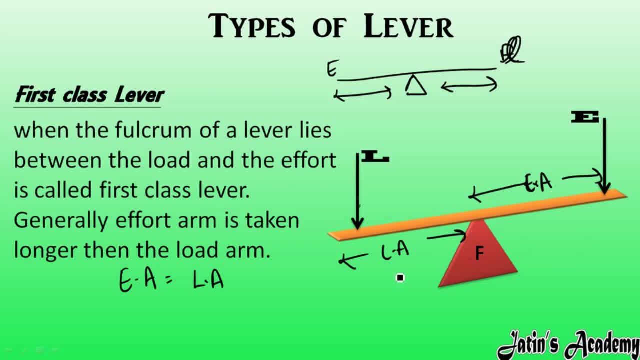 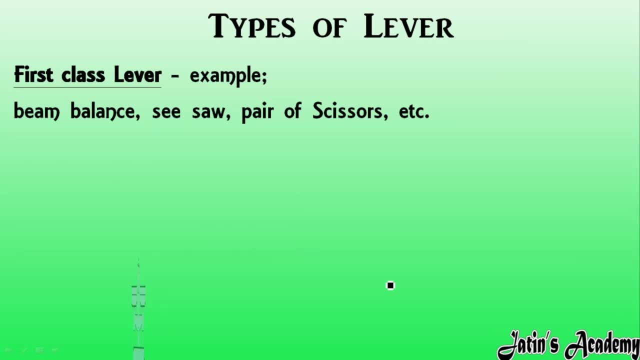 first class lever, we are having effort arm greater than load arm, fine. next we are having examples related to the first class lever, for example. first we are having beam balance. so in a case of beam balance, this is a kind of beam balance. here we are having a fixed point. 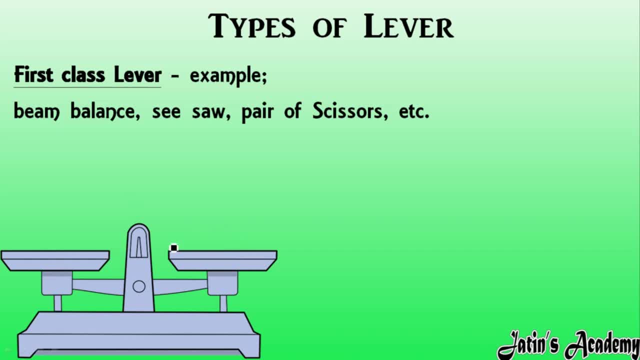 around fixed point these two weights are going to move. this fixed point is known as fulcrum fine and at the normally at the left side, we are using the weights. here we are using the weight means. weight is nothing but a effort applied whatever weights we are using, standard weight that we are. 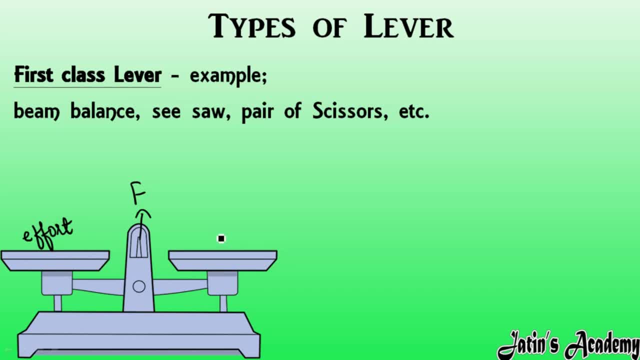 keeping in the left hand side. so here will be effort and here we are calculating the load means. whatsoever material we have to calculate, we are keeping it here. so here we are having a load. so see carefully what is happening here. actually. here fulcrum is in center effort and 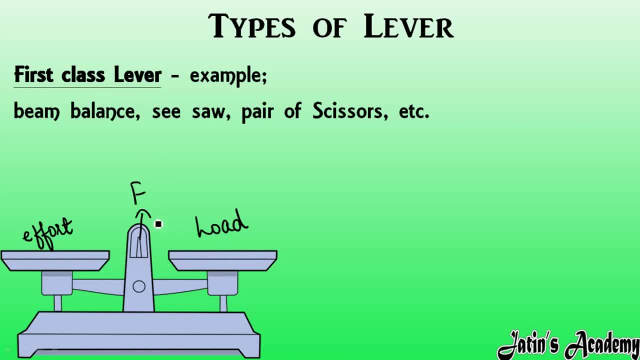 load are on other side. so this is which class lever, first class lever, fine. similarly, we are having a second example with seesaw in a seesaw. see carefully, this is a fixed point around which these two boys are going to rotate. okay, these two cartoons are going to rotate. so this fixed point. 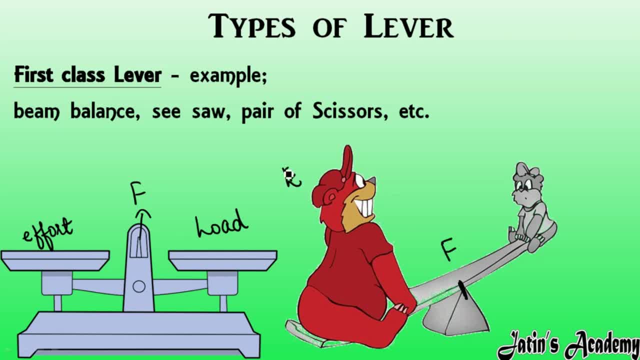 is in center. here we are having effort, here we are having load. or you can change also: this is a load or this is the effort, no problem. so fulcrum is in center. load and effort are on sides. means it is a first class lever. means whatsoever: example is coming for you. you have to just check the arrangement. whatever, wherever the 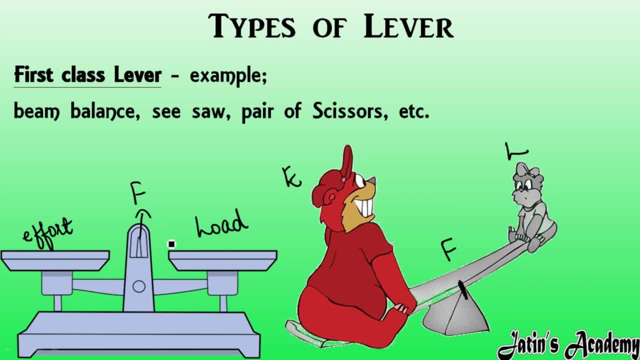 objects are kept or wherever the fulcrum, load and effort is kept. by watching that, you can just clearly know which kind of lever is there, fine. next we are having with a pair of scissors in a pair of scissors, carefully around this fixed point. this scissor is going to rotate or move. okay, this fixed point is. 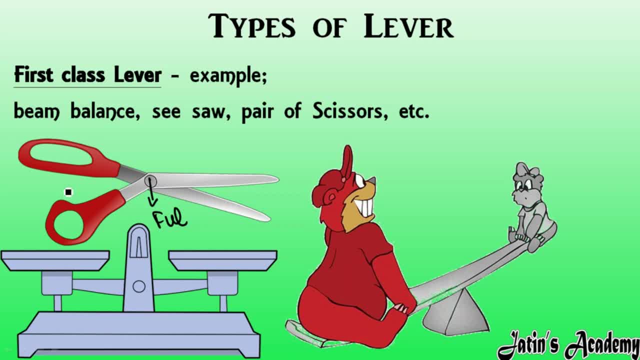 known as fulcrum, and we are going to apply force here on the hands of scissors. so here, wherever we are going to apply force on a machine, that is known as effort, and here we are having load means. here we are going to put a piece of paper or cloth in order to cut it, so here we are having a load. so 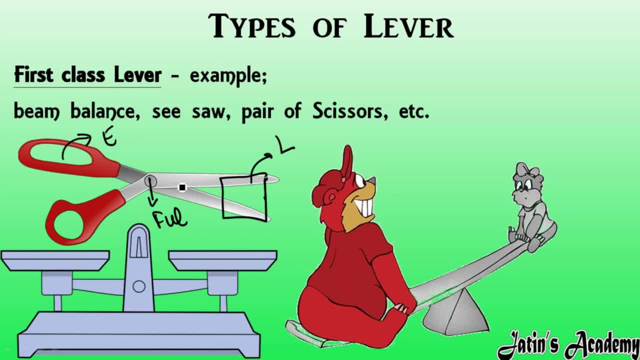 you can see carefully, you can see properly that fulcrum is in center load which is below the crush Naphtha. it is a first class lever. then fluid is called first class moving, the last flavor that goes on. first class can be hanging これ stripe l side. so scissor is which glass liver? Caesar is first class, leware, fine. 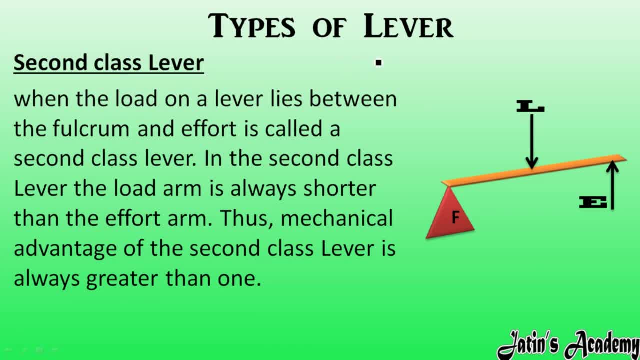 next we are having second class liver. so as I taught, told a formula: flea according to flee, second class lever load should be in center. so here same load is in center. so when the load on a liver lies between fulcrum and effort, that kind of liver is known as second class liver. so in a 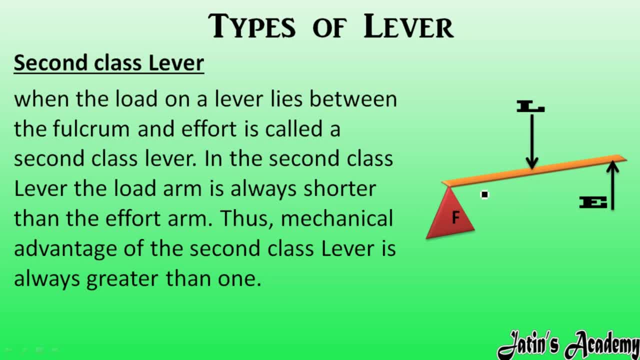 second-class liver. see carefully: here we are having fulcrum, here we are having load and, as we know, distance between the load and fulcrum is called load arm. this is load arm, and distance between the fulcrum and effort is effort arm. this is effort arm. fine, so see carefully. in a second 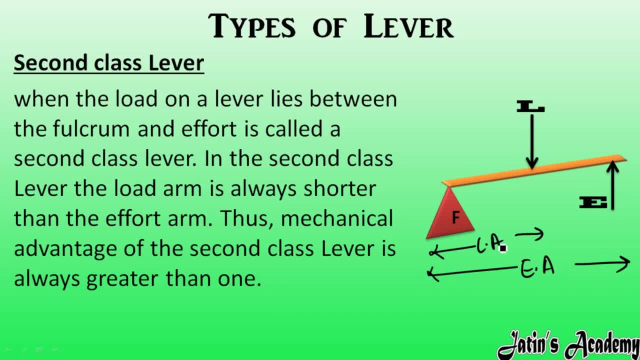 class lever: effort arm is longer as compared to load arm. okay, so see carefully. i will tell you the mechanical advantage also. actually here mechanical advantage formula is effort arm over load arm. okay, mechanical advantage formula we have studied only that: effort arm over load arm. see carefully in second class lever, as you can see, effort arm is more as compared to load arm. 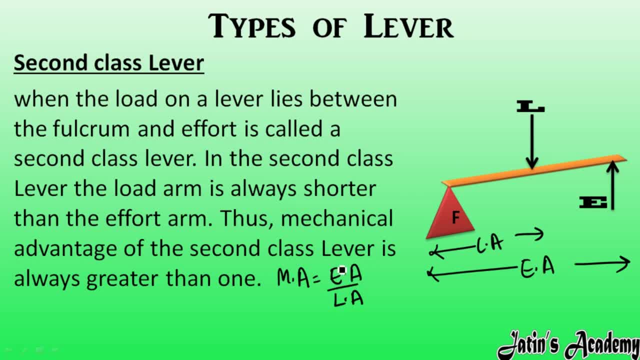 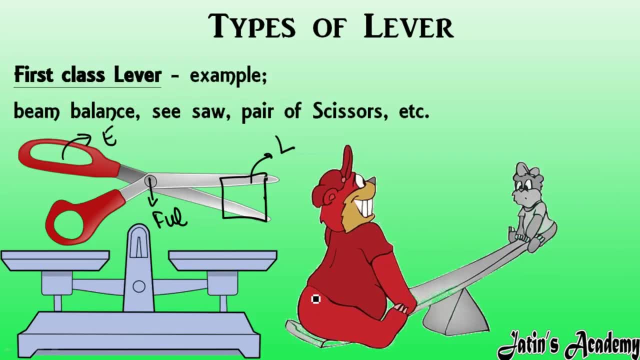 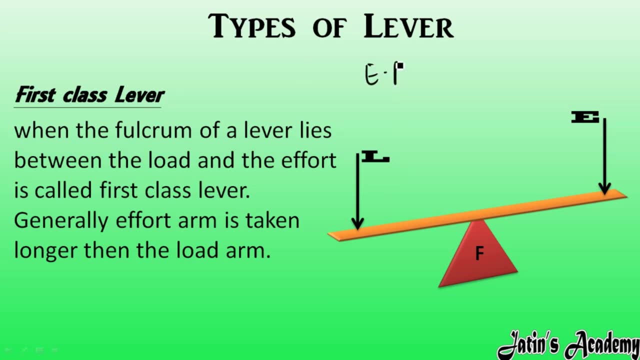 means effort arm is longer. if effort arm is more, then mechanical advantage is also more than or greater than one. fine, just see the first class lever. also in first class lever- see carefully, in a first class lever actually in somewhat cases effort arm is taken longer as compared to load arm. if effort arm is taken longer than load arm, then mechanical 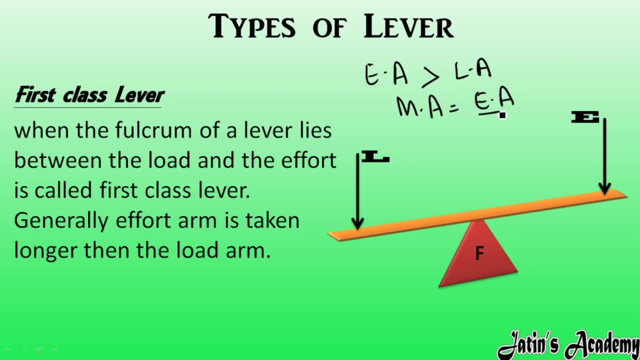 advantage will be what mechanical advantage is effort arm over load arm? if effort arm is more means mechanical advantage is greater than one. but in some cases in first class lever, effort arm is exactly equals to load arm. so here mechanical advantage is what mechanical advantage is one. if effort arm and load arm are approximately same, then mechanical advantage is one. but if effort arm 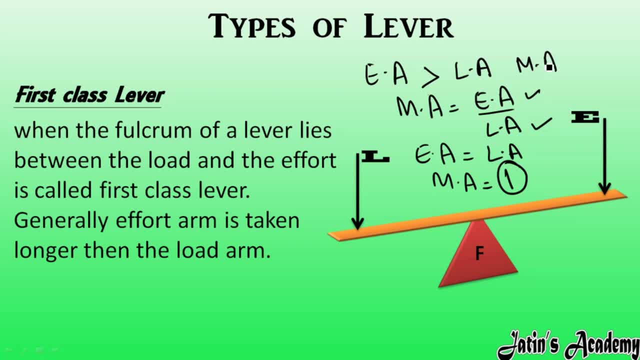 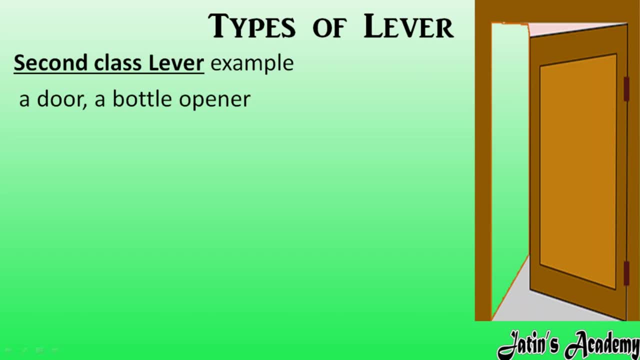 is greater than load arm. in that case mechanical advantage is greater than one. fine. next we are going to start with the examples of second class lever. so firstly i will draw the basic diagram for second class lever. basic diagram for second class lever is like this here in this case: 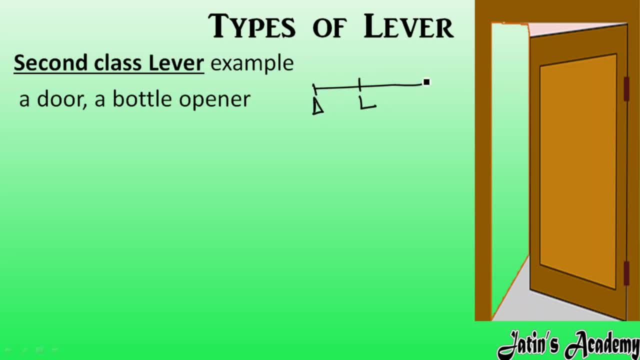 load is in center, fulcrum is on side and effort is on side. okay, so in a case of second class lever, first we are having the example of a door. so in a case of door, what we are having in a case of door, from here, from the handle, we are applying the force in order to move the door. so this is acting. 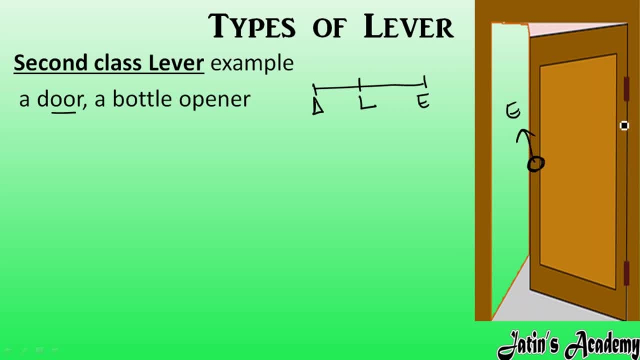 like a effort. okay, and these are the fixed point about which door is going to rotate, and this fixed point is called fulcrum and full-fledged door is acting like a load. so see from this diagram and see from this diagram, compare it: here we are having fulcrum, here we are having load and here 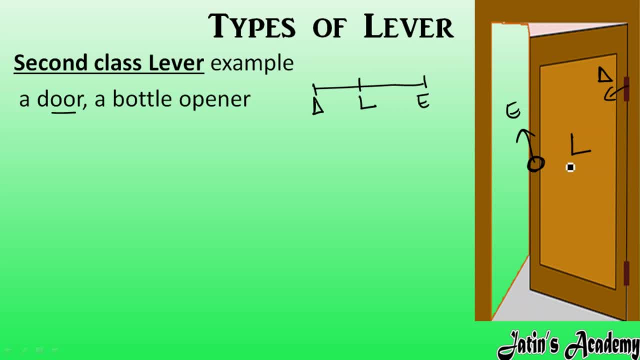 we are having effort means in between fulcrum and effort, we are having a load, so this door is acting like a second class lever. next example related to second class lever is bottle opener. so in a case of bottle opener, what we are doing in order to open the cap of the bottle, we are applying the 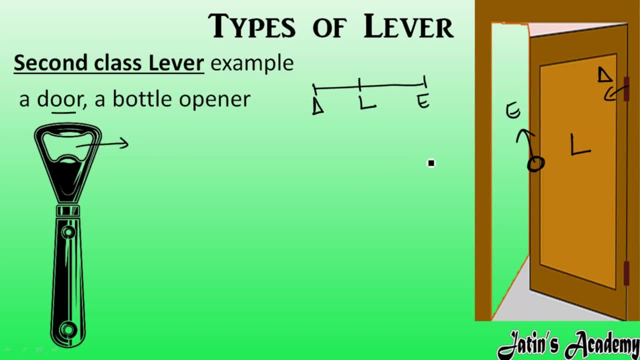 cap here means load. we are attaching here in center, so this is known as load. okay, and we are applying force from here, this part part where, from where we are applying the force is known as effort, and this is a fixed point about which that bottle opener is going to move. this fixed point is known. 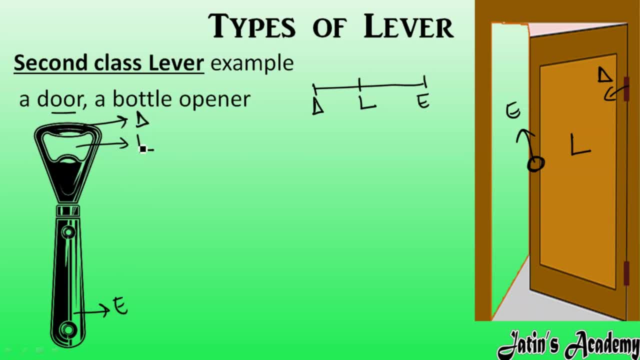 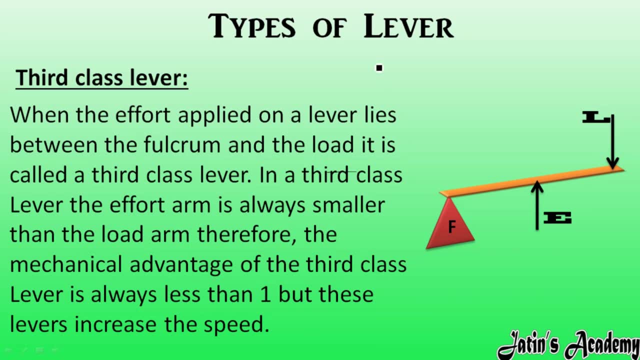 as fulcrum, between fulcrum and effort. we are having a load, so this is an example of second class lever. we are having third class lever. so in a third class lever we are having like this, as you know, the formula flea, f, l, e, e means in a third class lever, effort is in center, between fulcrum and load, so in between, 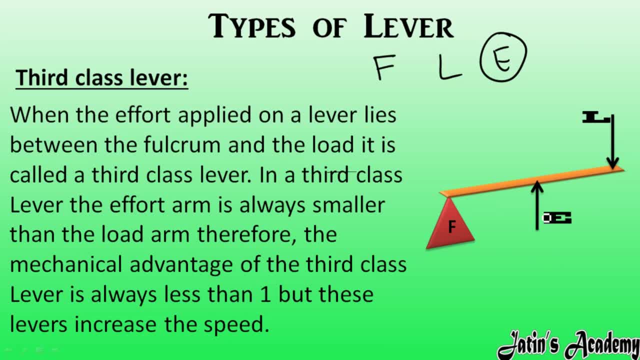 fulcrum and load, we are having effort. this kind of lever is known as third class lever. in a third class lever- see carefully- fulcrum is here and effort is here. so distance between fulcrum and effort is effort arm. and distance between fulcrum and load is load arm. so 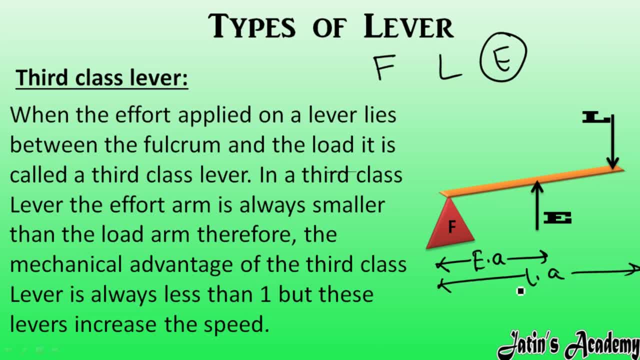 properly from the diagram, you can see clearly. you can see that load arm is greater than effort arm and, as we know, mechanical advantage formula, mechanical advantage is equals to effort arm over load arm. okay, and here load arm is greater and mechanical and effort arm is less. if effort arm is less means mechanical advantage is also less. less than what? less than one mechanical? 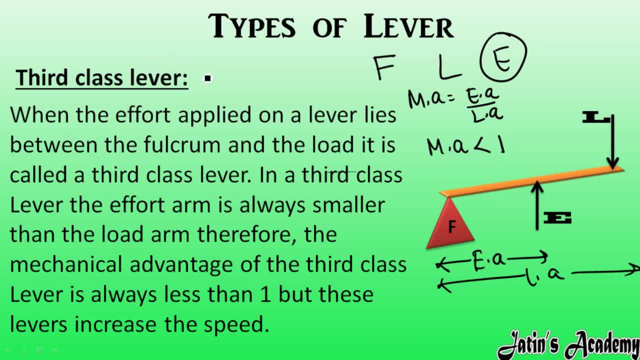 advantage is less than one in a third class lever. fine, and what is the use of this mechanical advantage? equals to one, greater than one. actually, here, in this case, as we have studied, in a first class lever, mechanical advantage is equals to one. equals to one means whatsoever, effort we are. 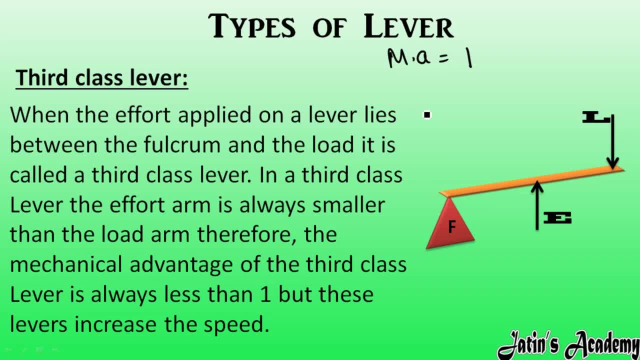 applying on the body or on the simple machine same kind of same kind of work. we are applying work that simple machine is also going to do, same kind of force that simple machine is also going to apply on the load. this is a means of mechanical advantage. is equals to one in a second class lever. 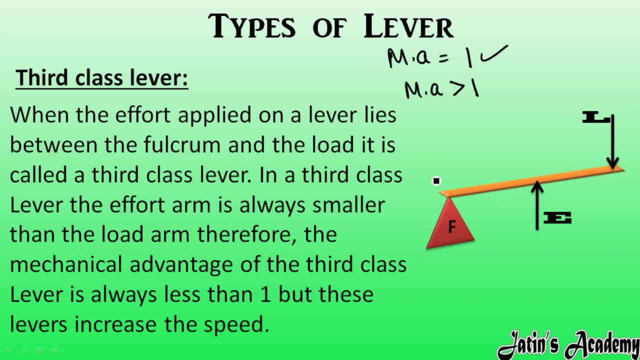 we have learned that mechanical advantage is greater than one. what do you mean by this? actually, mechanical advantage means effort over load, sorry load, sorry load over effort. mechanical advantage greater than one means whatsoever work we are going to apply or whatsoever effort or force we are going to apply on a simple machine. in return, machine is going to show us more force on. 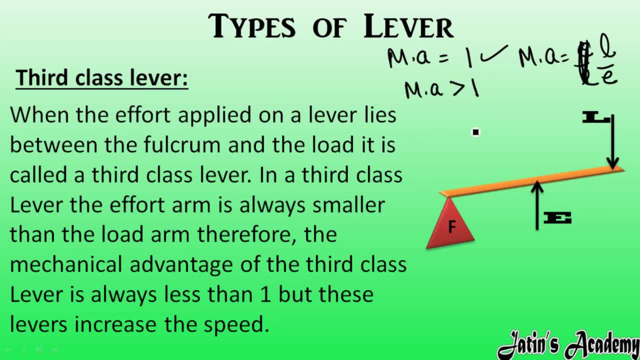 the load. so mechanical advantage greater than one means more and more kind of force simple machine is going to show in order to move up, or any in order to take the object. okay, and in third class, lever, mechanical advantage is less than one. mechanical advantage is less than one means. 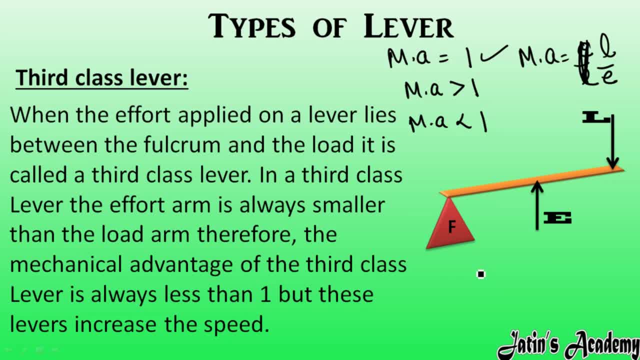 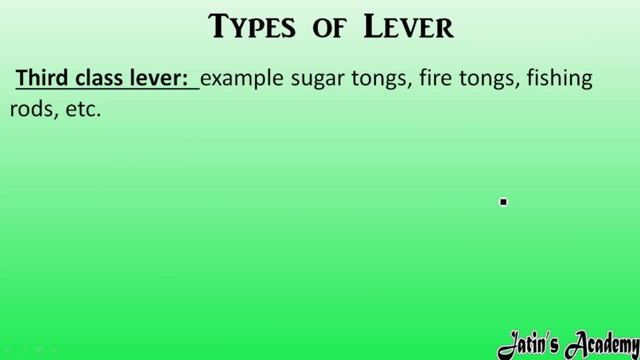 we are applying more and more force on the effort. but simple machine is not showing that much force on the load. that is why in a third class lever mechanical advantage is less than one fine. next we are having third class lever examples. first we are having sugar tongs, so in 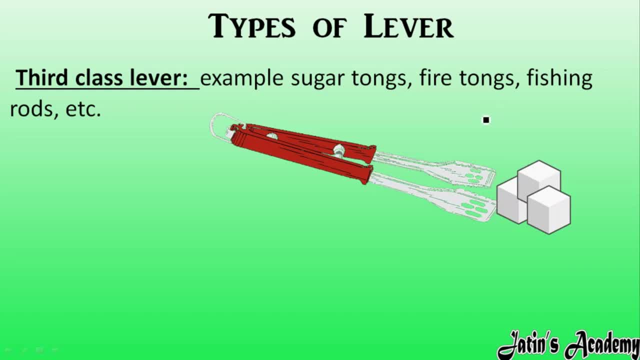 a case of sugar tongs. this is a third class lever. firstly, i am going to draw the diagram for third class lever. in a third class lever, f, l, e, flea means effort is in center, fulcrum is always on left side and load is here. fine. so here, see carefully. here we are. 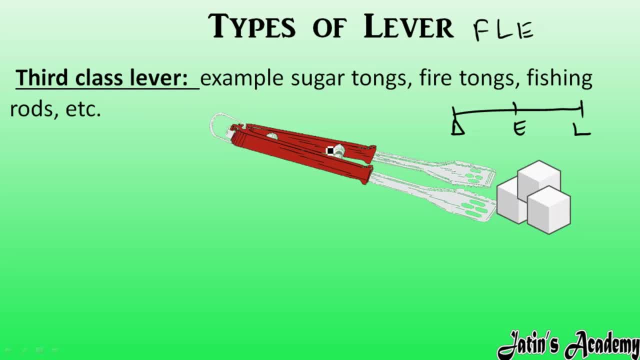 having a fulcrum means about this fixed point. this sugar tong is going to move. this is a fulcrum. here we are going to apply the load means here only, from here only, we are going to pick up the sugar. fine, this is a load. and in between, here we are going to apply the force. this is known as 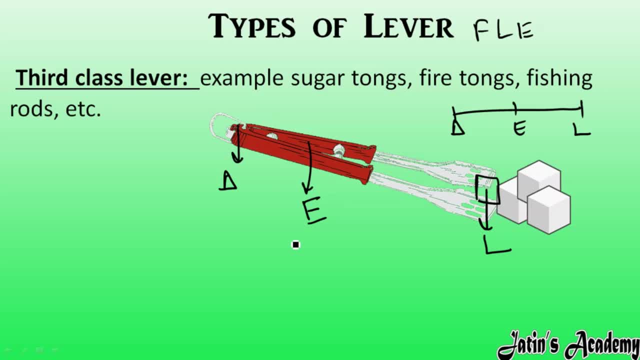 effort. so see carefully: effort is in center, effort is in center means. this is which kind lever? it is third class lever, okay. next we are having similar example of fire tongs. also here we are having a fixed point. that is a fulcrum. here we are going to apply force from. 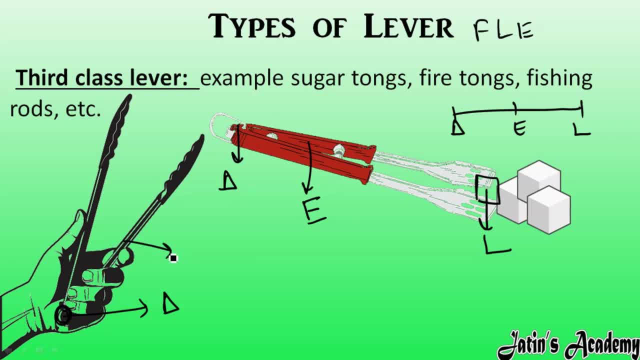 these points we are going to apply the force, so it is a effort. and here we are going to put some kind of load in order to move it or in order to use it. that is a load, okay. so here effort is in center. when effort is in center, we are having it as third class lever. fine, similar example: we are 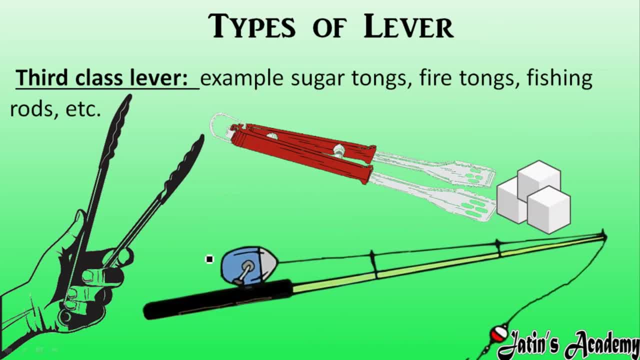 having with a fishing rod. so in a case of fishing rod also what we are having in first case, here we are having a fixed point, here we are having a fulcrum- sorry, here this is a fulcrum- about which, fixed, this fishing rod is going to move and here we are applying the effort on this means handle. 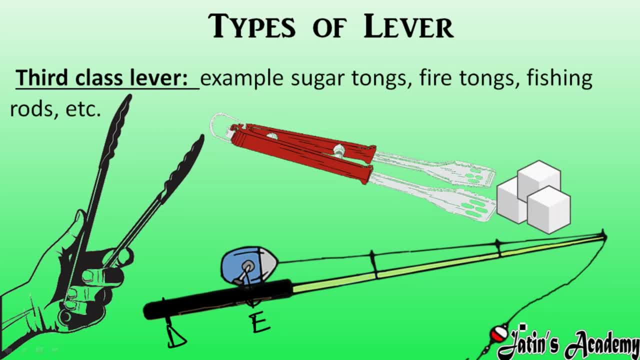 we are going to apply the effort. this is the effort, and from here we are going to pick up the load. this is a load, so here you can eat clear, clearly see that effort is in center. when effort is in center, this is which class lever. it is a third class lever, fine. next we are having numericals. 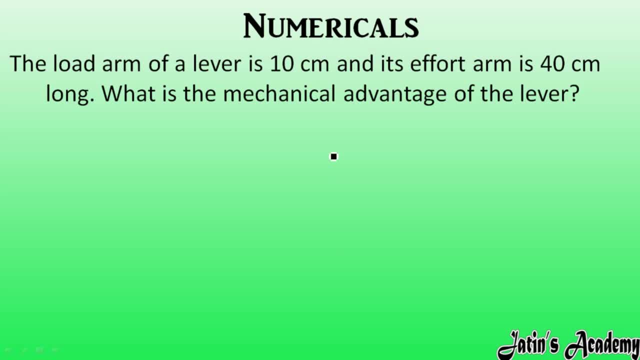 related to numericals, related to lever. so, firstly, write the formulas of the lever. first formula we are having: mechanical advantage is equals to load over effort. second formula we are having: mechanical advantage is equals to effort, arm over load arm. these two numericals, these two formulas we are 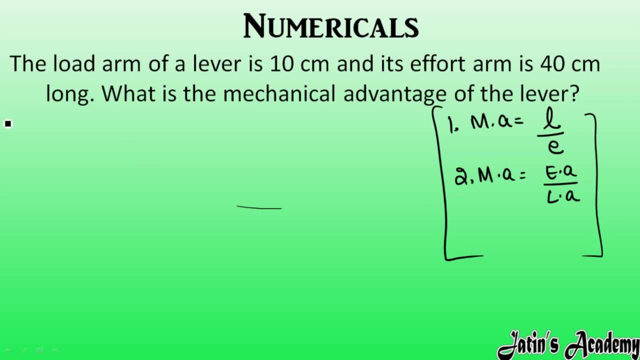 going to use in order to solve the numericals. so see carefully. first numerical: the load arm of a lever is 10 centimeter. we are given with load arm, right load arm is equals to 10 centimeter and effort arm is this and effort arm is given 40. 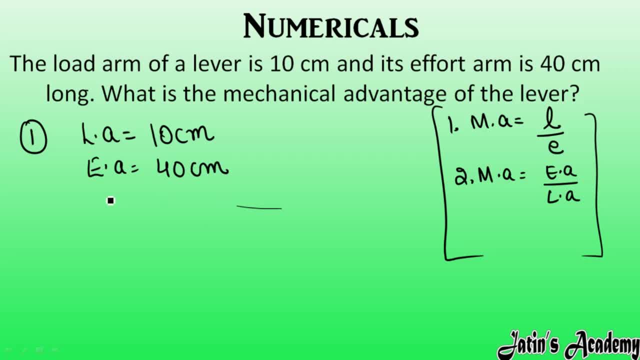 centimeter. okay, what is the mechanical advantage of a lever? so, mechanical advantage of a lever, we have to calculate and, as you can see from these formulas, effort arm and load arm is given. so which formula you will apply, first or second? yes, you will apply the second formula. so what the second? 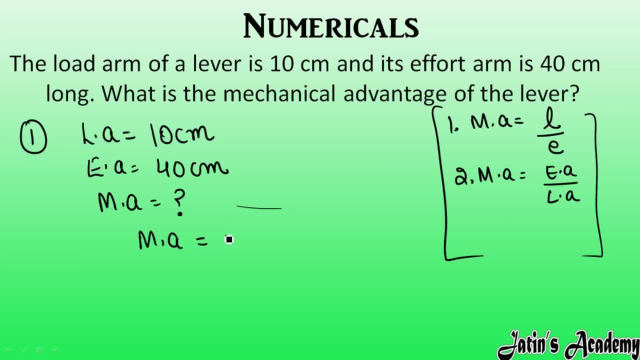 formula is. second formula is: mechanical advantage is equals to effort arm over load arm. fine, so what is the value of effort arm that is 40 over? what is the value of load arm 10.. so 0 cut with 0 we are having mechanical advantage is equals to 4.. and what is the unit of mechanical? 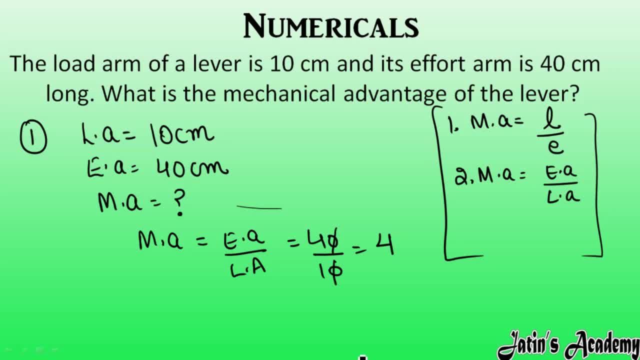 advantage? tell me the unit. mechanical advantage is having no unit. why? because effort arm and load arm, both are in centimeter. here also centimeter, here also centimeter. centimeter, centimeter will cut with each other. so we are having no unit of mechanical advantage. simple way to calculate the: 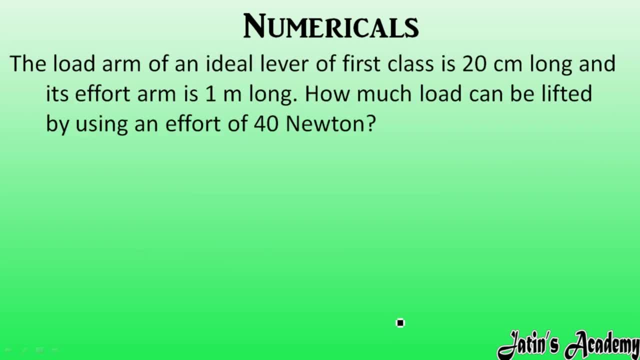 mechanical advantage is equals to four. next, we are having second numerical related to this. so second numerical we are having the load arm of idle lever is 20 centimeter long. so load arm we are given with 20 centimeter and its effort arm is one meter long. effort arm we are given with one meter. 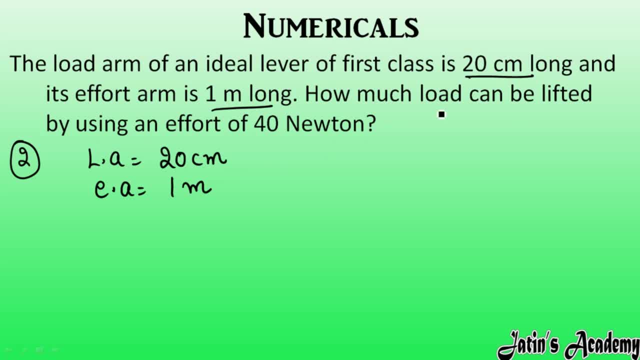 long, how much load it can be lifted, how much load means load. we have to calculate by using an effort given with. effort is equals to 40 newton. firstly, i will write the formulas here. first formula we are having: mechanical advantage is equals to load over effort. second formula of mechanical advantage: 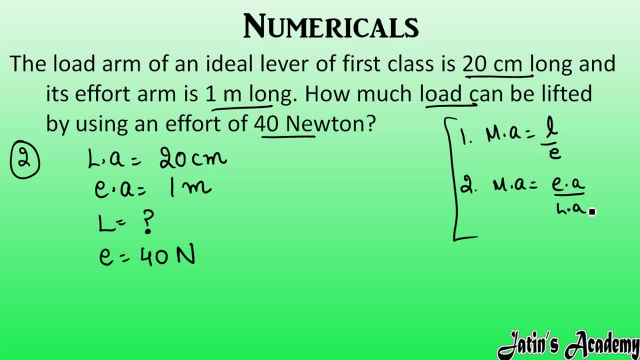 we are having effort arm over load arm. fine, see carefully here. effort arm is in centimeter. sorry, load load arm is in centimeter and effort arm is in meter. firstly, convert the both units into a single unit. i will convert this meter into a centimeter, which is easily. 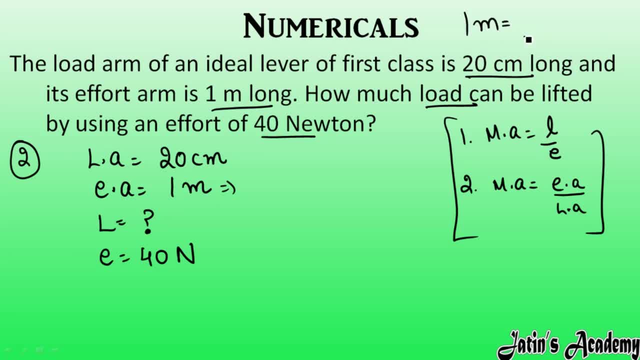 to convert. so one meter is equals to how many centimeter? one meter is equals to 100 centimeter, so one meter means here you can write 100 centimeter. fine, now see the formula in order to calculate the load. what we will do means they are not given to solve with mechanical advantage. they 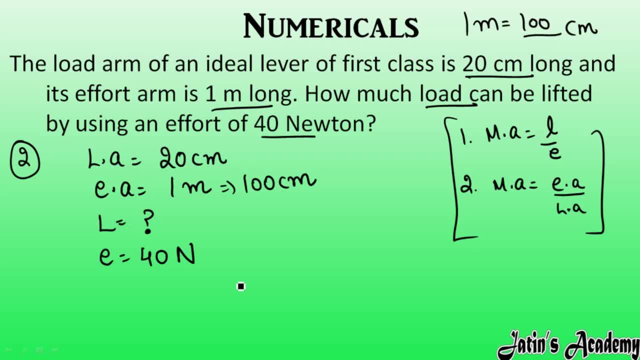 told us to solve with the load. we have to calculate the load, so which formula i will apply? i am not getting how i will apply the formula. so third thing we are having with the principle of lever formula. i will tell you the same which we have studied in the previous slide. also, that is effort. 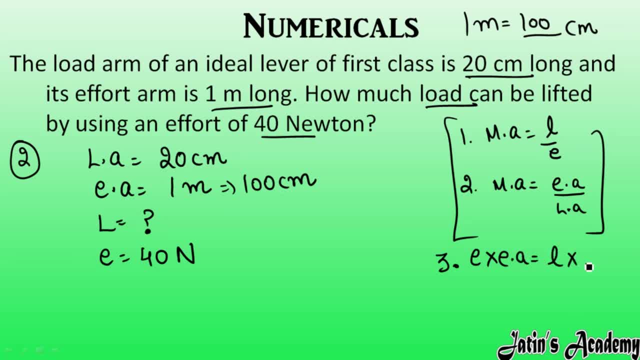 into effort arm is equals to load into load arm, which is nothing but a principle of lever. fine, so we will apply this formula. why? because we are given with effort, we are given with effort arm. we have to find load. we are given with load arm. so we are going to use this formula. 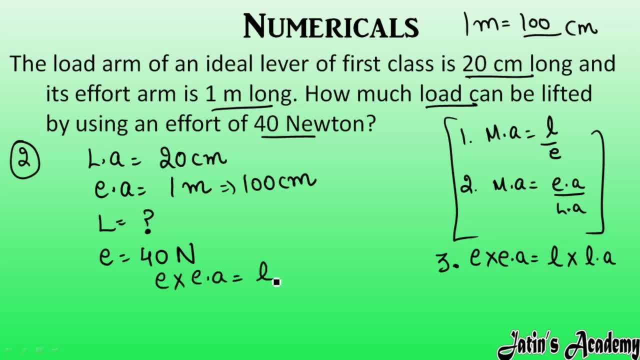 so write it here: effort into effort arm is equals to load into load. arm means according to conditions. we will see which formula we are going to apply. so effort is what? effort is 40 newton. now you will see. now you will see that it is in centimeter and here effort is in newton. how this actually? 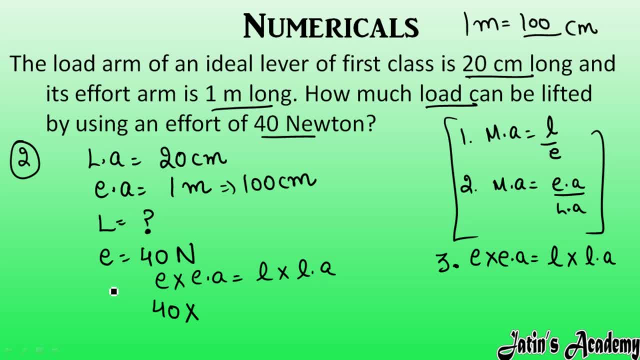 effort is a force applied by us on the machine, so force applied. we know force is a newton. only force as a unit is newton and this is a load arm and effort arm. arm means distance. distance should be in centimeter, so it is units are given right, fine, effort arm is given what? 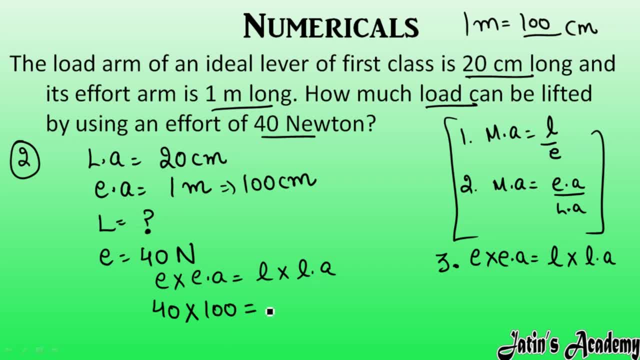 100 is equals to load is given. we have to calculate multiply. load arm is given 20.. so as you have to calculate load, we have to take this 20 to that side. 20 is in multiply. that said, it will go in divide. so here we will see 40 multiply: 100 is same is equal to load is same, 20 is in multiply. 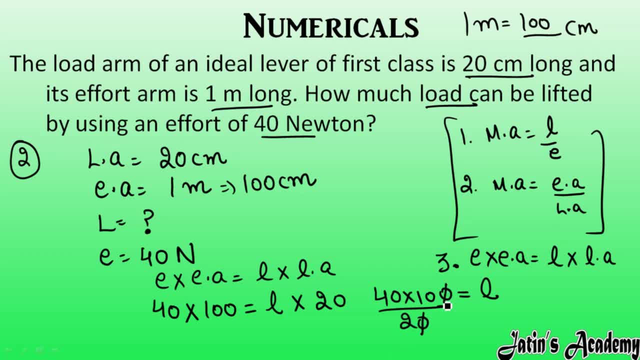 that side it will go in divide cut 0 with 0, two ones are two, two twos of four. twenty will be there, so here load will be two hundred centi newton, sorry, newton load means force applied by machine on an object, that is a load. so 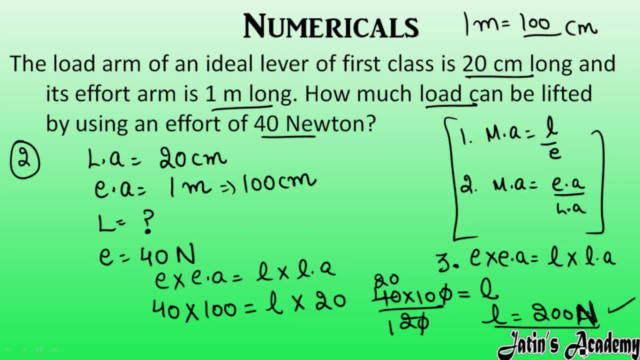 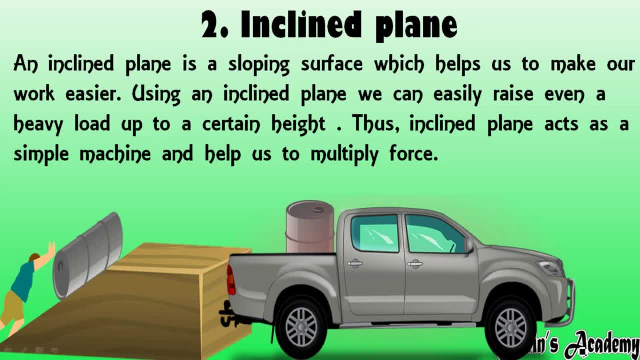 load is a 20 newton. fine. next we are having- we are going to study about- the second kind of simple machine, that is, a inclined plane. so what do you mean by inclined plane? actually, inclined plane is a sloping surface. this kind of sloping surface we are having which help us to make our work. 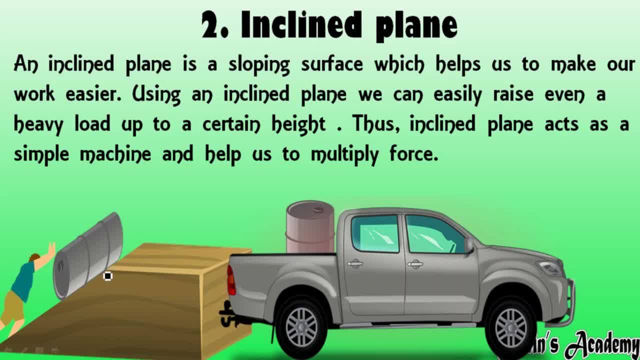 easier might be. you have also seen this kind of inclined plane or sloping surface at your house or in a front of hospitals. fine, so using an inclined plane, we can easily raise a heavy load means, if you want to raise this can on this jeep, just applying your force, applying your muscular. 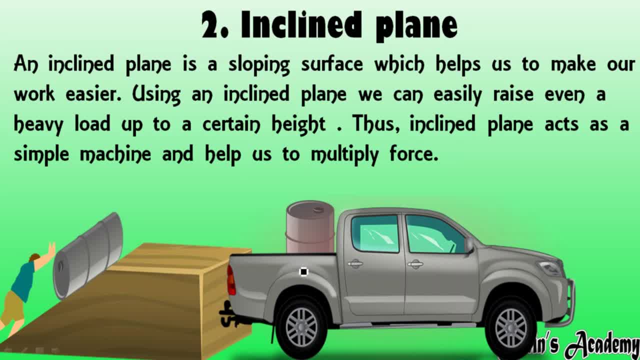 force and taking it up and putting into the car. it is very difficult, okay, but we can make our work easier by using this inclined plane. just use this inclined plane and apply little force. so by applying little force, it will move up and it will go into the car or jeep, okay. so this is 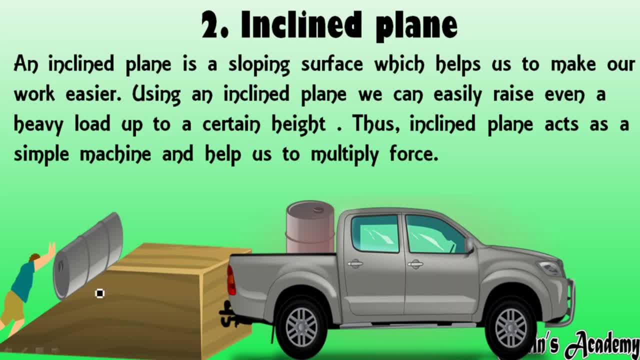 an inclined plane which makes our work easier and faster, how it can easily raise a heavy load into a certain height, up to a certain height, so this inclined plane act as a simple machine. so whatsoever things which make our work easier and faster, like this inclined plane is making our work. 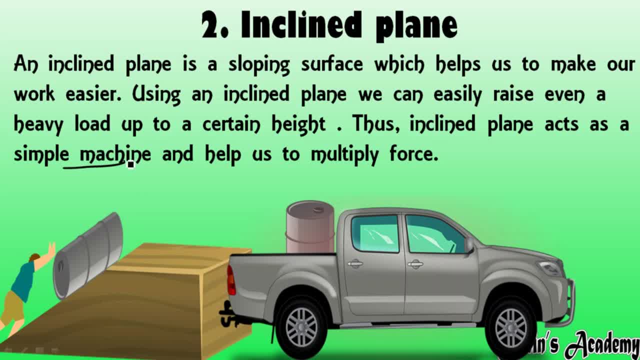 easier and faster. this inclined plane is nothing but a simple machine. plus, it is helping to multiply force. also, what do you mean by multiply force means even though applying less force, we are going to, we are going to raise the very heavy load. okay, so it is going to multiply. 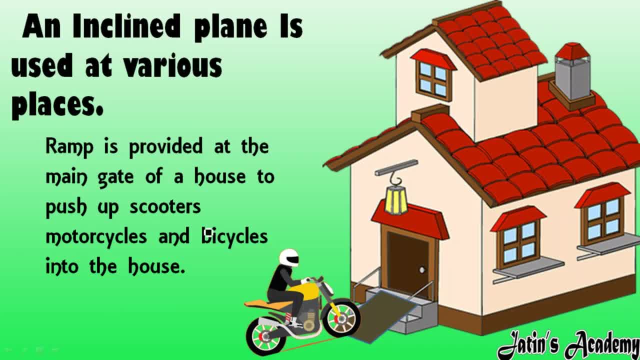 our force. fine. next we are having an inclined plane is used at various places. might be you have seen this kind of examples at your home. also means in a front of home ramp is provided. why ramp is provided at the main gate of the house to push up the scooters or motorcycle or 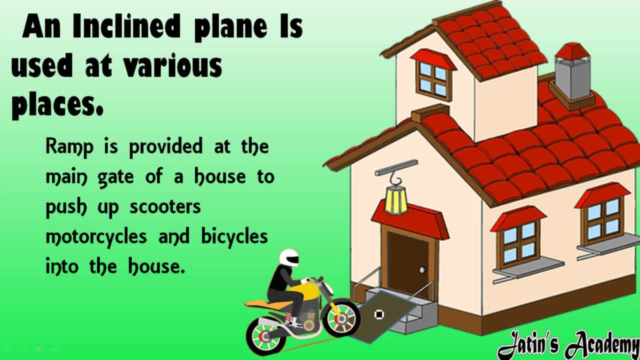 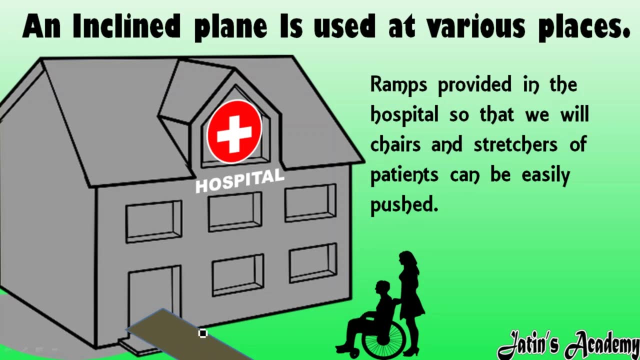 bicycles into the house. by using this kind of ramp we can easily push up the scooters motorcycle into the house by using an inclined plane or a simple machine. next, we are having in front of hospitals, so ramps are provided in the hospital so that wheelchairs or stretchers can easily move. 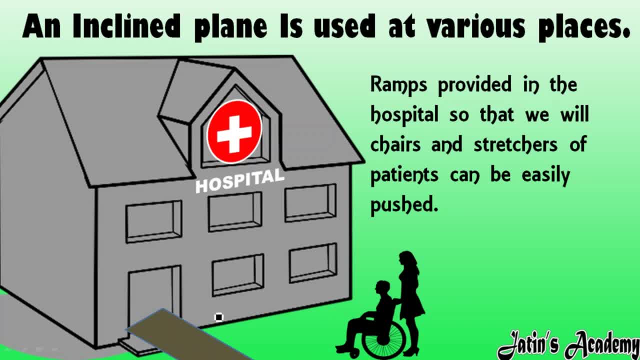 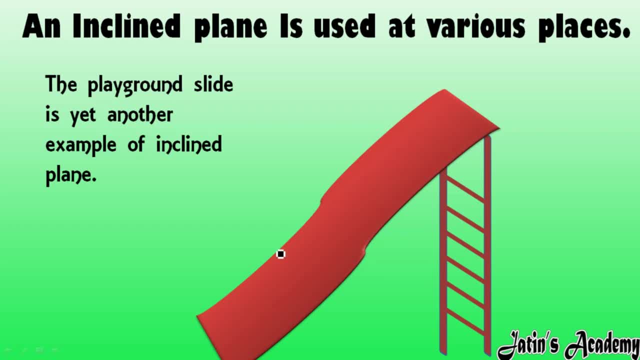 into the hospital by even though applying less force. next we are having- this is your favorite example: playground slide. so might be. now you are going to link it with your daily life. the playground slide is also another example of inclined plane means. by applying even though less force, you are coming with a more force here. okay, so next, kind of simple. 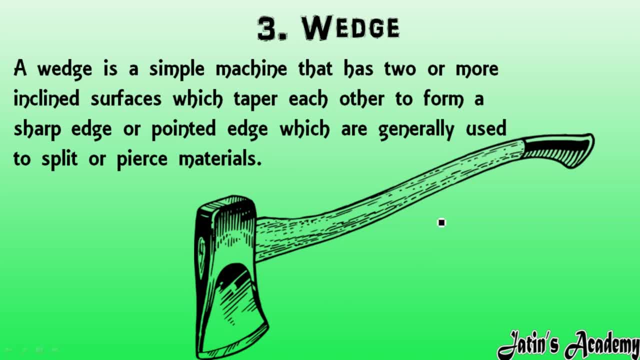 machine we are having a wedge. so wedge is also a simple machine in which two or more inclined planes are there. how inclined planes are there? see carefully here: one: this inclined plane is there. second: this inclined plane is there and this is also acting like a inclined plane. 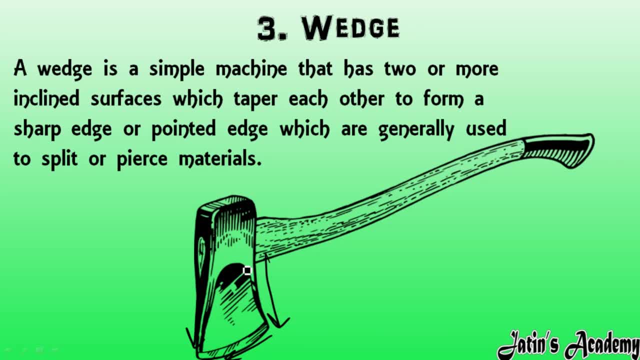 This means wedge, is that simple machine where two or more inclined planes are tapper together, or means fixed together to form a sharp edge. here two or more simple machine or two or more inclined planes are combined together to make a sharp edge or a pointed edge, and 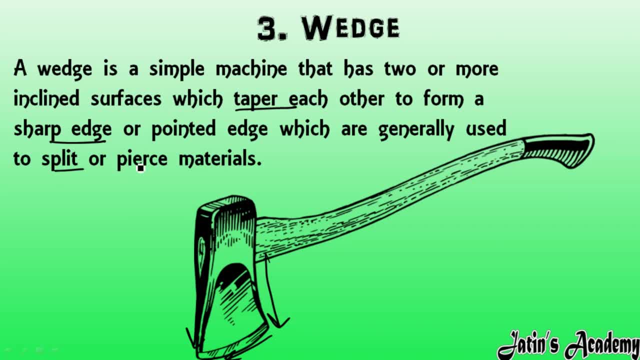 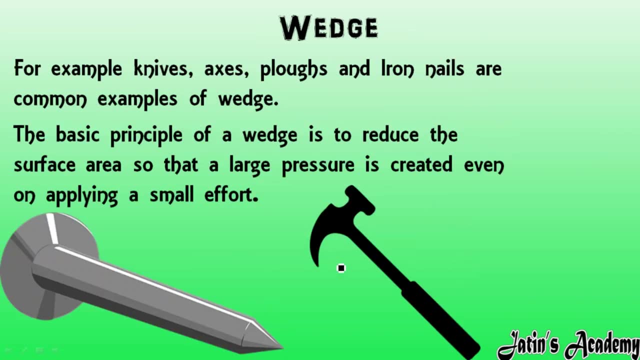 this wedge is generally used in order to split or purse material. purse is also means to split the materials into two halves. so in order to cut the material, in order to cut the material into two halves, we are using this kind of wedge. fine, so, for example, of wedge like knife. 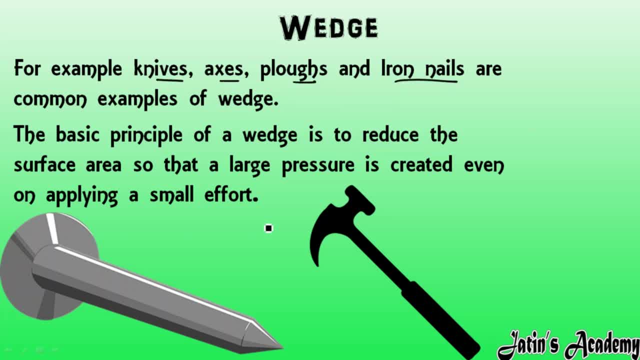 axis, love, iron nails. these all are the examples of wedge where you can easily see that two or more kind of inclined planes are joined so that it can easily, like cut the materials into two halves, or it can easily make the materials to move together. okay, so the basic. 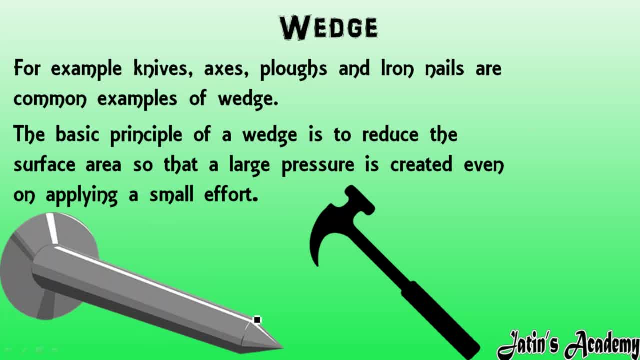 principle of the wedge is to reduce the surface area. actually, what we are doing in a case of wedge by using two inclined plane at one point, we are decreasing the surface area. whenever we are decreasing the surface area might be you are knowing this formula or no. I dont. 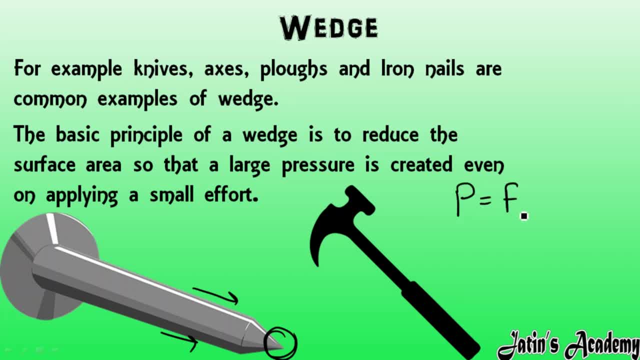 know formula is: pressure is equals to force over area. this is the formula we're having for pressure. if we're having an object of very less area, we're having an object of very less area. that object will apply more and more pressure into any object, even though by applying small effort or 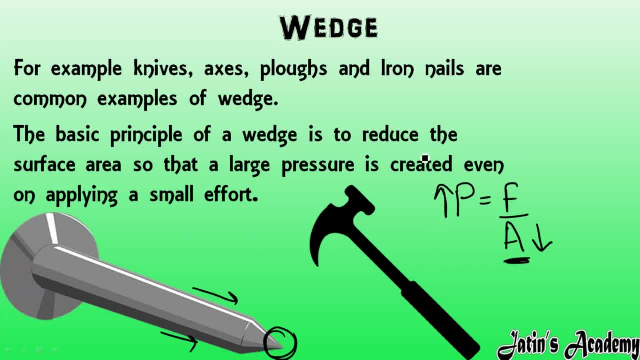 small force on that object, that object will move with a more pressure. fine. so this is a basic criteria. means, if you want to cut this log, we are using a, for example knife, or x. we are using axis. we are using fine in axis. actually we are having a very reduced surface area, reduced surface. 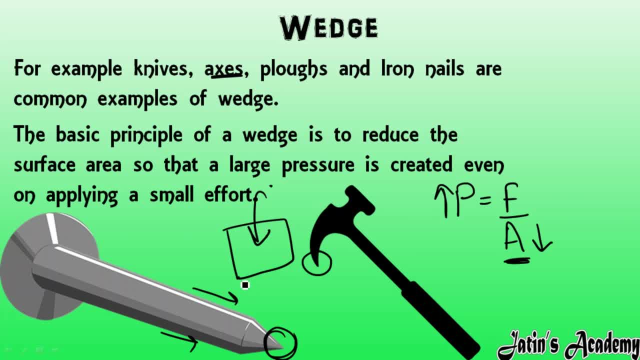 area means this x will produce more and more pressure in a wood log and it will cut the wood or split the wood log into two pieces. so the basic principle is: between is behind this. it will. we will reduce the surface area of the wedge in order to increase the pressure on any object. 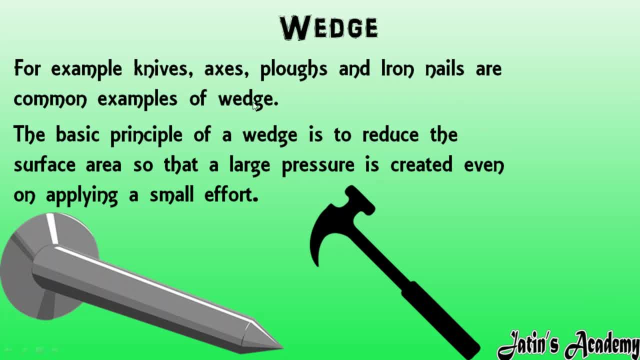 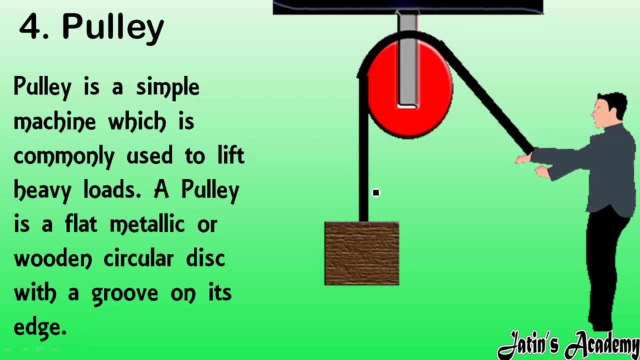 next type of simple machine we are going to study, that is a pulley. so what do you mean by a pulley? pulley is a simple machine. pulley is also a simple machine which is commonly used to lift a wood log. so if you want to lift a wood log, you can lift a wood log by using a simple machine. 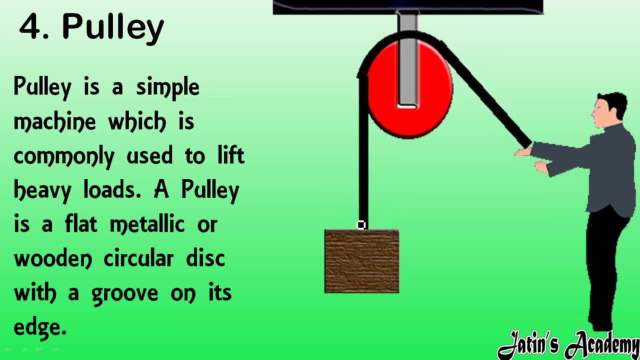 up a heavy loads. so, in order to lift up a heavy loads by applying our muscular force, in order to lift this heavy load, it is very difficult to do this task. fine, so by using this pulley, we can easily lift up a load by applying small effort or small, uh force. fine, so this is a pulley. 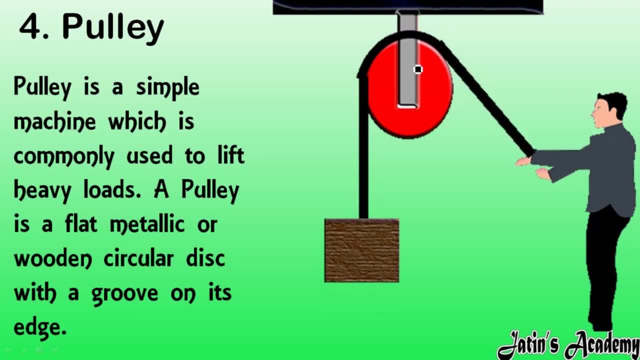 the arrangement of pulley is like this: a pulley is a flat metallic or wooden circular disc which is having one groove on. it means on a pulley- this on a circular disc- one groove is there. groove means hollow surface. is there, on this hollow surface, one rope is attached. 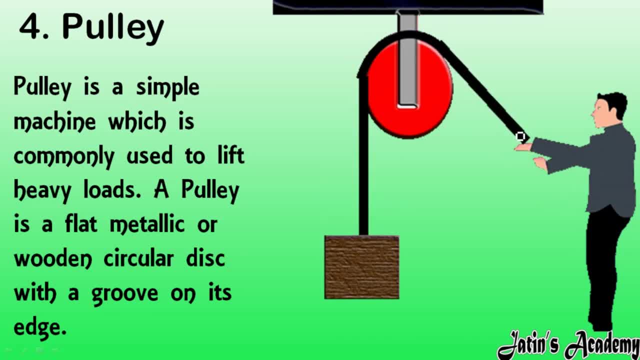 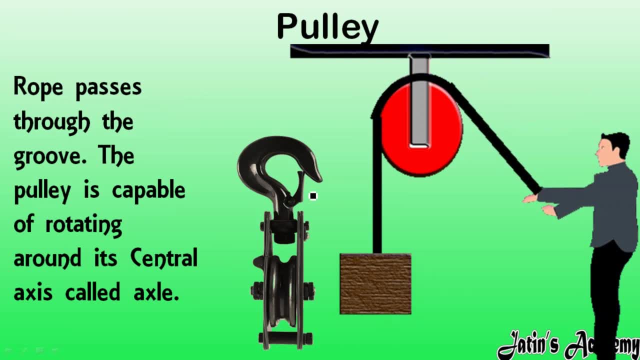 one end of the rope is going to. on the one end of the rope, we are going to apply effort and on the other end of the rope, we are going to lift up the load, fine. next we are having rope passes through the groove, from this groove, from this hollow surface. 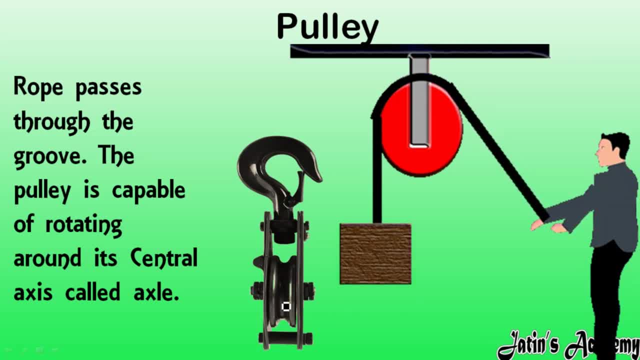 rope is going to pass. this kind of pulley you can see inside this hollow surface is there? so from this hollow surface rope is going to pass. like this, the pulley is capable of rotating the central axis. means this pulley can rotate about its central axis, this fixed point. 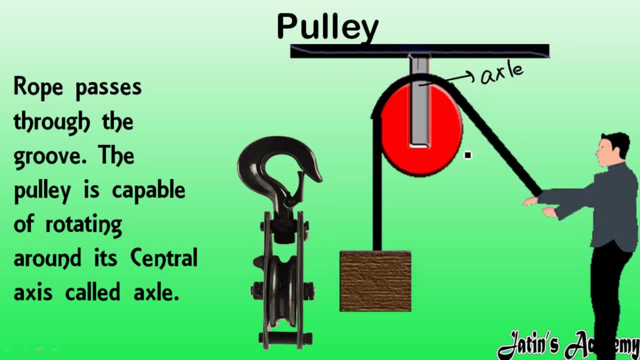 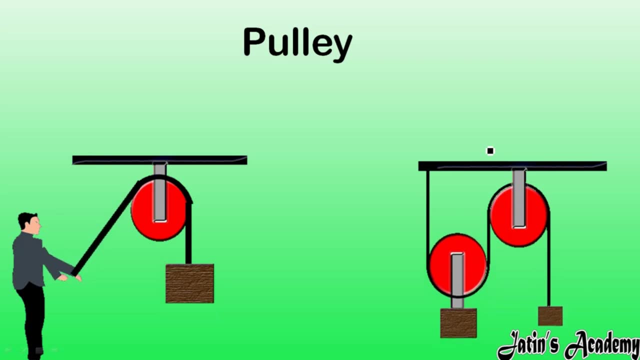 is known as axle, about which the pulley is going to rotate, and axle is also attached to some rigid sport. okay, here at a rigid sport, axle is attached and around the axle, about the axle, this pulley is going to rotate. next we are having kinds of pulley. so pulley are of two kinds. first we are having 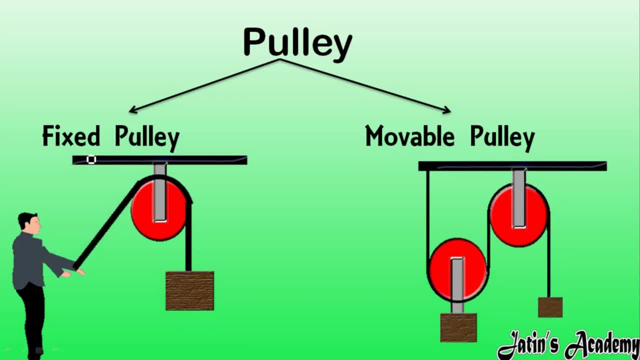 fixed pulley. second, we are having movable pulley, as the name suggests, fixed pulley. fixed pulley is that pulley in which this circular disc or this pulley is fixed at some point. okay, so here rope is there, here also rope is attached. means from the one. 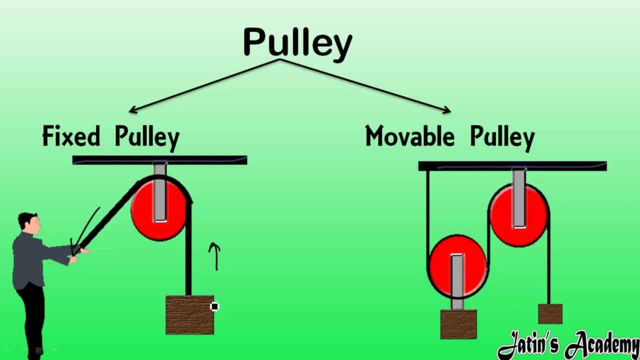 end we are going to apply effort and from the other end, load is going to raise up. and second type of pulley is movable pulley. as the name suggests, movable pulley means in this kind of pulley, pulley is going to move about a fixed point or about this: okay, in order to raise up a load. 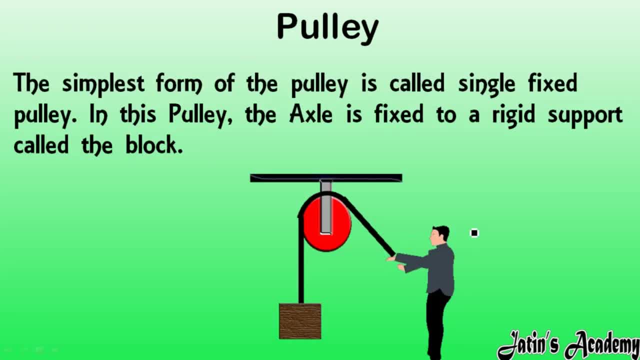 pulley is going to move itself. next, we are having the simplest form of pulley which we are using in our daily life or which you have also seen might be near the well. that is known as single fixed pulley. okay, so in this pulley, the axle. this axle is attached to a rigid sport and this rigid sport 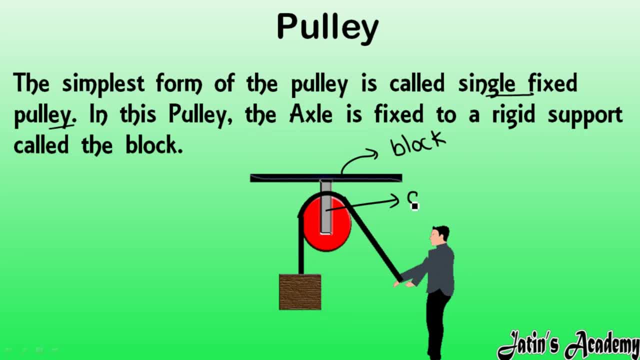 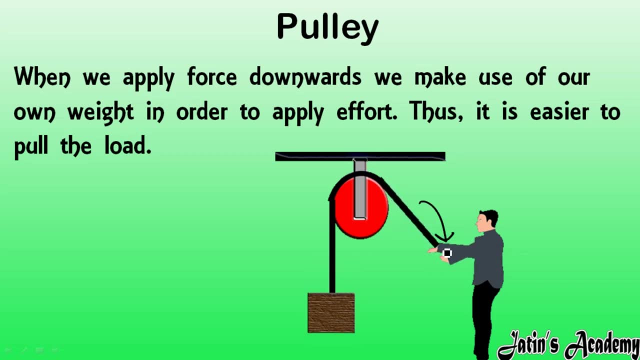 is known as block. this is a axle around which circular disc is going to rotate and this fixed point at which axle is going to attach, that is known as block. next we are having when we apply force downward. whenever we are applying the force to the downward direction from one side of the rope, so means we are applying, we are using our force in order. 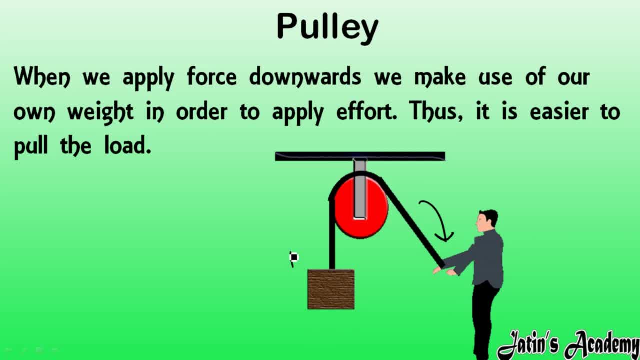 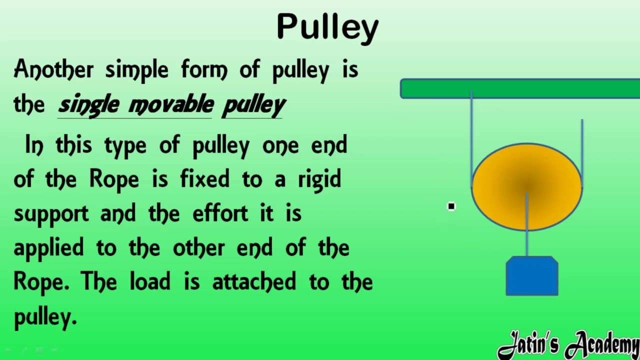 to make the effort. so by applying our force here, weight is going to come outside or weight is going to move upside, so thus we can easily pull the weight by applying a little effort. another form of pulley is single movable pulley. this is an arrangement of single movable pulley in this type. 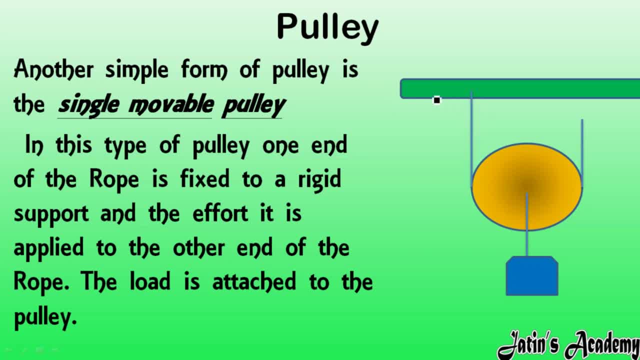 pulley. one end of the rope is attached to the fixed point means one end of the rope is attached to a fixed rigid sport and the effort is applied on the other end of the rope. here also two ropes are there, but one rope is actually attached here to the block. fine, and one end of the rope. here we. 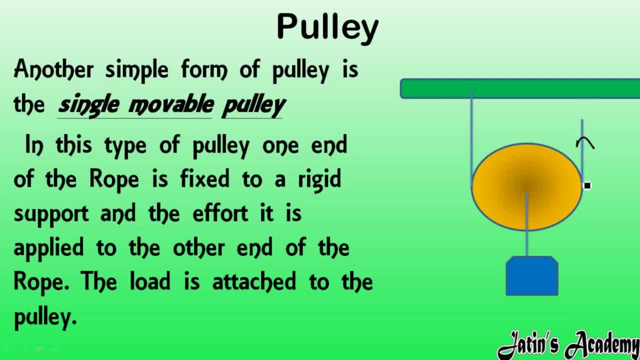 have to apply the effort. whenever we are applying effort here from this side whatsoever, pulley is there. that full-fledged pulley is going to move upside and the load is attached to the pulley. this load is attached to the pulley and when we apply the effort from here, this pulley start. 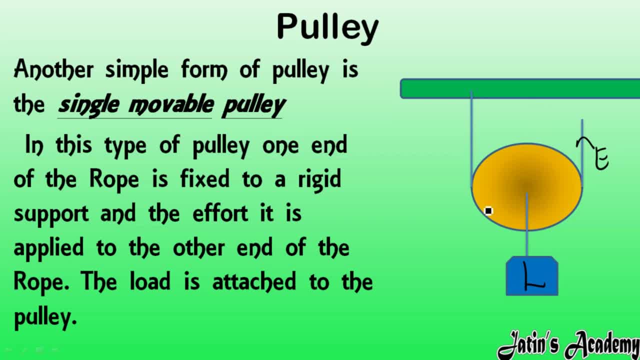 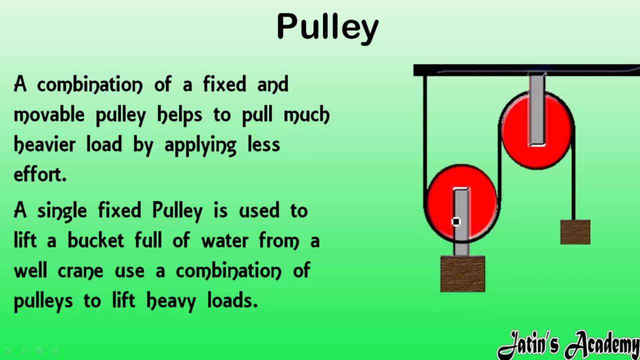 moving upside with the help of pulley. load will also move in the upward direction and the means more. this explanation of the single movable pulley you will study in the higher classes. in this class you are having this much only arrangement and how it is working fine. next we are having a combination. 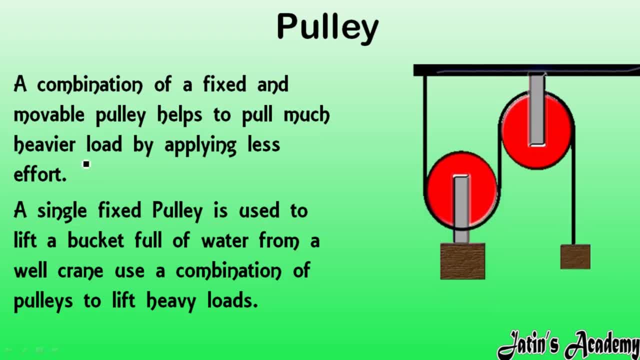 of fixed and movable pulley help to pull much more heavier load. if we are having much more heavier load by using single movable pulley, then also we are not able to move up. by using fixed pulley, then also we are not able to move up. so in that case we are using a combination of fixed as well as. 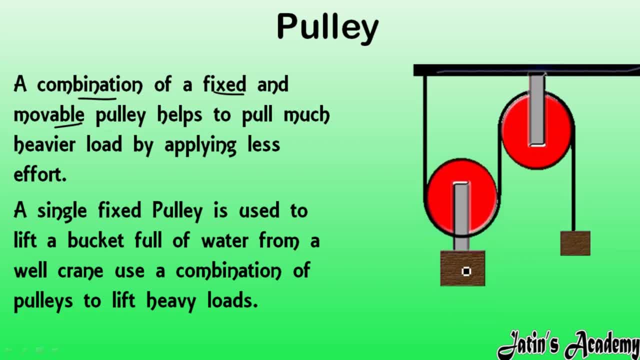 movable pulley in order to lift a very heavy load. okay, this is the arrangement of fixed and movable pulley. so fixed pulley in a single fixed pulley is used to lift a bucket full of water means. might the american municipality equip well in a singleיזbe advance truck that bucket full of water? we are? 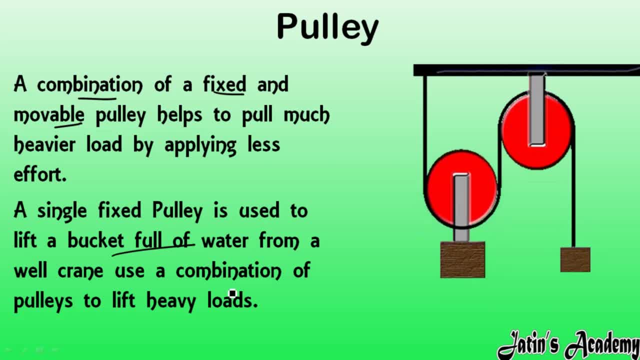 going to apply a force in the upward direction. that bucket can come easily from a well by using a single fixed pulley, okay, but in other hand, if we are using- if we are talking about the cranes- cranes are lifting very much heavy loads- okay, so in a crane we are using the combination of two. 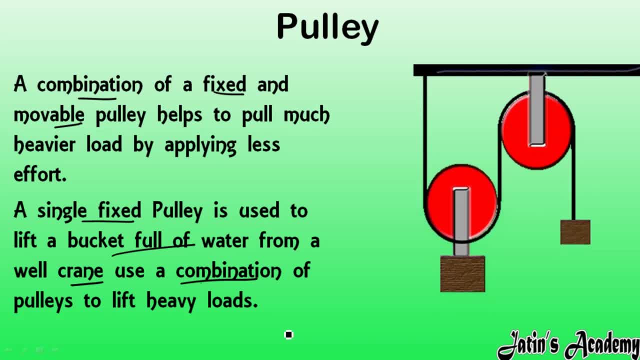 or more pulleys, or in a combination of fixed and movable pulley- fine. so in order to lift up very heavy load, we are using crane and in order to lift up small load, we are using a single movable pulley, single movable pulley or single fixed pulley: fine. next, we are having numericals related to pulley. 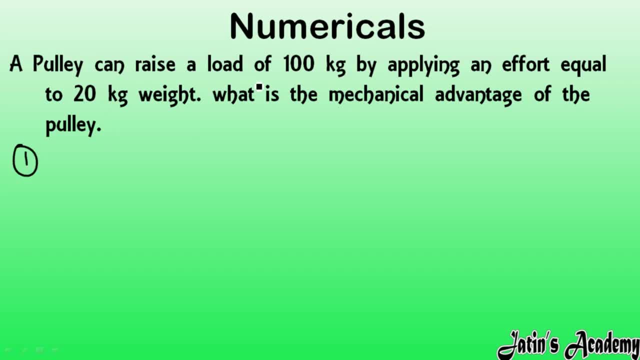 so see carefully the first numerical: a pulley can raise a load of 100 kg, so load is given. load value is given 100 kg by applying an effort equals to 20 kg, so effort is given 20 kg. what is the mechanical advantage? mechanical advantage, we have to calculate. i will tell you. 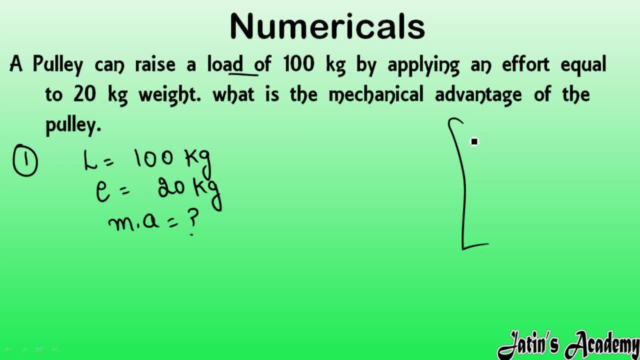 the formula again one time that what is the formula for the mechanical advantage? mechanical advantage formula is load over effort or one formula also. we are having effort arm over load arm. okay, if in any numerical we are having effort arm or load arm, that in that numerical we will use. 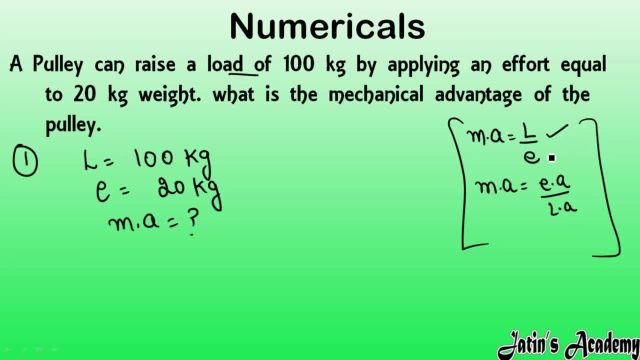 this formula, otherwise, if we are having load and effort, we will use first formula. fine, so see the formula carefully. we are having mechanical advantage is equals to load over effort. so what is the value of load, load, load over effort. load is 100 kg over effort. is what 20 kg? so zero cut with zero, two ones are two, five, twos are ten. 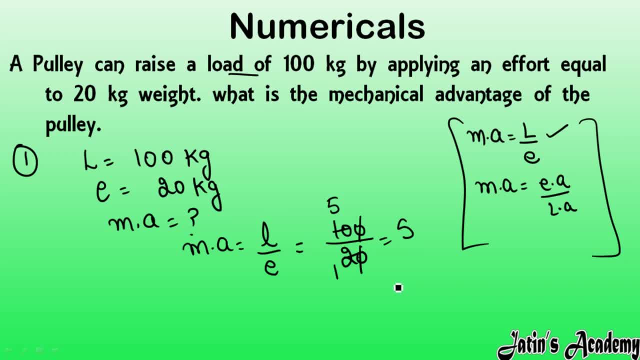 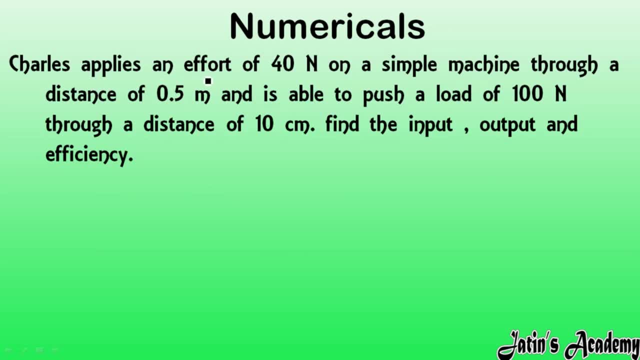 so mechanical advantage is five. what is the unit of mechanical advantage? no, mechanical advantage is having no unit. fine. next we are having charles apply an effort of 20 newton, so effort we are given with- sorry- 40 newton. charles apply an effort of 40 newton, so effort we are given with 40 newton. 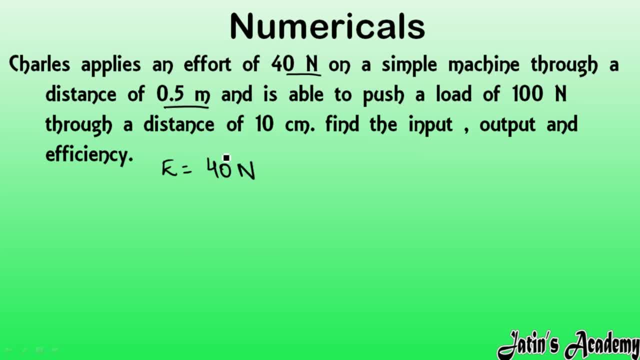 on a simple machine through a distance of zero point. five meter means on a simple machine whatsoever. this simple machine is there. he is applying effort of 40 newton, so this distance is given. this distance is nothing but a effort arm. effort arm is given 0.5 meter and is able to push a load of 100 newton. so he is able to push a load of 100 newton. 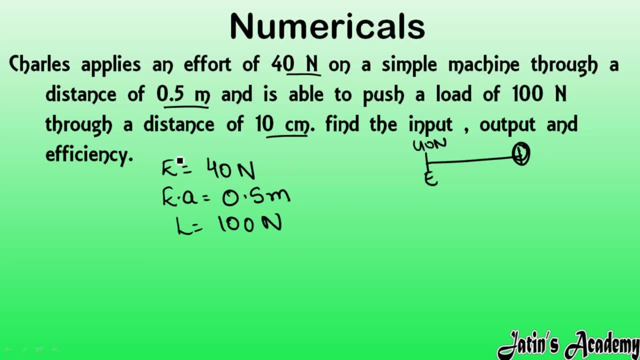 through a distance of 10 centimeter. so load and distance is given means load arm is given that is 10 centimeter. firstly, convert this 10 centimeter to a load arm and then we are able to push a load of 10 centimeter into meter. why? because upside you can see carefully that effort is in newton effort arm. 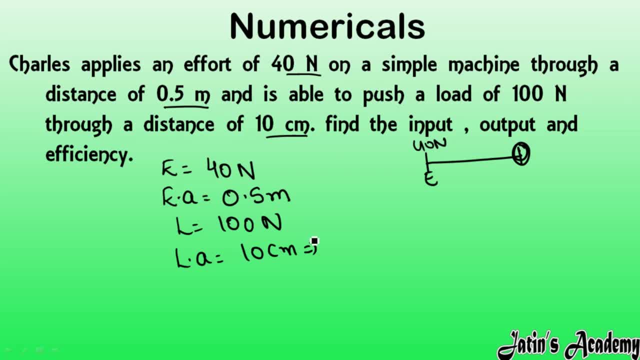 is in meter, so here also it should be same. that is, load in newton and load arm in a meter. so convert into a meter, as we know, in one centimeter. 1 by 100 meters, are there fine? so 10 by 100 meter, that is. 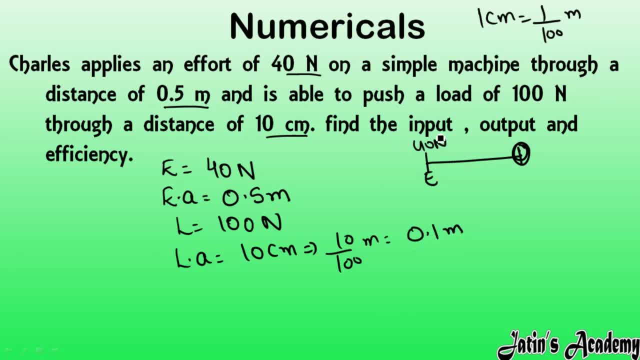 0.1 meter. so we have to calculate input, output and efficiency of a charles. okay, so what do you mean by input? actually, what do you have, knowing that formula that effort into effort arm is equals to load into load arm, principle of lever? actually, in this case, effort into effort arm is nothing but input and load. 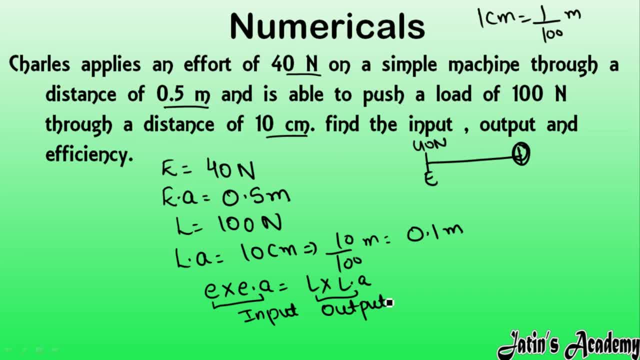 into load arm is nothing but output. so from here you can see the formula: input is equals to effort into effort arm. this is a formula of input. so just put the values of effort and effort arm, so input will be: effort is what effort is 40 multiply effort arm is what that's. 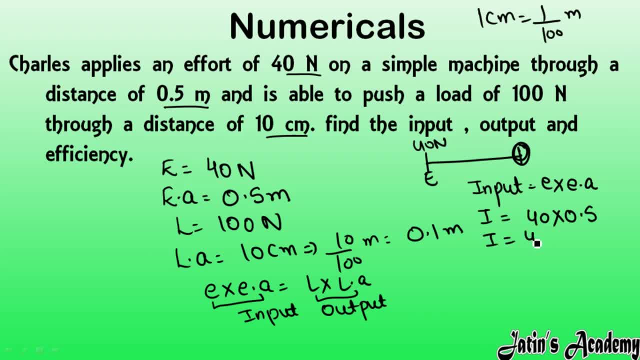 is 0.5. solve it, you will get. input is equals to 40. multiply 5 by 10, 0, cut with 0, you will get 20 joule. fine, and here we are going to calculate the output. output formula is what output is load. 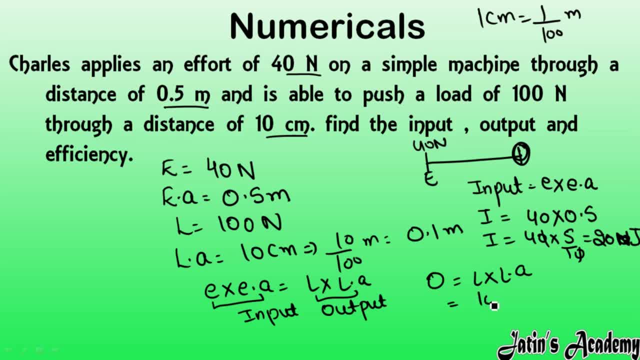 into load arm, so load is given. we are with 100 multiply, load arm is given 0.1. so solve it: 100 multiply 1 by 10, that is 10 joule. so output is 10 joule. input: we have found. output we have found. 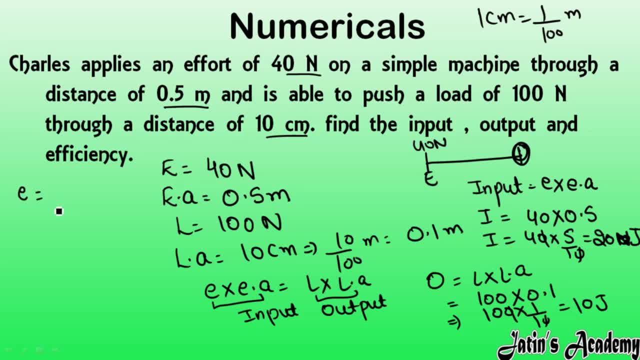 now the work is efficiency. so what is the formula of efficiency? efficiency means output over input. so what is the value of output? that is 10. what is the value of input? that is 20. so efficiency is 0. cut with 0, that is 0.5. or in efficiency percentage you can write 0.5 multiply 100, that is. 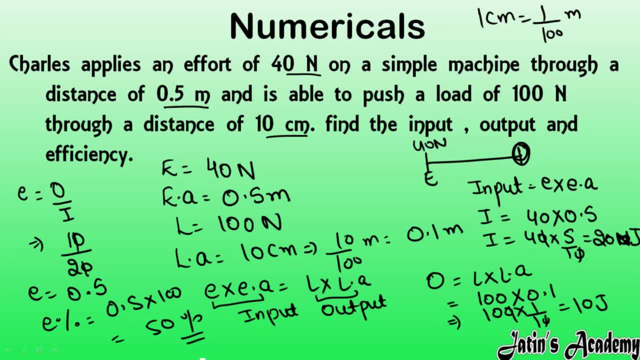 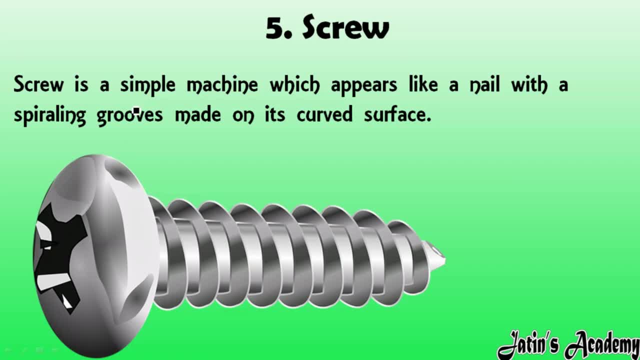 50 percent is the efficiency fine. next type of simple machine we are going to study, that is a screw. so screw is also a simple machine. which appears like a nail means in a screw. it appears like a nail but it is having a spiraling groove made on a curved surface. in this curved surface. 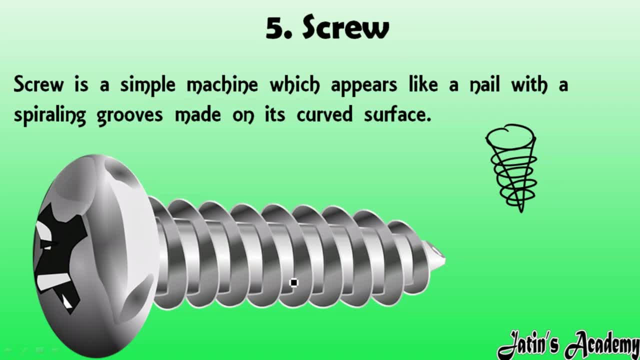 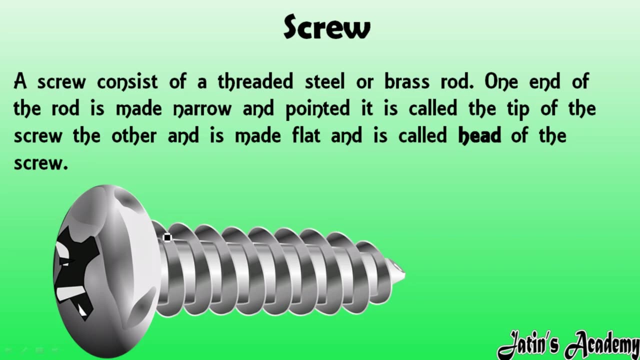 spiraling grooves are there might be this you are watching here. these grooves are there. okay, and whenever on a nail, grooves are there, that is known as, or spiraling, spiraling grooves are there. that is known as screw. okay, so a screw consists of a threaded steel. actually, in this screw, threaded steel, is there one end of the? 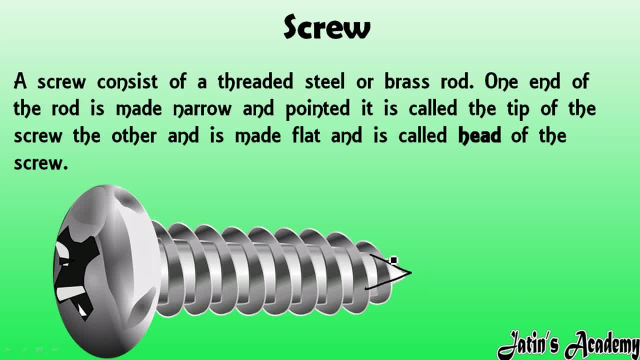 rod is made narrow. one end of the rod of this screw is made narrow and pointed and this edges and this and this narrow and pointed is called tip of the screw. this is known as tip of the screw, the end of the screw which is made narrow and pointed. 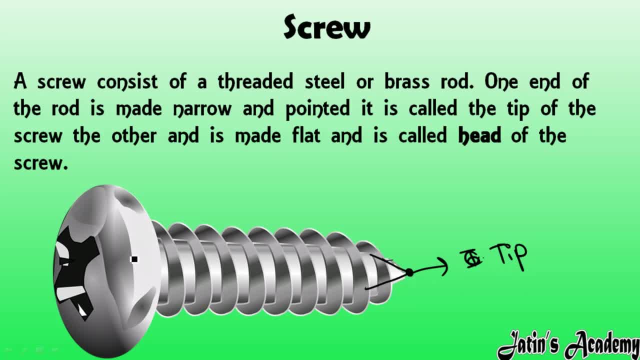 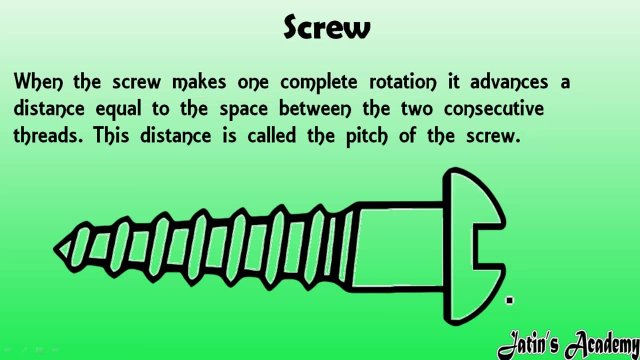 that is known as tip of the screw, and the other end, which is made flat. that end is known as head of the screw. head and tip is clear to you. the broad area of the screw is known as head and the narrow and pointed area of the screw is known as tip. next we are having when a screw makes one. 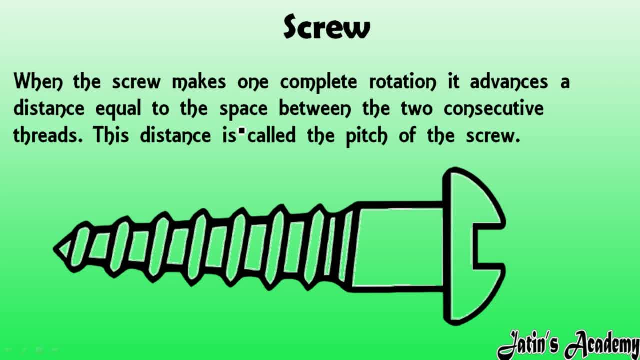 complete rotation, it advances a distance equal to space between two consecutive threads. means whenever the screw is going to complete one rotation means whenever we are going to push the screw into a wall, whenever we are applying force from here, we are applying force from here. okay, in a rotational form, we are applying the force. so whenever this screw is going to complete. 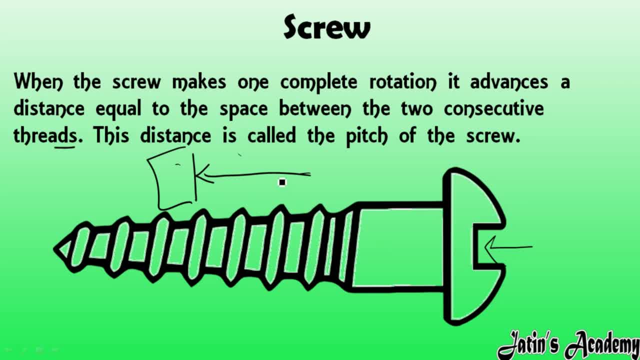 its one rotation. one rotation means what? that one rotation is equal to the distance between these two threads. actually, these are the threads whenever this screw is going to complete its one rotation, whenever we are applying force from the outside. that one rotation, then one complete rotation, is exactly equal to the 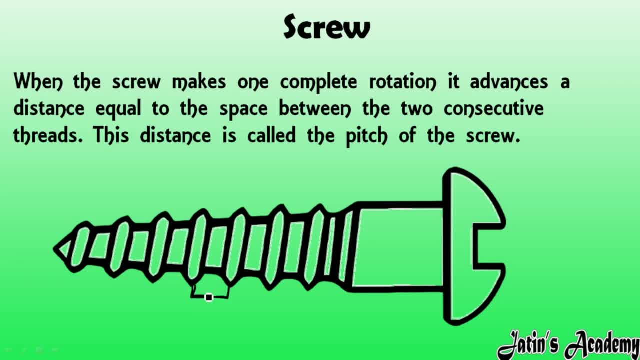 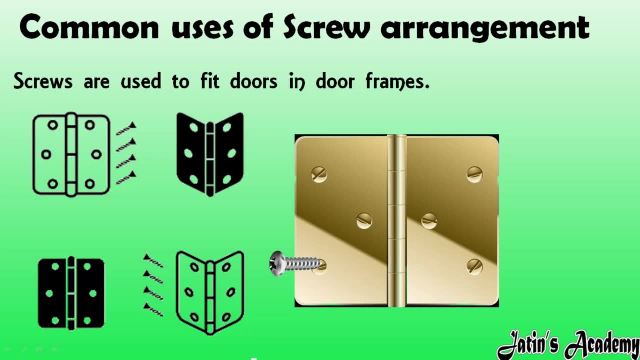 distance between, or the space between, the two consecutive thread, and this distance between the two consecutive thread is known as pitch of a screw. this is known as pitch of a screw. next, we are having common uses of screw arrangement. so screw arrangements are used to fit the doors in a door frame. whenever you want to fit the door into a door frame, you are using these. 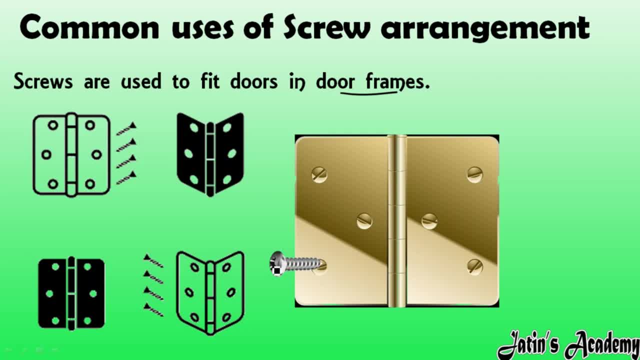 kind of screw might be. you have seen this: whenever hole is there, we are going to put the screw into it from the outside. we are applying the force. whenever we are applying the force, it is going to move inside, inside and finally it will look like this: okay, so screw arrangement is used to fit the doors. 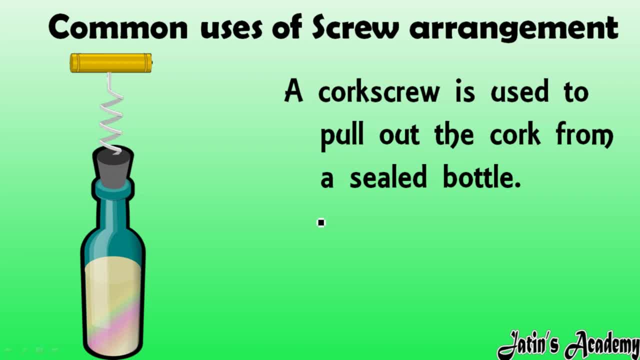 in a door frame. next, we are having common uses of screw arrangement. a cork screw is used to pull out the cork from a sealed bottle. actually, this is a form of cork screw. this cork screw is used to take the cork out from a sealed bottle means when you want to take the cork out from the seal or sealed. 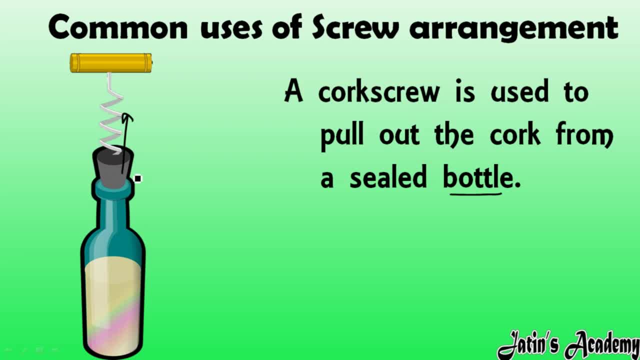 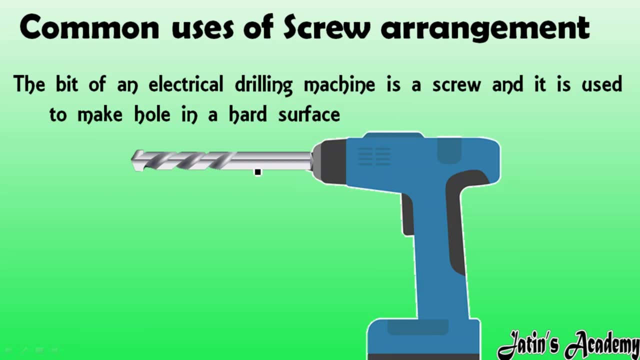 bottle. by applying our force, by our hand, it is not possible to take it out, so we are using this kind of screw, cork screw. so with this cork screw we can easily pull out the cork from the sealed bottle. and a bit of an electrical drilling machine is a screw here also in this k in a drilling. 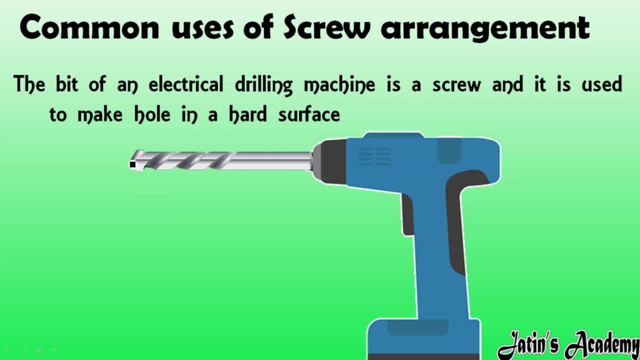 machine also, we are using a screw and it is used to make the hole in a hard surface by using a drill. in a drill screw arrangement is there whenever we are applying force from the outside. it is going to move inside and inside on into the wall or into the hard surface, so it will make a hole into a hard 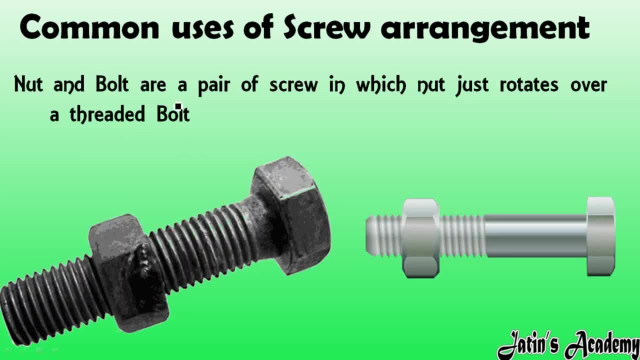 surface. next we are having nut and bolt. nut and bolt is also a pair of is also an example of pair of screw in which nut is just rotate over the threaded bolt. this is a bolt, this is a bolt full fledge. this is a bolt and this is a nut. whenever you want to move the nut inside the bolt, then also. 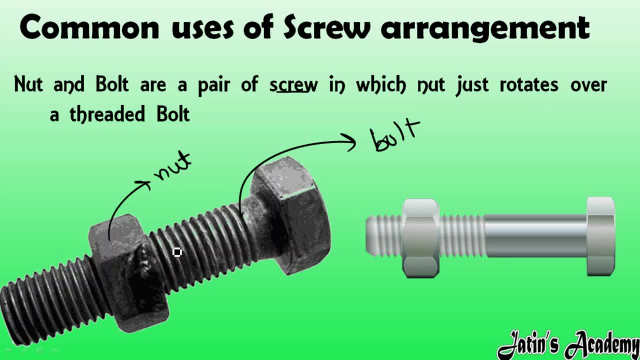 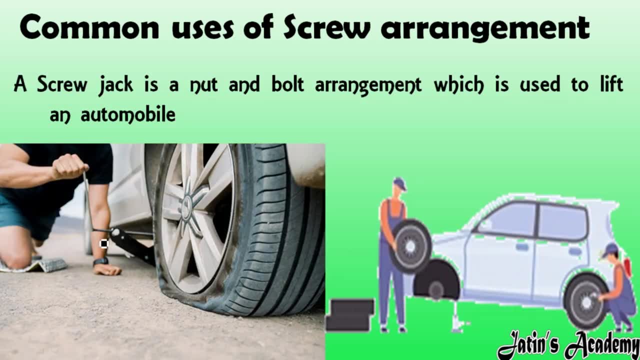 we are applying the force and that nut is going to rotate over the thread, that bolt. okay, then we are having a screw jack. so screw jack, this one which is used to lift up the heavy materials or heavy cars, vehicles. okay, this screw jack is also a nut and bolt arrangement in. 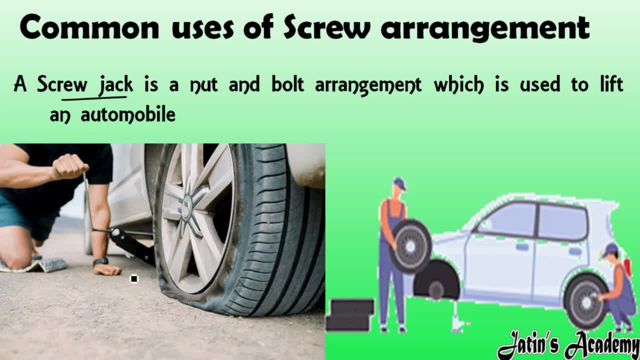 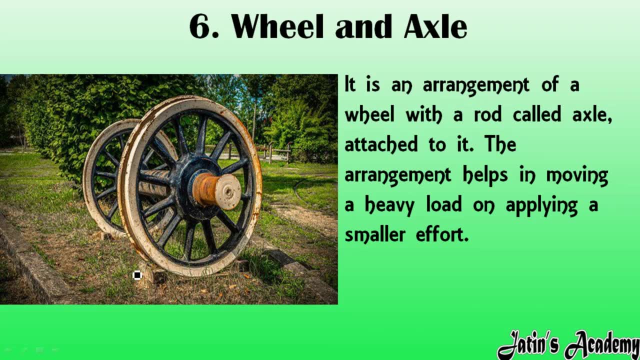 the screw jack. also, we are having nut and bolt arrangement in which nut is attached on the like threaded bolt. fine, then arrangement of simple machine. next six: we are going to study that is the arrangement of wheel actually here in wheel and axle. first we are having wheel. this wheel is: 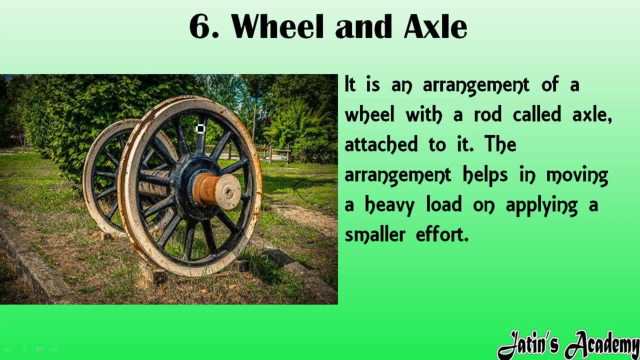 attached to one fixed sport that is known as axle. this is a wheel and this fixed sport in in between might be you are watching that is a axle. okay, the arrangement. help in moving a heavy load. might be you are knowing, in a cars also, or on a heavy loads also, these wheel, we are using these kind of wheel. 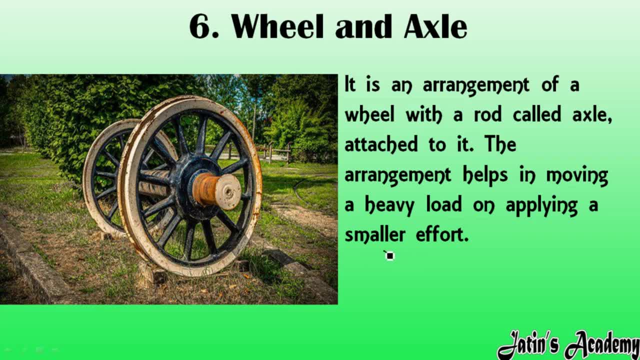 we are using in order to move anything. so by applying even though less effort on a heavy load, we can easily move a heavy load with the help of wheel and axle. in a car also, in automobile also, we are using wheel and axle arrangement. so here this, we are having a wheel. 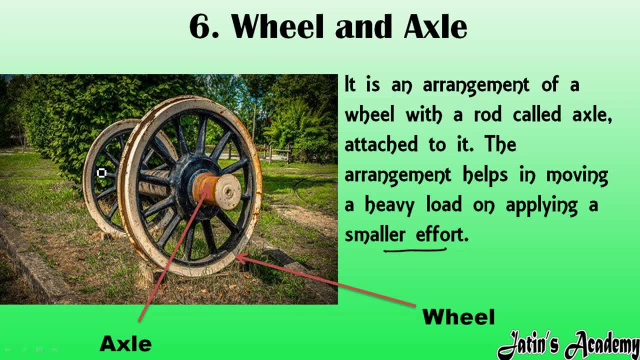 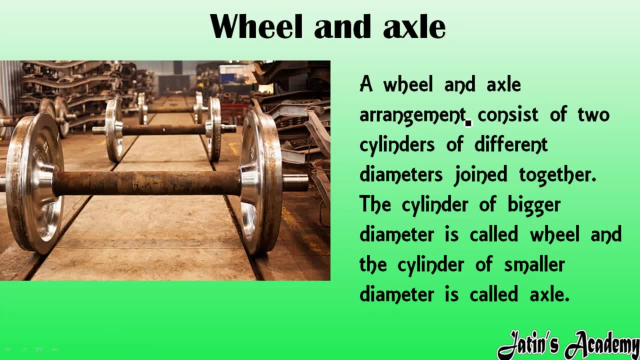 this circular part. we are having a wheel and this fixed point about which wheel is going to rotate. that fixed point is known as axle. next we are having a wheel, and axle arrangement consist of two cylinders of different diameter. how to slender? see carefully. first we are having this one. 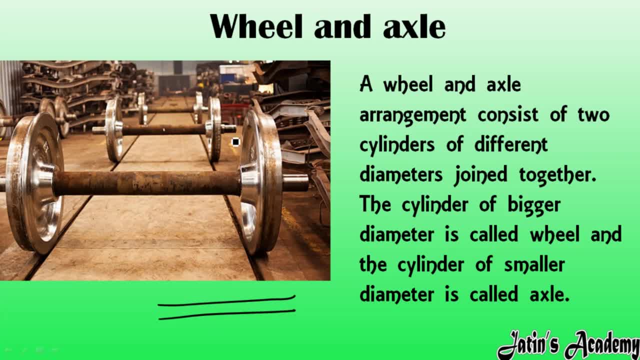 in between two wheels, one cylinder we are having, and here also this circular path is a cylindrical form. actually cylinder is in this form, like this. this is a form of cylinder, so this is a cylinder. this is also cylinder means in a wheel and axle arrangement. we are having two cylinders, but with 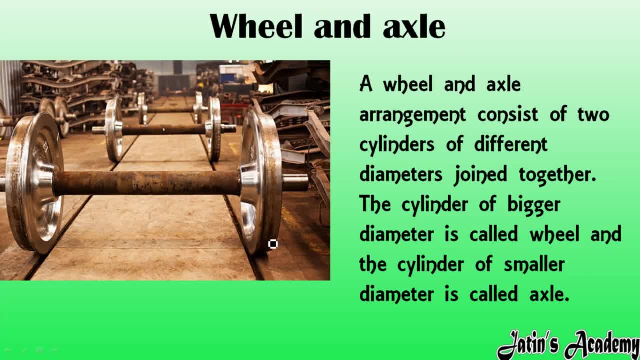 a different diameters, as you can see carefully, see clearly that in this wheel larger diameter is there and in this cylinder, in this slender we are having larger diameter and in this slender we are having smaller diameter and the slender of bigger diameter is known as wheel. this slender of 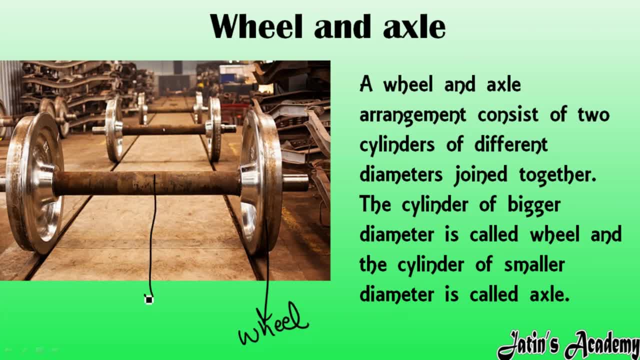 bigger diameter is known as wheel and the slender of smaller diameter is known as axle. if definition of wheel and axle will come in exam, then you have to write like this, okay. next we are having examples related to wheel and axle. so first example related to wheel and axle we are having 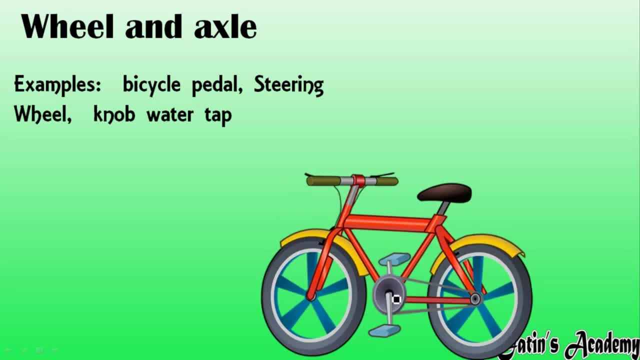 bicycle pedal. so in a case of bicycle paddle, actually what we are doing here? here we are having two circularnectar wheels. these paddles here in a, in the paddles, are two circular wheels are there and in between, two circular wheel. this axle is there means whenever we are rotating the paddle with one paddle. second, 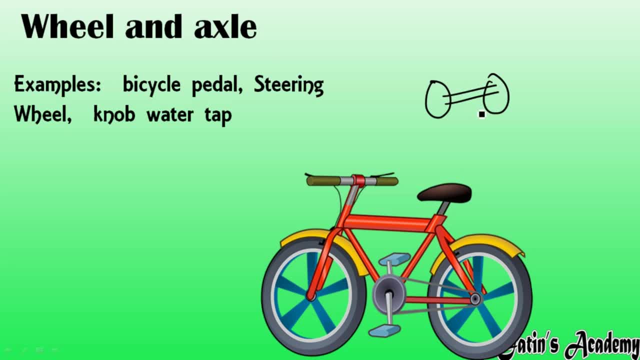 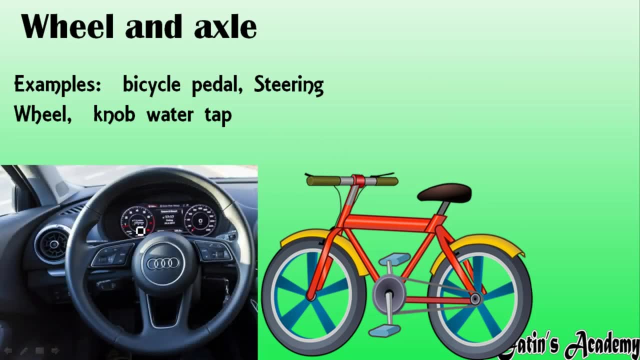 paddle is also rotating with the help of this axle, okay. second example related to this wheel and axle is steering wheel. in a case of car, this steering wheel is attached to the tire of the car with the help of one axle. okay, this is steering wheel is also a wheel, and tire of a car is also. 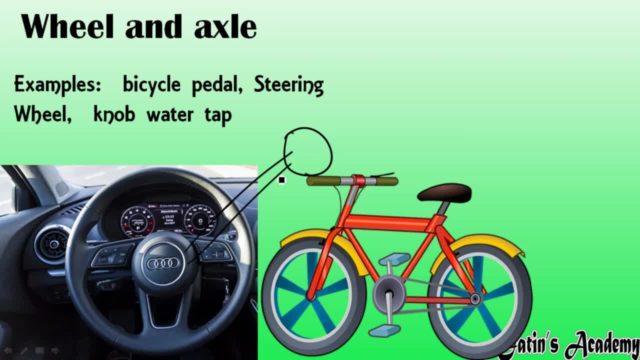 a wheel and in between we are having axle. so this is a wheel and axle arrangement. so what is happening here? actually? in this case, whenever we are rotating the steering of the car, by rotating the steering of car, this axle is also rotating. with this wheel, this axle is also rotating. and whenever this axle 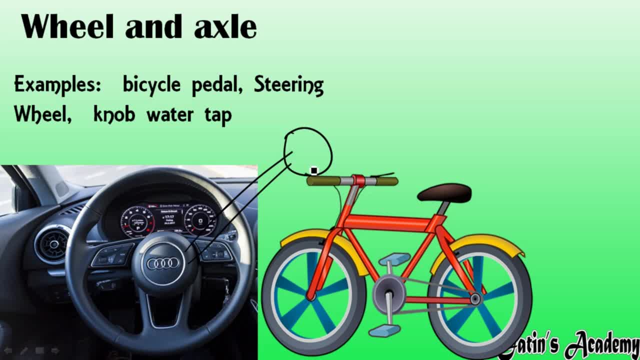 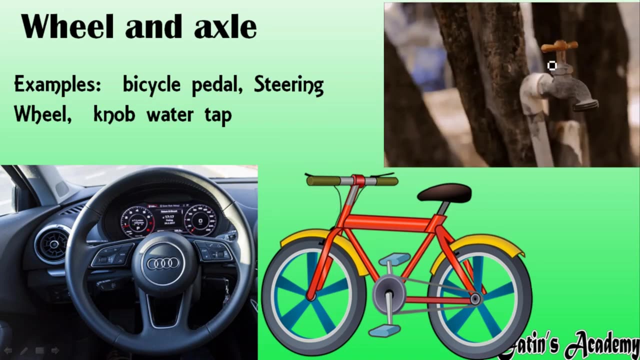 is rotating. it is also rotating the tire of the car means by applying the force on the steering we can easily change the direction or we can easily change the movement of the tire. next, we are having knob of water tap. in a knob of water tap also, we are having wheel and axle arrangement here also. 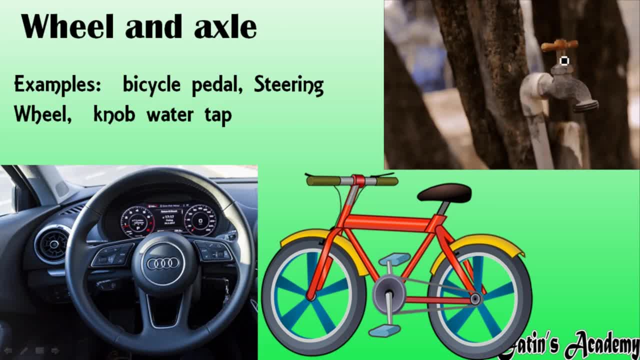 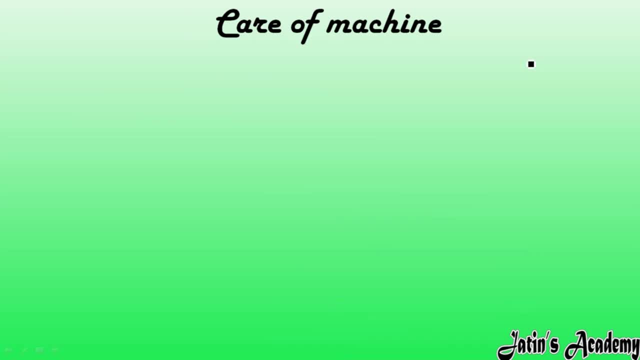 whenever we are rotating it. actually, this is a circular and here we are having axle. okay, wheel and axle is there, which can easily rotate a tap. next, we are having care of machine means. now we have studied about the six kinds of machine- simple machine- which we are using in our daily life. 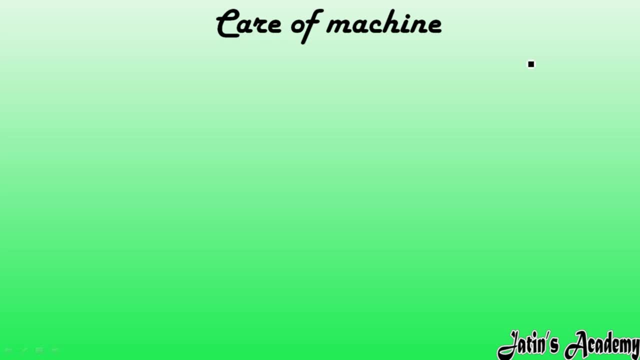 and we are going to talk about the six kinds of machine which we are using in our daily life. as we know, machines are making our work easier and faster means, with applying even the less effort, we can use it very comfortably. we can lift up heavy loads. we can use it very properly, okay. 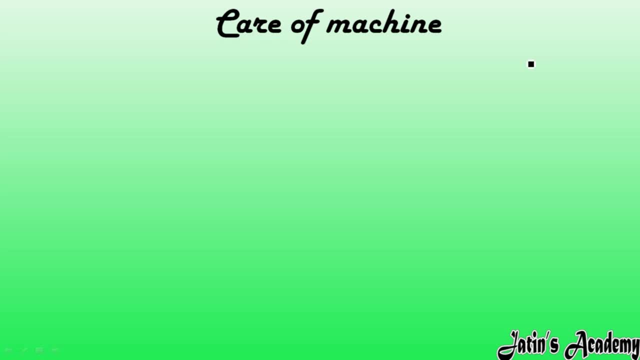 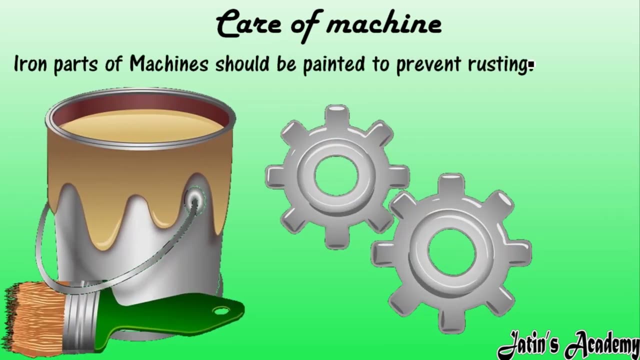 but in order to use this machine we should care these machines also. so here we are going to discuss some of the points: how to take care of your machines. so first, we are having iron parts of machine should be painted to prevent from rusting whatsoever machines we are having in that. machine. if any iron parts are pink, then you are having very, very strong machines, which we are using because we are using sand to predict the wear or the wear and tear of the machine. working order of the mixture equ, fordi here we have too much noise or dust, or if there is only a littleasit, so we have to accompany them as they can see. 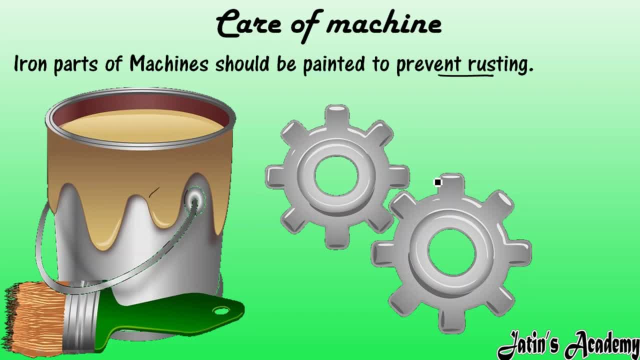 any parts on the machine, we will have a combination on that. any iron part is there, that iron part should be painted frequently so that iron should be prevented from rusting. so what do you mean by rusting? rusting means whenever iron, whenever iron is coming in contact with the oxygen or moisture or water, it will form iron oxide layer. 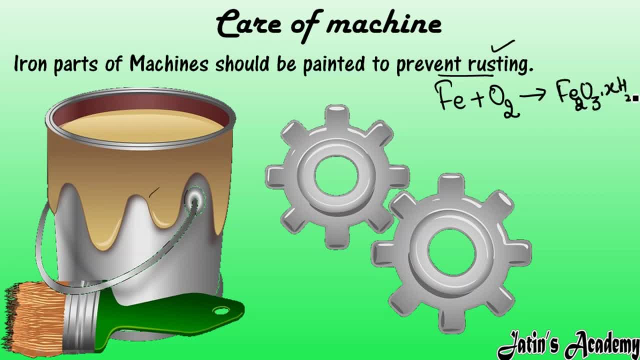 fp2o3, dot x, molecules of water, which is a rust. okay, so whenever iron is coming in contact with moisture, it will form the iron oxide, or we can say rust. it is going to form and this rust will slowly eat up the metal surface. so in order to prevent from the rust, we are using the paint in. 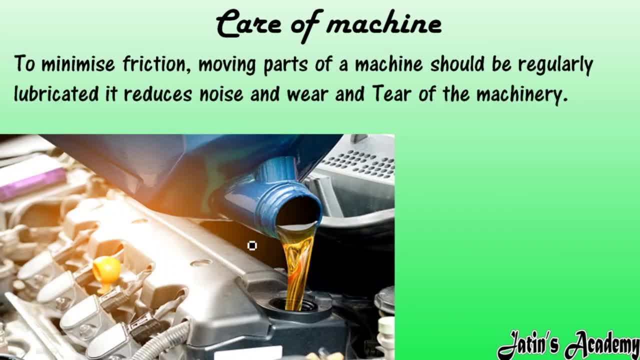 order to reduce it. next, we are having in order to minimize the friction, in order to minimize the friction in the moving part of vehicles, we are giving them to the. we are giving the oil or lubrication lubricant we are giving to the moving parts of the machine so it can reduce the. 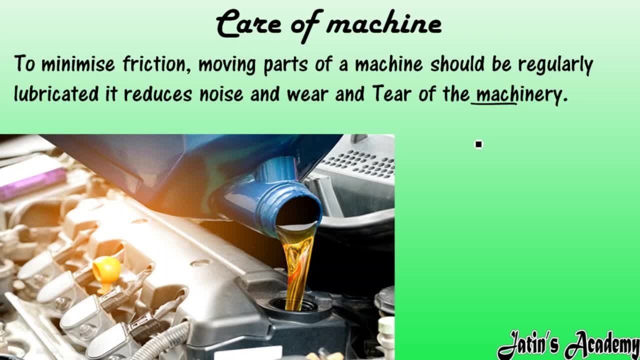 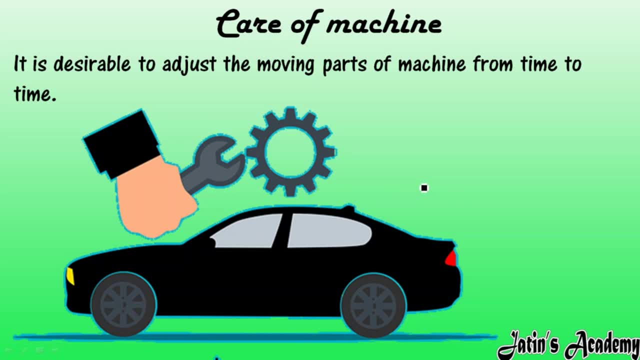 noise and wear and tear in the machinery parts. next we are having. it is desirable to adjust the moving parts of machine from time to time. if you will see that, yes, now my bicycle or now my car is not working properly, then you should take that bicycle or automobile to the like a care center. 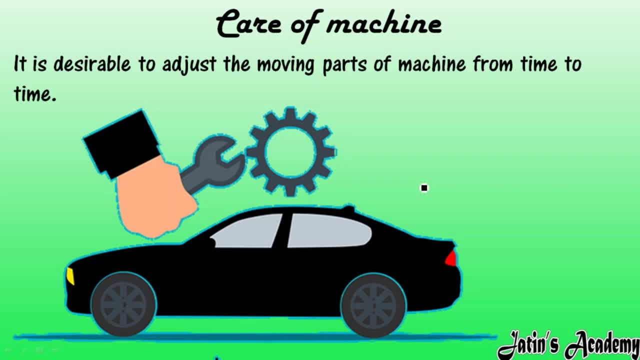 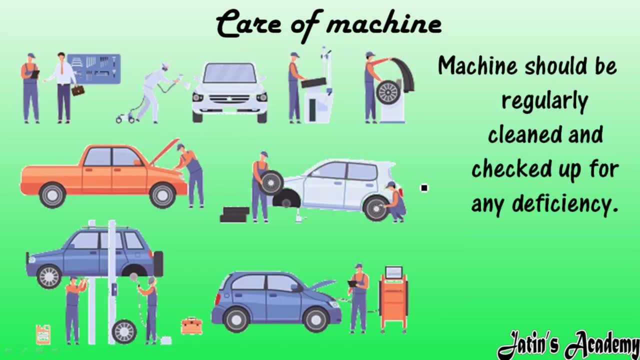 so that they can properly make it. they can adjust the moving part by using some formulas and all okay. so it is desirable to adjust the moving parts from time to time. next, we are having machine. should be regularly cleaned means if you having a bicycle or you having any simple kind machine in. 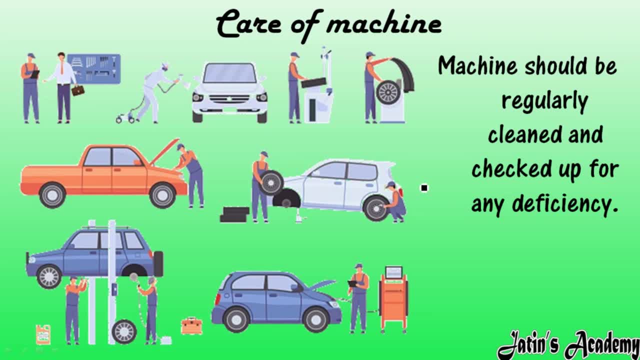 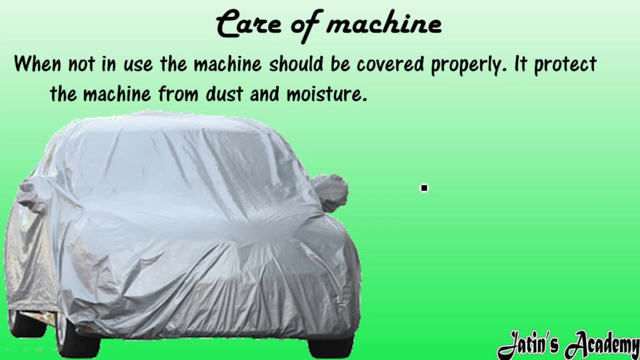 your house. that machine should be cleaned after regular intervals of time. even though, for example, you are having an automobile that should be go in a service center, that person can service it properly and it should be maintained properly whenever not in a use. whenever our machinery parts are not in use- for example, our car is not- we are not moving, we are not using it many, much.